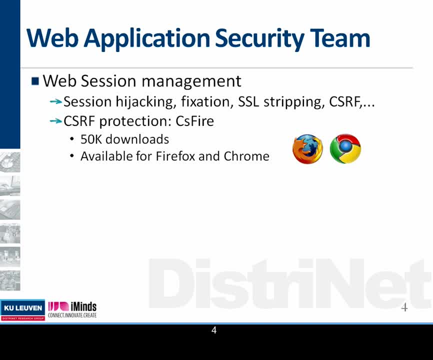 fixation, SL stripping, cross-hatch, request forgery and the like. We have the knowledge on the server side, but we also tried out what we can adapt on the client side, how we can actually secure the client side when we are visiting web servers that are not protected. 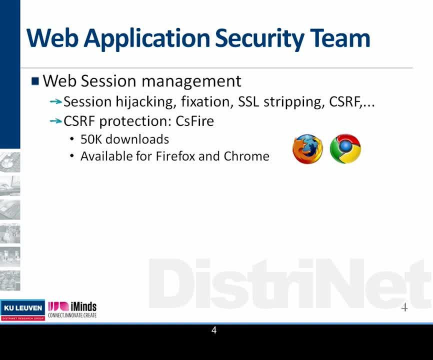 against these type of attacks, And the most popular one is Ceasefire. It's available for Firefox and Chrome and has over 50,000 downloads per day. It's already in the extension store. We're also working on mashup security, And what I mean with mashup security is actually 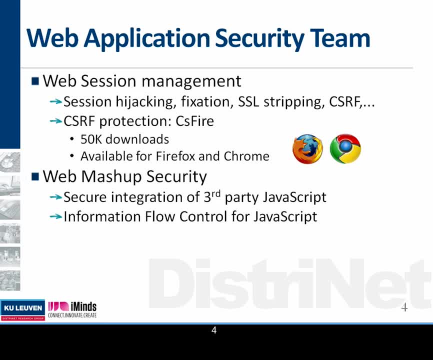 how we actually treat JavaScript in our websites. If JavaScript from multiple sources is coming together in a website, how can we make sure that one JavaScript does not impact the security of your website or does not affect the execution of other scripts on your page? It used to be mainly in dedicated websites, mashup websites with gadgets and so on, but 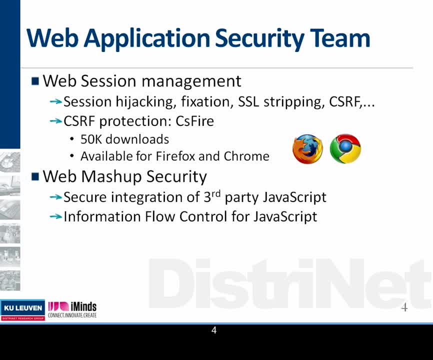 to be honest, any website you're visiting nowadays has content coming from multiple sources, and Nick will go into much more detail in this afternoon's session. We're also working on information flow control for JavaScript, which is an orthogonal topic on purely sandboxing. 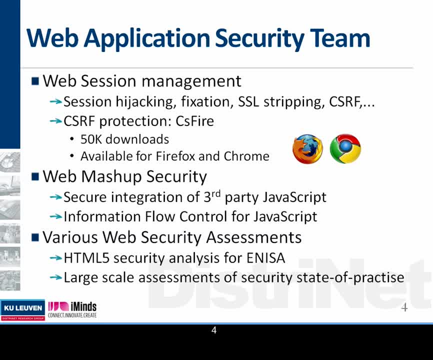 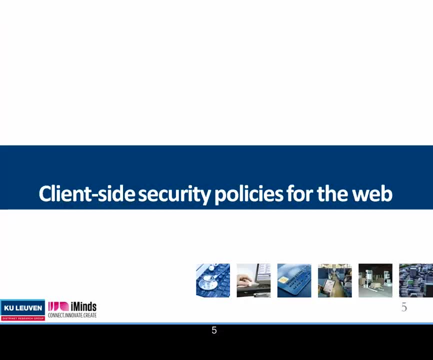 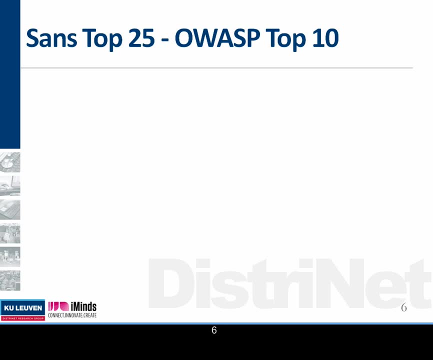 We did various web security assessments. We did the HTML5 security analysis for Anissa, but we're also doing a lot of experiments to see what is the state of practice on the web nowadays. But for today, the client side security policies. When we look into web security, we have, for instance, the sound stop 25, we have the 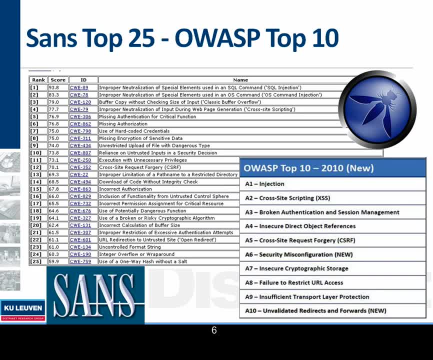 OWASP stop 10, all different vulnerabilities that occur quite often in web applications and a whole set of mitigation techniques from the server side. What are the security coding guidelines to protect against cross-site scripting, against SQL injection, against cross-site request forgery? 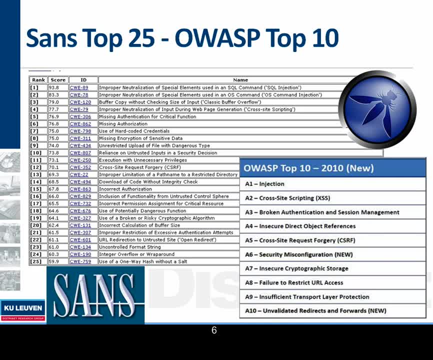 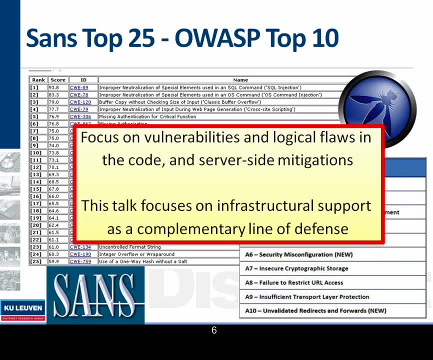 We already saw quite some of those vulnerabilities and countermeasures in other talks, like the talks of Jim. In this talk I will not focus on how to adapt the server code. In this talk I really want to focus on how we can actually add or: 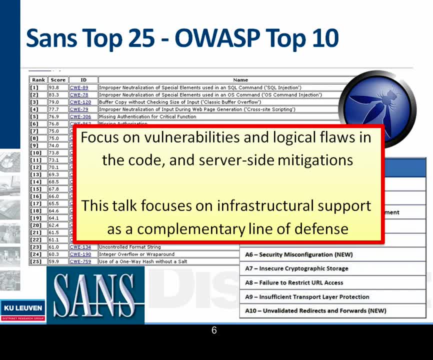 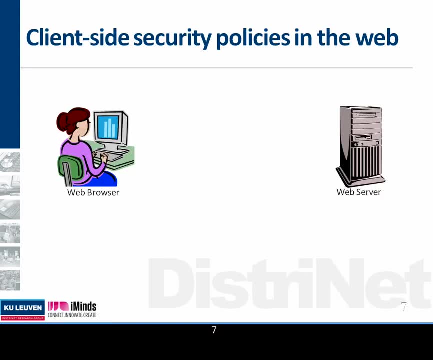 use the infrastructure support as additional line of defense in protecting your web application. So you still. the server wants to protect this website from the server side out, but it will not adapt the code of the website application itself, but send additional information to the browser to secure the application. 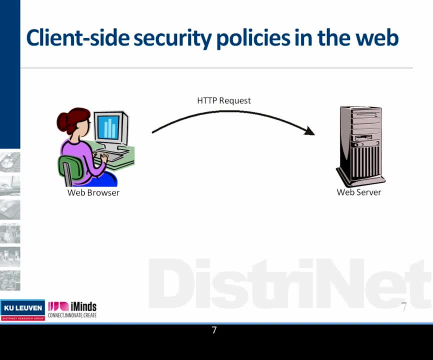 So if I try to visually demonstrate this, so we typically have the HTTP traffic going on between the web browser And the web server. in the talk, in the items I will discuss today, we will have actually security policies residing on the server side, So the website owner decides what is the appropriate. 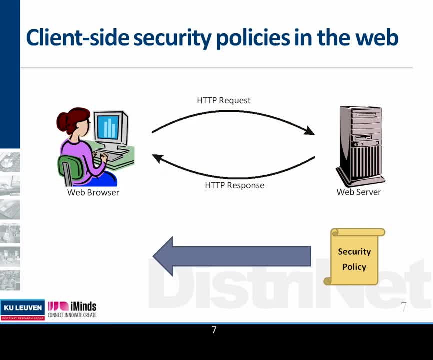 security policy for its own application and pushes that security policy to the client and that is enforced in the browser. What's important is this whole setup. This policy enforcement gets standardized and is actually almost all the things I will discuss today are by default enabled. 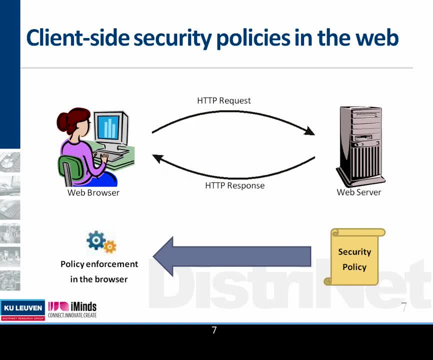 So we can really use this kind of technology to enforce your policies. So the policy enforcement in the browser does not rely on No. So it's really part of, for instance, the HTML5 standard, the way browsers are actually adapting new standards like secure transport, security and all the things They're really. 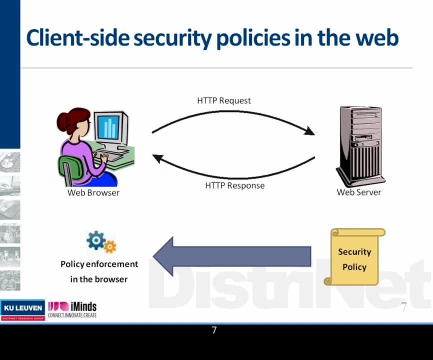 adapting themselves to be more secure than originally planned, You will see, for some of the techniques that were extended in the past. So you can actually enable that. But it's not that you need things like no script and configure them. They are by default embedded in Chrome, Firefox and so on. So this is. 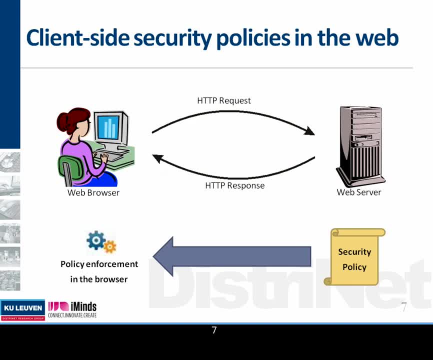 actually the main focus of the talk. Important to say: You say policy enforcement in the browser. Does it also mean that there is also a default policy? Because now you said the security policy comes from the web server, Depending on the technology. For some there's a default policy already in the browser. that 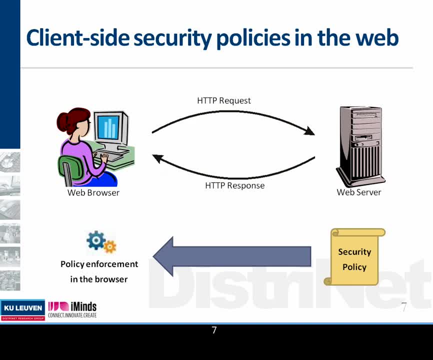 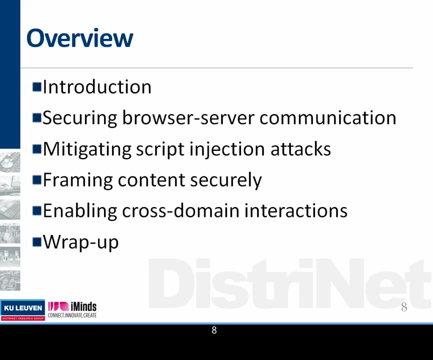 you can override. For some it's very reluctant because they want backwards compatibility. They don't enforce anything unless the server says that it needs to be enforced. Okay, This is the general picture of what I want to do today. I first will give a little. 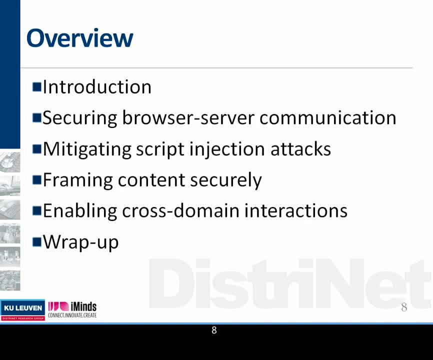 bit of introduction just to make sure that we're all on the same page about the standard security policy in web applications, And then I will discuss four topics where we actually will see that the state of practice actually evolves quite quickly. We've seen this quite a lot in the past two, three years. to actually make this server-driven. 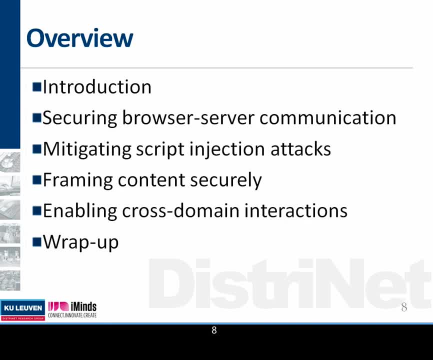 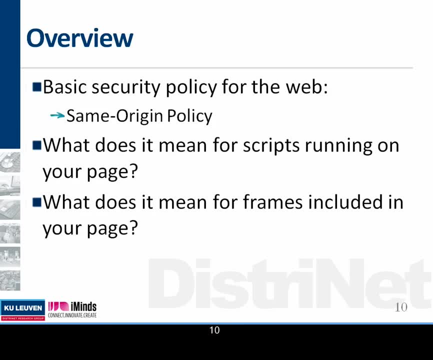 security configuration actually possible. So we saw already quite some talks on web security. So the basic technology of how HTTP, HTTP cookies and all the rest is working. I will not repeat this in this talk. I don't think we need to focus on that. One topic I wanted to pick out is the working of the 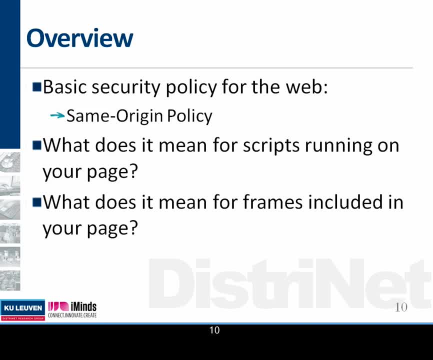 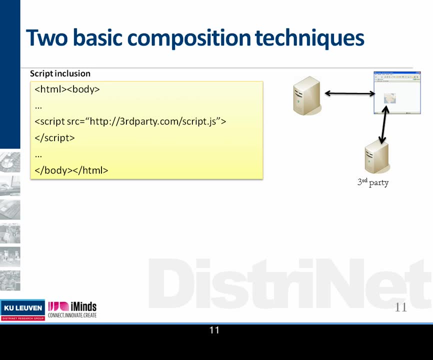 same origin policy because the basic security policy for the web already since the 90s is the same origin policy. Okay, And we need to understand what is the impact of the same origin policy on scripts and frames, to understand how certain techniques are taking advantage of that. 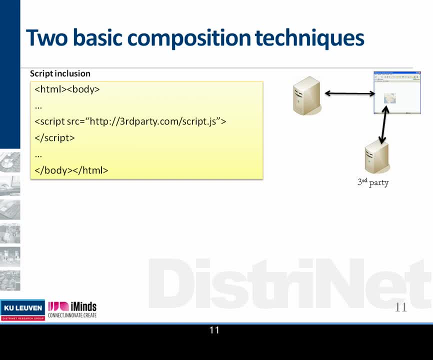 We have two basic composition technologies if you want to include content from a third party or from an interested source, even within your own domain. The first one is script inclusion. It means that you actually can load scripts from third parties as if you have written them yourself, And what it means from a security point of view is you're actually loading. 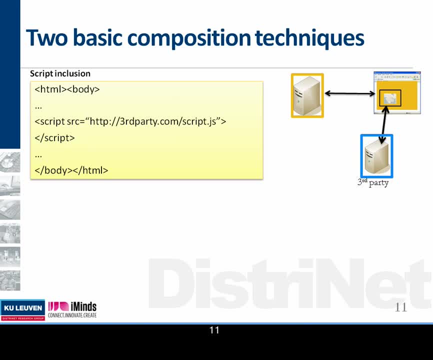 the resource from the third party in your application. But for the web browser it doesn't differentiate between external scripts and your own scripts. It's just running as if you wrote the JavaScript yourself. It's running in your security context. It has full access. 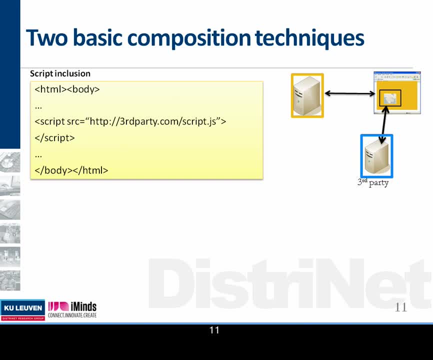 to the DOM, to cookies, to local storage. It can do anything your own application can do as well. So there's no security enforcement, There's no security boundary. You're just taking third party resource and running and executing it as if it was your own resource. 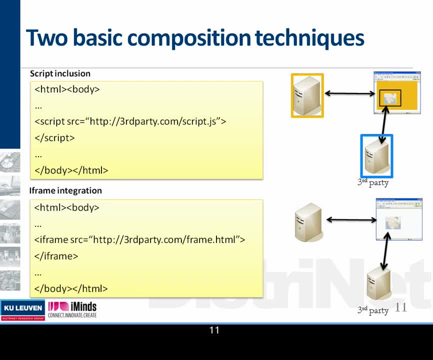 The other technique to include third party content is iframe integration, And it means that you actually will put a separate almost window as part of your original website, an additional frame, And that frame loads content from a third party. This has a whole different technology in looking towards security enforcement, because the original page, the outer page, 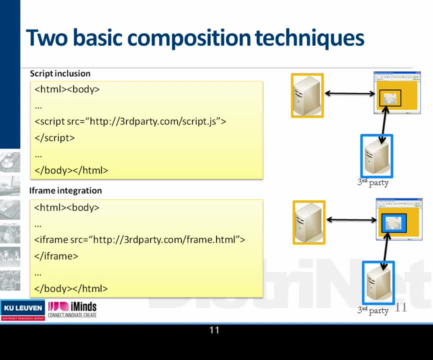 will run in the security context of your own website, But the third party content will run in its own security context of that third party domain. So we have a strict security sandbox between the two. You have a strict security separation. The third party content can still do all sensitive operations at once, but they will execute. 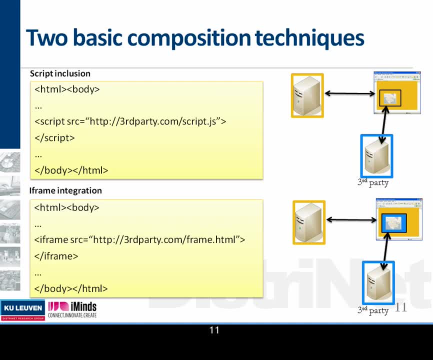 in the domain of the third party. So it can only look to the cookies of the third party. It can do storage in the third party. It can contact back to the server of that third party domain. If you're looking to what is used on the web, I would, Two years ago I would say 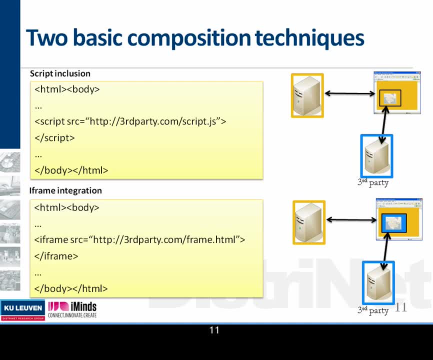 almost anyone is using script inclusion, So all the things that you include from third party reside to be script inclusion. We see a trend, for instance in Facebook, but also in other integration networks, that they are actually using the sandbox attribute to make. 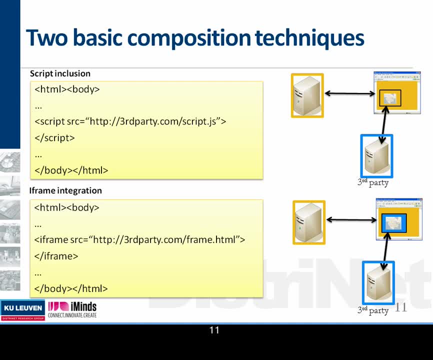 sure that there's, by default, separation between content of a third party and their own content, and that they're using interaction mechanisms like web messaging to interact between the yellow context And the blue context. So we see a shift from this towards this, but this is only a minority. Nick will go. 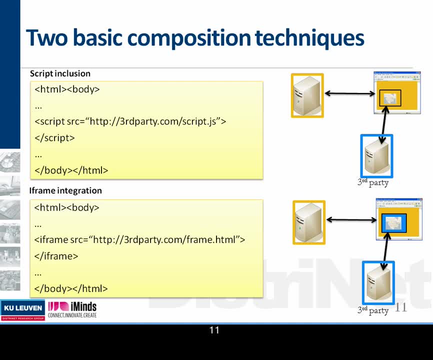 much further in discussing this. but script inclusions: we can easily say that almost 90, 95% of all the websites are including scripts from a third party. Okay, This is enough for basic context. We know the security policy. the same origin. 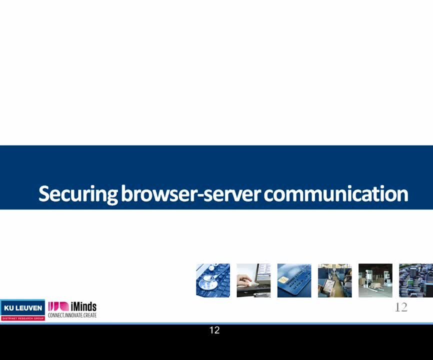 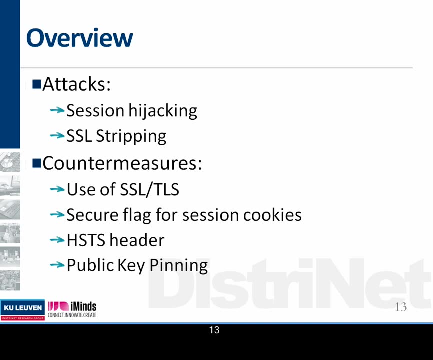 policy, and that will be enough to understand all the rest of the talk. The first topic we want to actually touch is how we can secure the browser-server communication And the two attacks I will discuss here all: session hijacking and SSL stripping- and I will discuss 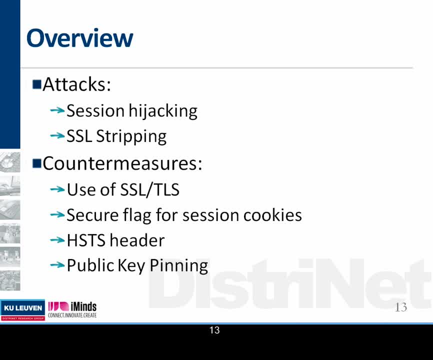 a number of countermeasures in increasing complexity or in increasing protection that they will offer towards secure communication between the browser and the server. So the first attack, session hijacking, will not be new. We already touched on that in the talk of Germanico. The idea is that you have to have a security, a security-based 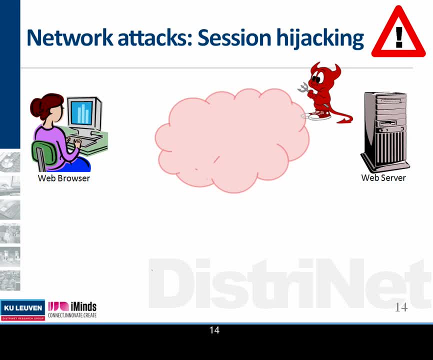 communication between the browser and the server. So the first attack, session hijacking, will not be new. We already touched on that in the talk of Germanico. The idea is that you have, between the web browser and the web server, some attacker that has control. 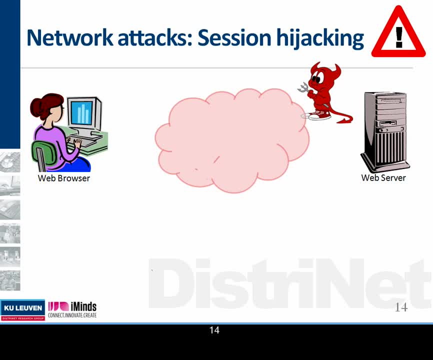 of the network and it can be a passive network attacker. Namely, it can just eavesdrop on the network. That's very easy to achieve. Any one is almost. you can easily eavesdrop what's going on and you can actually see any packets passing by without interrupting. 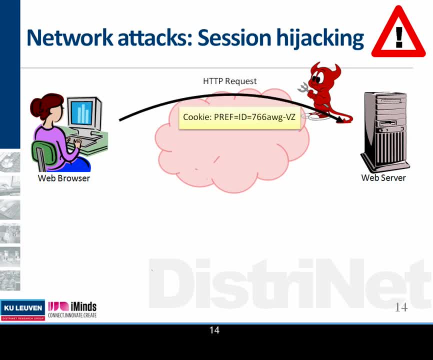 or without being visible. So what happens if you are using session management between the two? the web browser is sending an HTTP request to the web server. The library itself is a security, because this intelligence shows the security and the record. forestry is also concerned With the hackers. 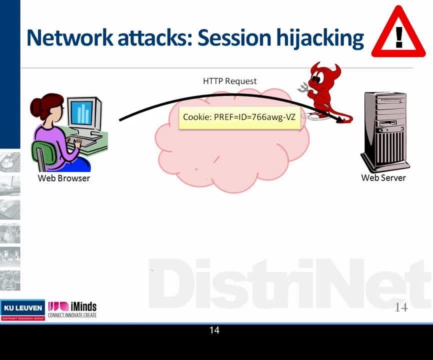 server attaching the cookie with the session ID. The eavesdropper, the attacker, sees that this cookie is passing by. It's actually setting up a new session to the web server reusing the same session identifier, And from that moment on, well, you can just take over the. 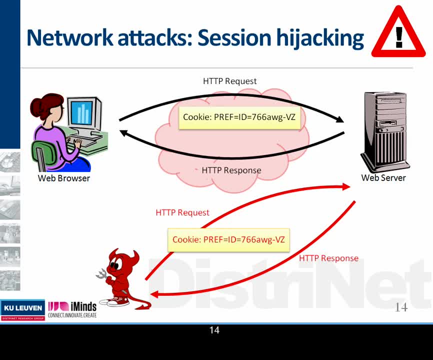 session and execute all the operations you want in a separate browsing environment. You don't need to control the browser of the client anymore. This is well-known to attackers, but still a lot of websites are verbal to this attack. Think about the FireSheep extension a few years ago. that. 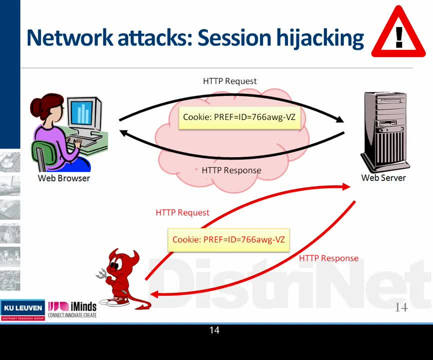 actually sniffed all the passwords of social networks, Gmail and the like. We see a trend that some of the larger websites are moving towards countermeasures, But still, if you would sniff during second death, I'm pretty sure that you would have a lot of passwords. 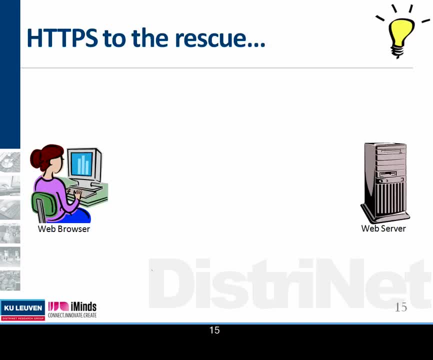 sniffed just purely by system hijacking. OK, We already saw a lot of talks Touching on HTTPS. it's an obvious choice If you want to protect your website against this. you're starting to put HTTPS on that, So you're actually tunneling or encrypting the channel. 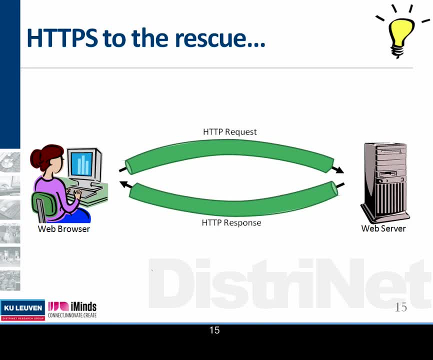 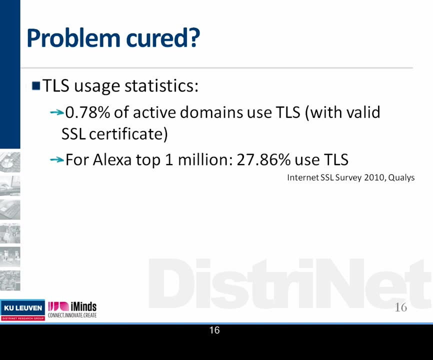 between the web browser and the web server, And by doing so, because you have confidentiality, the network attacker can't see your session identifiers anymore and you're protected. Quite obvious. But the question is: is the problem cured? Well, if you're looking to the survey made by Qualys in 2010,, 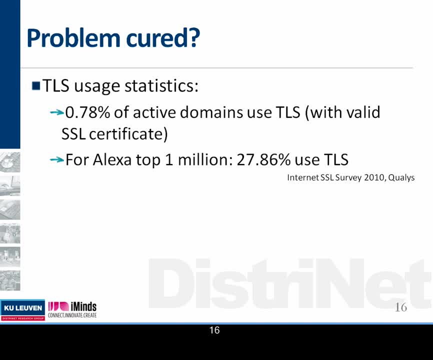 the use of SSL TLS is quite low. They actually monitored and they scanned all the domains on the internet to see whether they have HTTPS port open. They were also controlling if they had a valid SSL certificate and it turned out that only less than 1% of all. 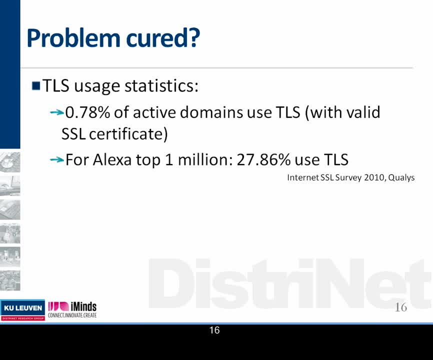 the active domains had TLS enabled with a valid certificate. We have to be honest: These are valid certificates. The numbers are a little bit higher with self-signed certificates, but we can't assess in the wild whether it was self-signed. certificates actually make sense or not. 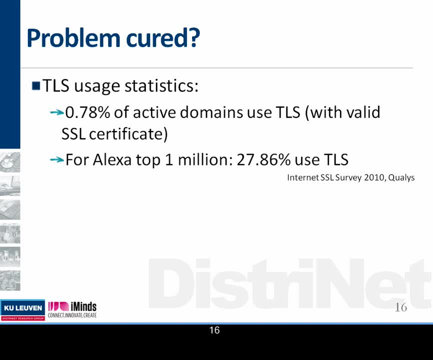 It could be, for instance, that organizations have their own CA actually signing the certificates so that people browsing externally can't assure that it's valid or not valid, but that for that company it's a good solution. Also, a lot of the devices that are scanned on the network. 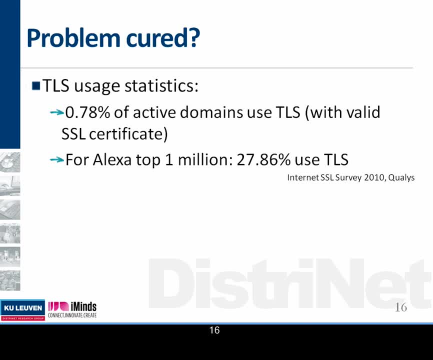 might not be a web server, might be your NAS connected to your home router or anything else- Anything that communicates HTTP was included in this survey If they were looking to the top 1 million domains recorded by Alexa, so the most popular domains which were visited by: 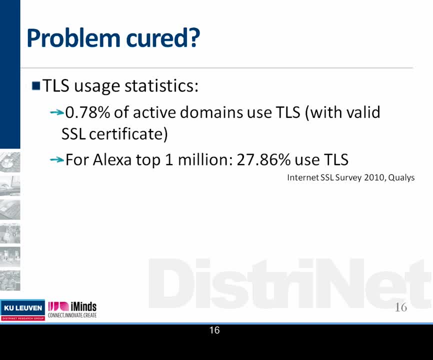 users having the Alexa toolbar in their browser. it turns out that around 27% were using TLS. The rate is much higher if you're looking to the most important websites or the most frequently used websites, But even if you're using TLS- I will show you in the next. 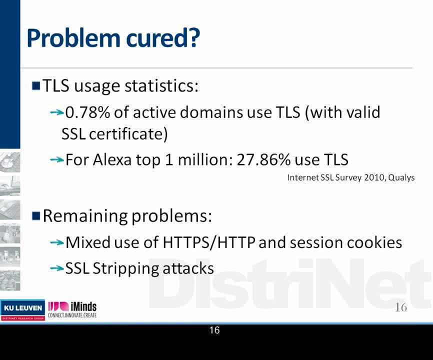 slides that there are still some remaining problems, namely in using HTTP and other services. I will show you how to use TLS and HTTPS in combination in hybrid setup and also with SSL stripping. So first, what is the mixed use of HTTPS and HTTP? 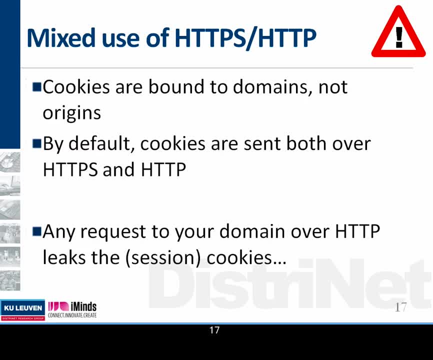 Well, you will notice a lot of websites you're visiting. you're starting with HTTP. you're going to HTTPS to actually enter your password. you're having a secure session on all the things that are changing session state or changing your profile, and it was already discussed in previous sessions. 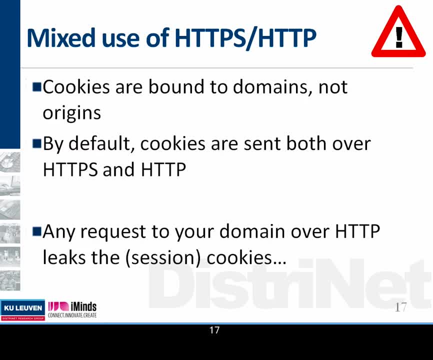 as well. So you have to make sure that you're protecting your session identifiers in a good way. By default, all those cookies that are set on HTTPS are also transported over HTTP. What's the impact of that? Any packet over HTTP, any request over HTTP, will leak. 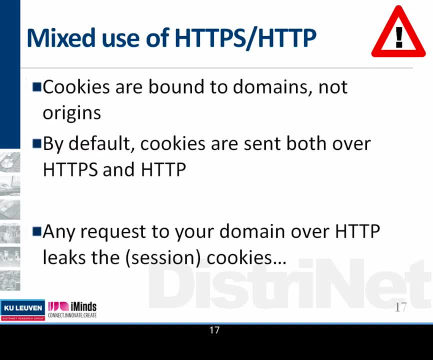 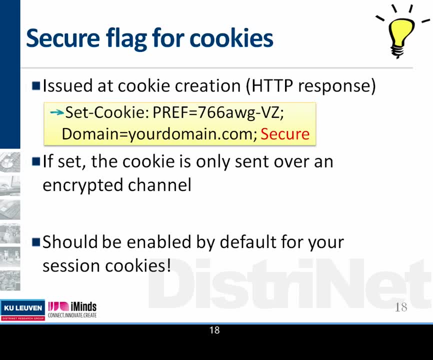 your session cookies or the whole set of cookies. So it means that you have to make sure that, if you're using a hybrid setup, that you secure them. And how can you secure them? Well, quite easily. there's a specific flag for cookies. 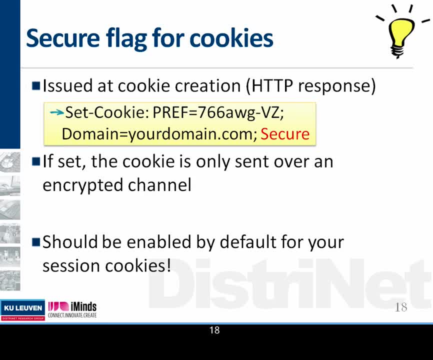 namely the secure flag. If you're including the secure flag on the issuing of a cookie in the HTTP response, then the browser knows that that cookie can only be sent over an encrypted channel. So then you can have two session cookies, one for the. 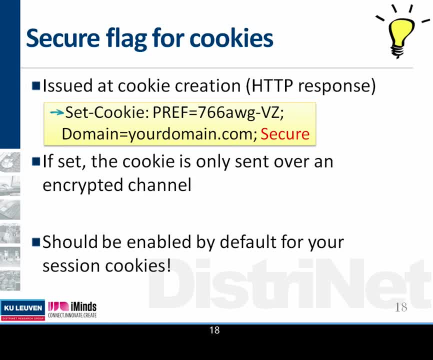 HTTP session, one for the HTTPS session, But by now you know that your HTTPS cookie will never be sent in the wild. Can you set the disattribute on an HTTPS session? Yes, of course. OK, Thank you. So in the HTTP response the server issues a new cookie. 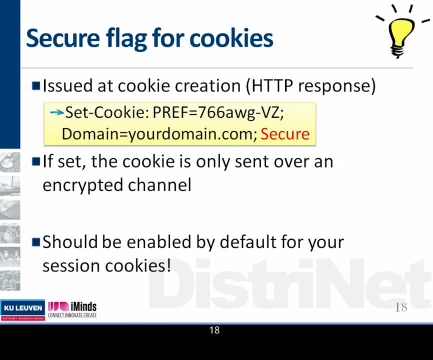 And while saying, this cookie has this value, domain and even path and expiration date. you can also add the flag secure, And if the flag secure is added, then the browser knows that it has to treat it as a secure cookie, meaning that it. 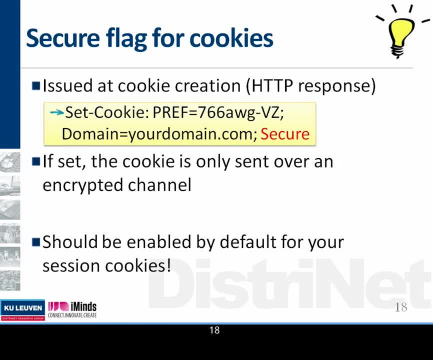 never should be sent over HTTP. But isn't it too late by then to set that flag or set that attribute, because it's traveled or probably not? Yeah, Sorry, In my presentation I don't make any distinction between HTTP- HTTPS. Of course this should be sent over HTTPS. 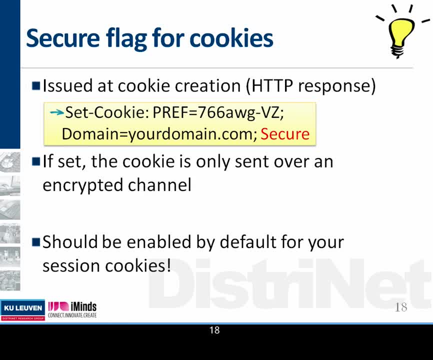 I just wanted to say the format of the request is HTTP request response, But of course this is sent over an encrypted channel. Also, in the rest of my slides, let's assume that by default we have to read it as HTTPS, because I think it's a. 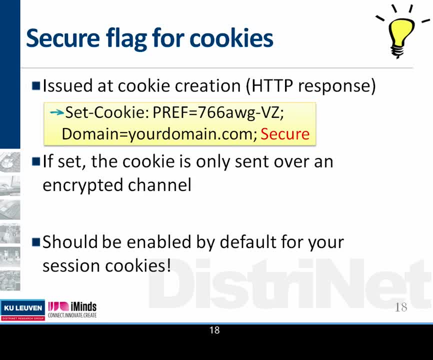 good enabler to protect your website by running it over HTTPS, Apart from problems we discussed earlier with performance and caching, But I think this should be the default behavior. OK, Even in the previous slide, you mentioned that cookies are tied to domains, not origins. 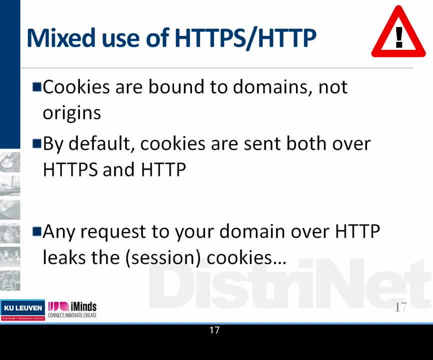 So what's the difference there? Indeed, I didn't discuss that. A domain is just googlecom And with domains in a web browsing security context, we typically have the topmost domain name, So we don't have the subdomains included. 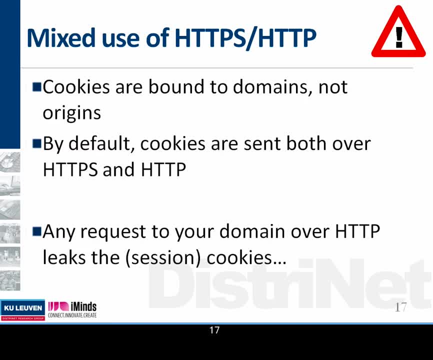 We typically discuss googlecom, facebookcom, k11.be. With origin we mean actually scheme, domain and port, So it's HTTPS, facebookcom and port 80.. And that triplet is actually an origin. And would cookies have been bound to origins? 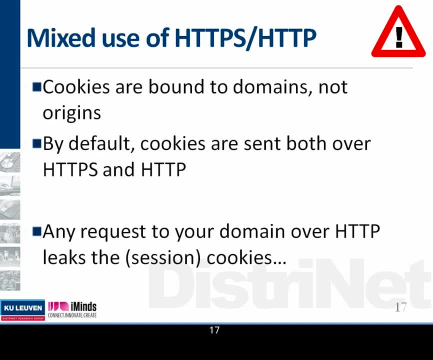 We didn't have the problem because the scheme would have been different for HTTP. HTTPS. But cookies are bound to domains. But it's interesting because we will later on also see how origins are specified in one of the techniques. OK, So secure flag. 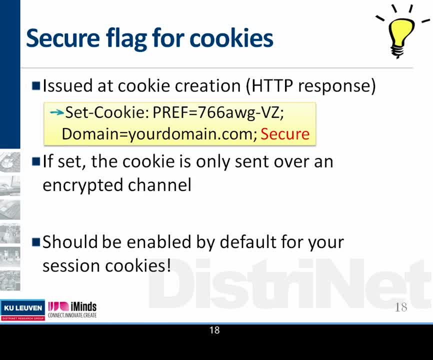 Actually, I assume that most of you were already aware of the secure flag. I just wanted to have it as a reminder. You just have to enable it by default for your session cookies. I don't see any good reason why session cookies should be. 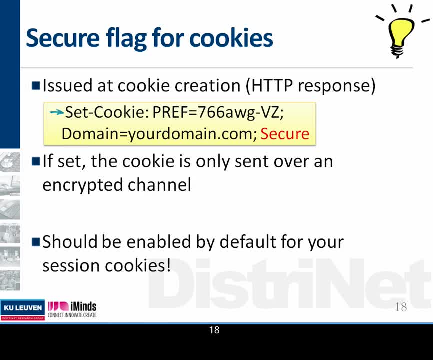 sent over HTTPS and HTTP and being the same, Because then you're actually mitigating the technique of having HTTPS in place. So it's the browser that enforces that. Yeah, Your browser is actually enforcing that, And all modern browsers are doing that correctly. 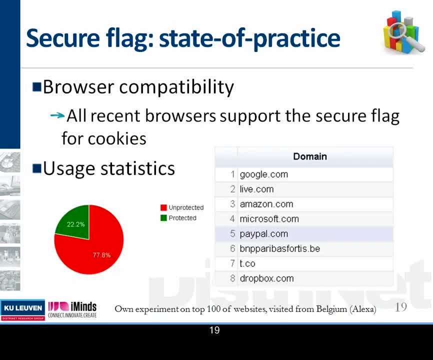 What I also wanted to do is actually, for each of the technologies I'm discussing today, seeing what is the state of practice, Just to give you some advice, some insights. in all technologies being used, what is the adoption rate? And also, in a second statistic, what is the? 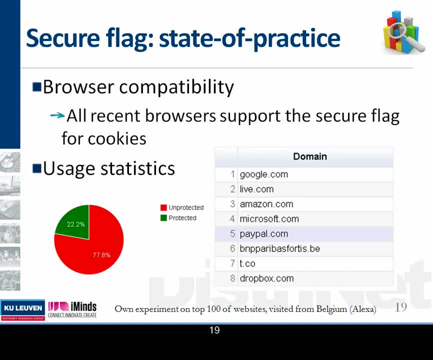 compatibility of the browsers. How well do browsers support this new technology? So the secure flag is already some old technology. So you see all the recent browsers all supporting the secure flag. If we're looking to use such statistics, we did a small experiment and I will focus on the next slide how we did. 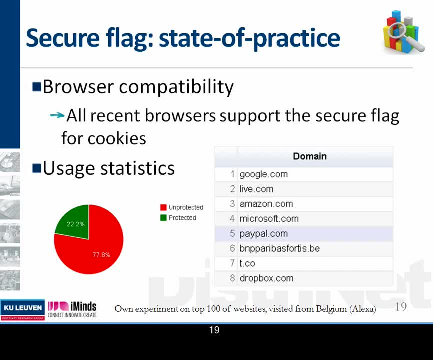 the experiment. What the takeaway is? well, we visited the most popular websites visits from Belgium, And only 22% of those were actually issuing a secure flag on their cookies, or at least one secure flag on one cookie in all the pages that we were visiting. 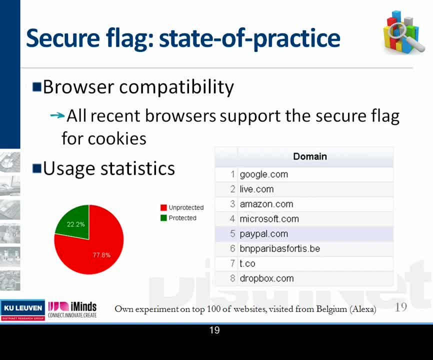 And you see, most of those domains are actually international domains that were visited from Belgium. You only see, I think, one local, One local domain specific tied to Belgium. So you mean, you have to see the flag is on in an HHPS session. 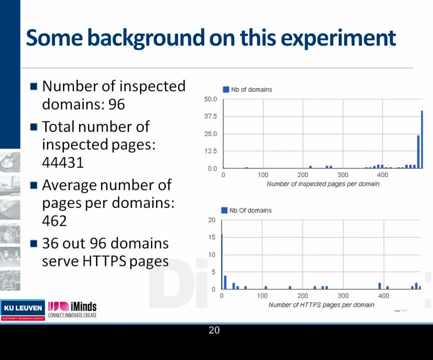 Yeah, So I will focus on the next slide. What is the data that we're using for that? So we did a small experiment. We only set it up like two weeks ago, and one of my PhD students is actually triggering that experiment. 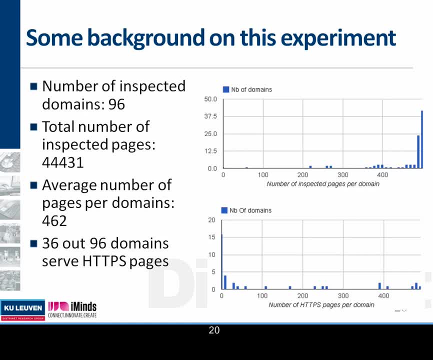 We expect that for this slide 100 domains, but only 96 of them were responding. We already increased the experiment to thousands and we are increasing even further, But all the sites today discuss about those. We have about 96 domains. 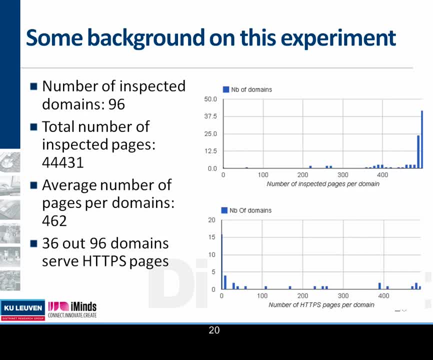 We wanted to visit 500 pages on each domain. How we did that? we actually searched in the search engines what are the top 500 pages listed for that domain And you will see some of the domains have 500 pages but some of them only have, like. 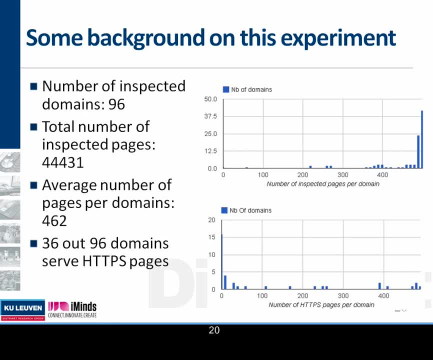 50 or 200, 400 pages that are visible in a search engine. So this means that we didn't visit 50,000, but we visited 44,000 pages on the web On average. So we have a domain at 462 pages in the search engine catalyzed and that we were able to. 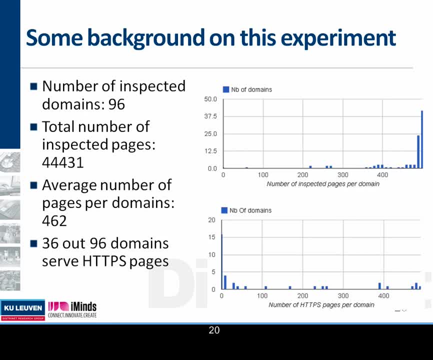 visit, And only 36 of the 96 domains were also reachable over HTTPS. Also important, it doesn't mean that all the pages were being able to visit over HTTPS. It could be that the only subset of them were accessible over HTTPS. So this is the number of HTTP pages per domain that we were able to visit. 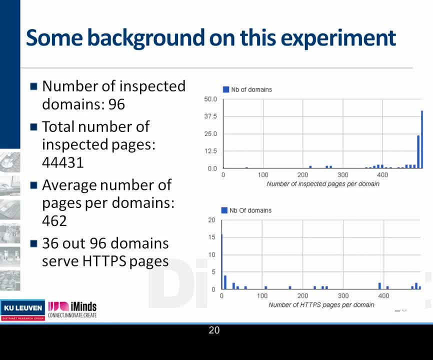 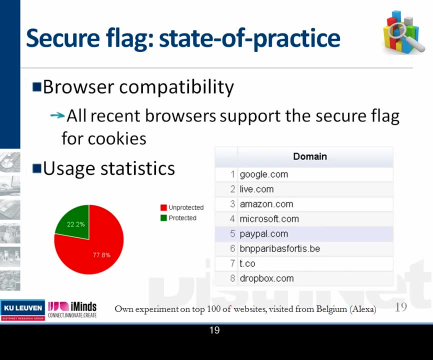 So a lot of those domains only have like a few pages- between zero and 10 pages- And the number of pages on HTTPS there are that actually serving everything over HTTPS. So we are looking back to the data on the previous slide So the 22% is actually 22% of the 36 domains running HTTPS actually having the SQL flag. 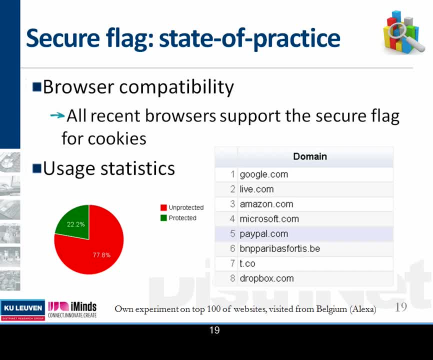 enabled, And I'm discussing this because we were actually having the same statistics for each of the features I will discuss today. So does it necessarily mean that if they both set up secure flag that they will be insecure? I can imagine they might use secure 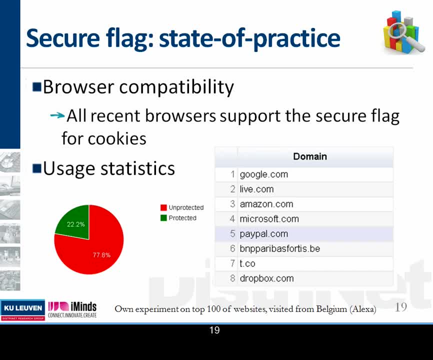 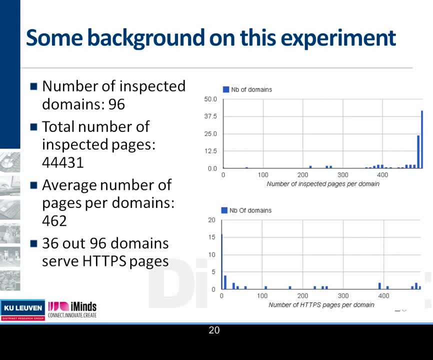 Yes, Yes, Okay, other techniques like avoiding using something else. So one thing that we could say: some of the domains that are using, for instance, only HTTPS, might be not variable for this technique, And we also see techniques where you actually can enforce the browser never. 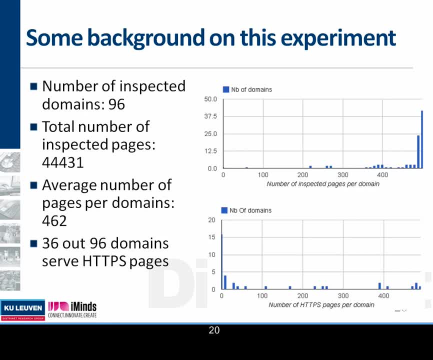 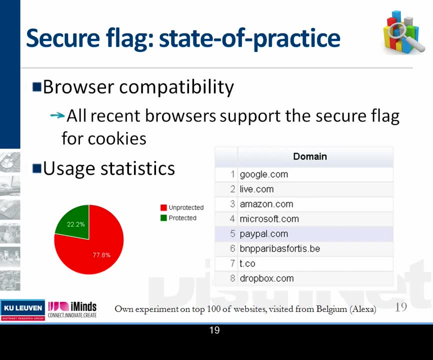 to go over HTTP for a certain domain, And for those I could say that might be good enough that they don't have the secret flag. Well, the one that is using this technology is Twitter, and Tito CEO is also a redirector of Twitter. They are actually using the secret flag as well, So I wouldn't. 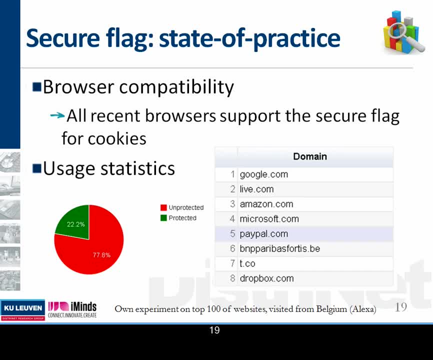 make the statement that you shouldn't use the secret flag. It doesn't hurt you by putting it into your response and it really gives you a good protection level, a first level of protection. So if someone in the audience is disagreeing having additional questions, please feel free to interrupt. 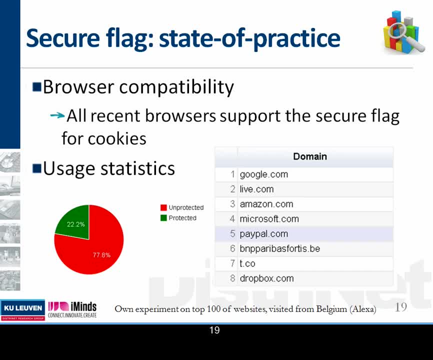 The slides will be online anyway on the SecUpDev website, so you only can see a subset of the material. I don't care, I want you to interact and to understand well what I want to present today. Okay, so we had some background on the experiment. We have the 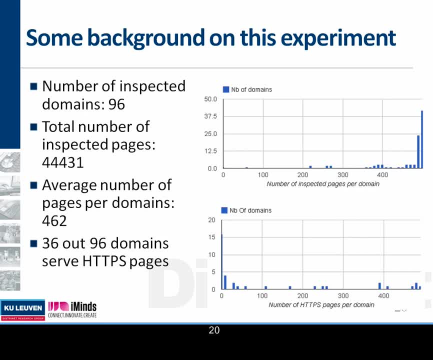 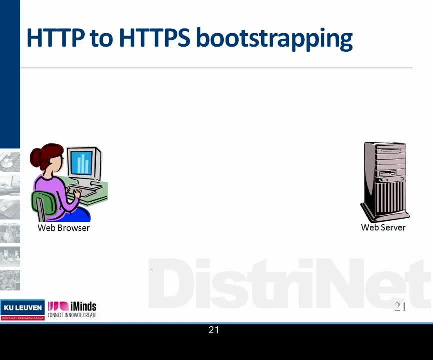 secret flag. This is just the warming up exercise. We have HTTPS and the secret flag. Let's now visit some of the other problems that are happening. One of the things is actually we need to bootstrap the whole thing If you are going to an HTTPS website. typically, 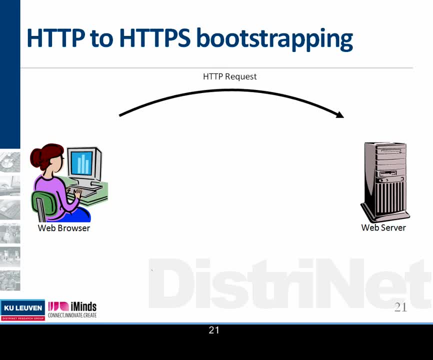 what you do is first issuing an HTTP request to the website. The website is issuing a redirect to HTTPS and, from then on, you are using an encrypted channel. This is certainly the case if you are browsing with mobile devices. How many of you are using an iPad or even your phone and entering HTTPS? 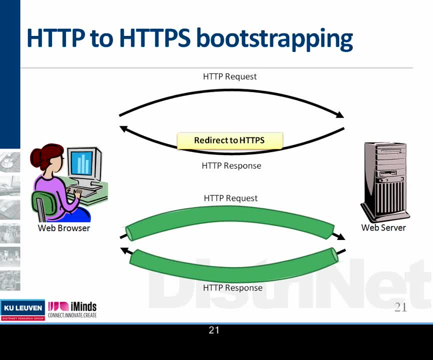 column: slash, slash. You just enter your domain name and from then on, you are going further. Well, this is actually an interesting pattern that is attackable, and it was attacked in 2009.. Maybe a little bit of background for people that want to know how to redirect. 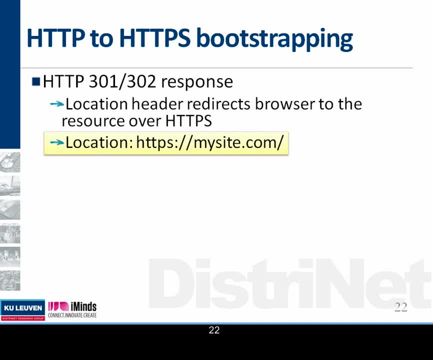 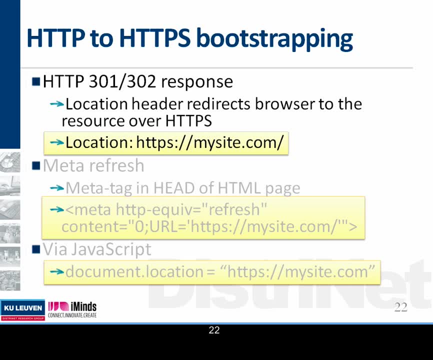 What you typically do is via a response and a location header, but there are other techniques in JavaScript or HTML to redirect as well, but we don't go any deeper on that. There is one redirection step from HTTP to HTTPS, So the SSL stripping attack explained. 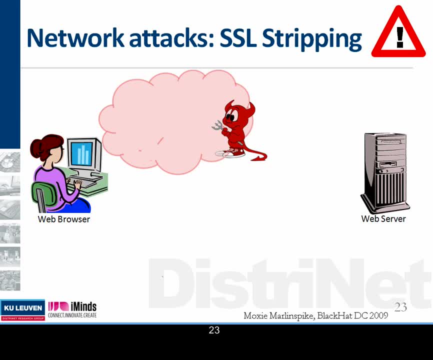 by Moxie Marlinspike in 2009 on Black Hat. Again we have an attacker on the network, for instance, close to the browsing environment. but this attacker has more capabilities. This is an active network attacker. It can handle as a man in the middle. There are several ways to. 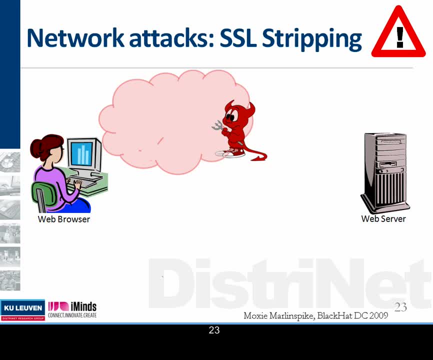 actually achieve those capabilities. Think about putting up a fake access point somewhere here at Sekabrev. Actually, I put up a WiFi in the other room, so I might have been an attacker there as well. You can even do it with all techniques as well, So one is R poisoning, actually redirecting all. 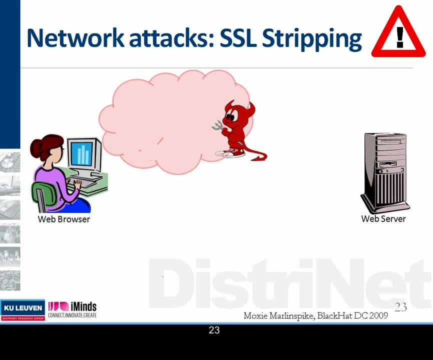 the traffic to your own and then pushing it further. But you need some kind of man in the middle to actually intercept and adapt and tamper with your responses being sent back. So the idea is the web browser is sending to the web server. It's. 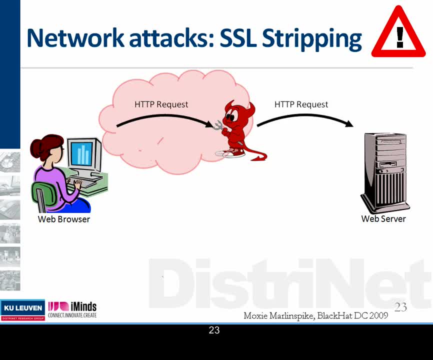 intercepted by our attacker. The attacker sends it, as is, to the web server. The web server says: oh, I want to talk about HTTPS, But the attacker doesn't pass that on to the web browser. It just is starting to communicate with the web browser over HTTP. 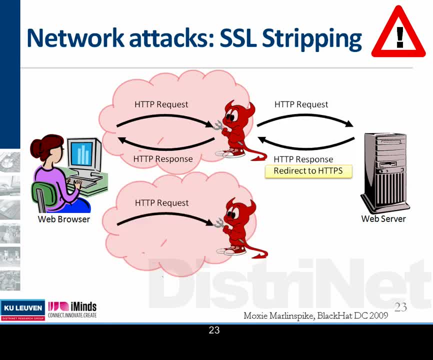 And from then on all the traffic between the web browser and the attacker happen over HTTP, But the attacker itself reflects that over an HTTPS channel to the web server. So for the web server, he's unable to detect that the endpoint is not using HTTP, He only sees HTTPS traffic coming in. 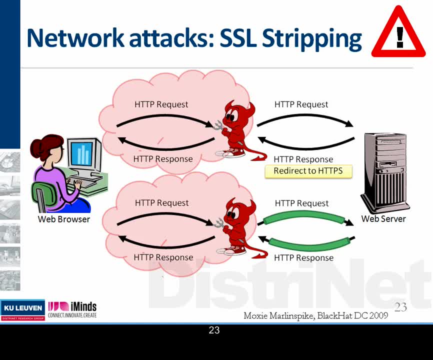 to the web server, But from here the attacker has full access to session cookies, credentials and all the alike. This is an important attack and the technology we had a few years ago. we were not able to protect against that, But luckily there are now new techniques. 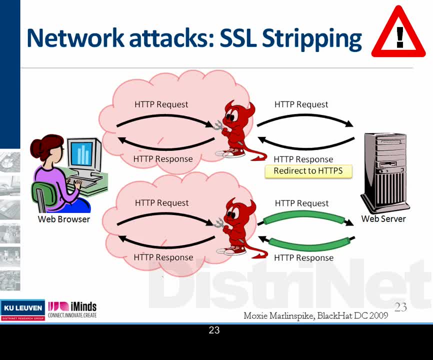 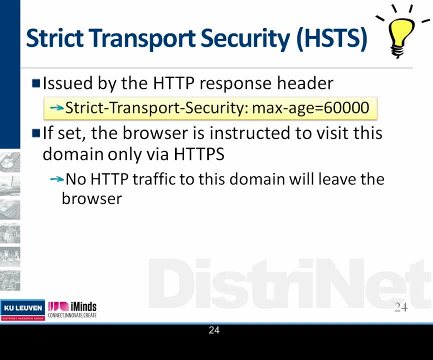 in the browser to easily protect against this type of attack, And it's called the strict transport security And it's issued again as a response header with the HTTPS response. if I say that, So what you do is in the communication with your client, you're actually saying next: 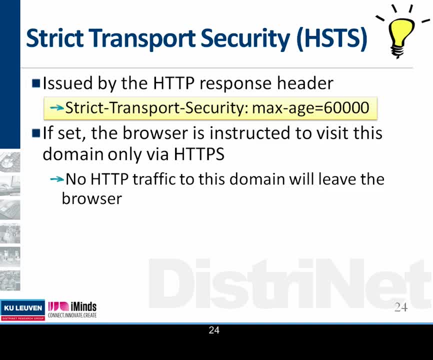 time you come to my website, don't start over HTTP. directly connect me with HTTPS And you give a lifetime, a max age, and from then on the browser is instructed to visit that certain domain only over HTTPS. It will never issue again over the channel. 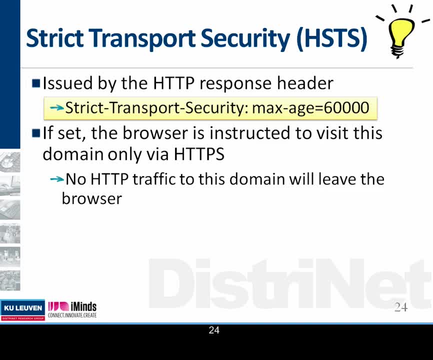 an HTTP request to that domain. Of course you have to make sure that the max age is high enough, But also you must install a max age because there might be some point in time that you have to fall back to HTTP for one reason or the other. So there's a kind of 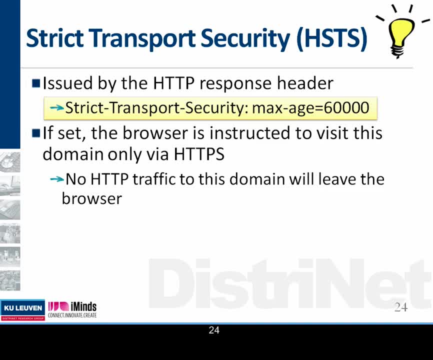 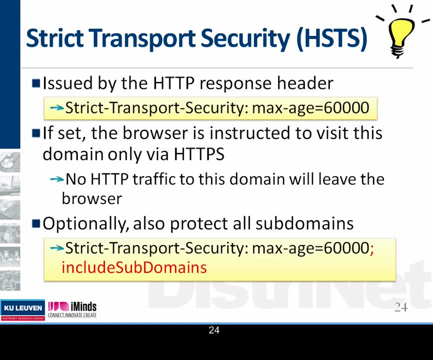 fallback mechanism. You have to renew it from time to time if you want to continue to use this. What's also interesting is that you can use this for subdomains as well, So optionally, you could also give the directive include subdomains and then all the subdomains of your domain. 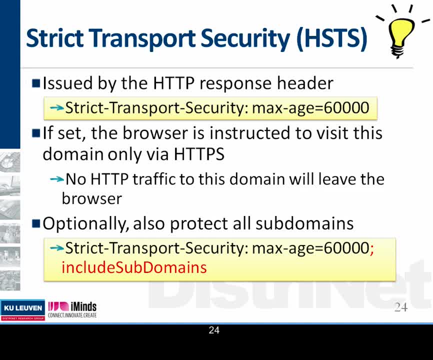 are protected as well with this technology, So there's still a bootstrapping problem. You need to be able to contact your server once before you're actually being protected by HSTS. Luckily, there are clever people in the browser community as well, So they actually 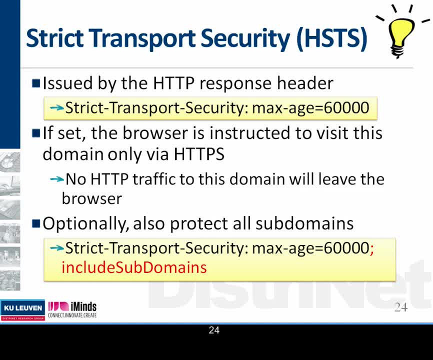 populate Firefox and Chrome with a precompiled list of domains that you should visit. with strict transport security. The list of domains is still growing. They do some kind of verification, But Google compiled such a first list and Firefox took over that list as well. So if you're going to Twitter, 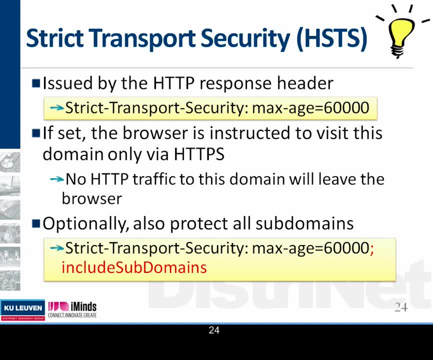 if you're going to certain domains of Google, you will by default, be protected with this technology, Which is actually nice because the bootstrapping problem stays an important factor of actually attacking it. It's only if you are redirected, if you directly, If you're directly contacting HTTPS, then you. That would be fine. 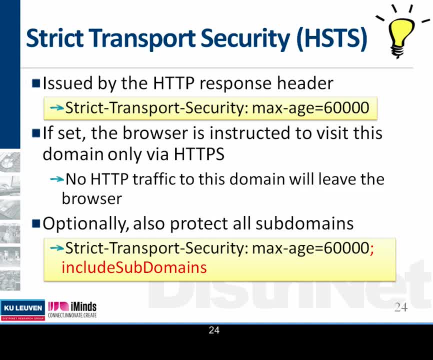 as well. So for your company website, once you've instructed your browser to go to HTTPS on your server and you're issuing this response header, you should be protected by this kind of attack. So again, let's see how many of them are protecting in the wild. 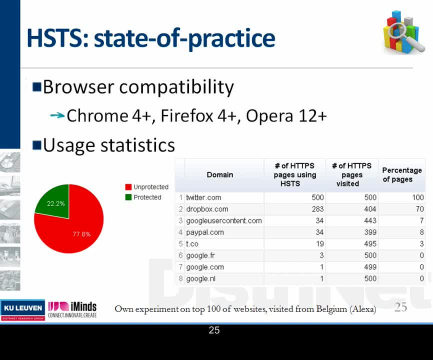 We see again that around 22% are protecting. Twitter is really the pusher in this technology, which is also proposing: Sorry, Is it per domain? that's the address set, or per web page Per domain? So you really want to protect your whole domain If you're running. 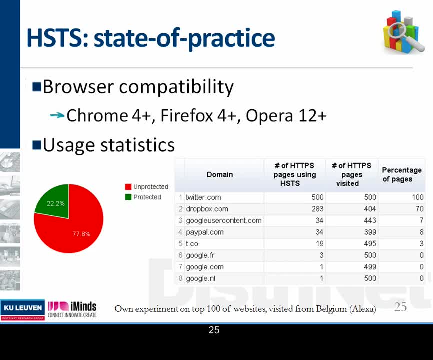 SSL. people installing this kind of features typically run the whole website over HTTPS, But that's a good question. Actually, those statistics will give you more insight on that. You're protected for the full domain, but it doesn't mean that any page on that domain will be issued a header. 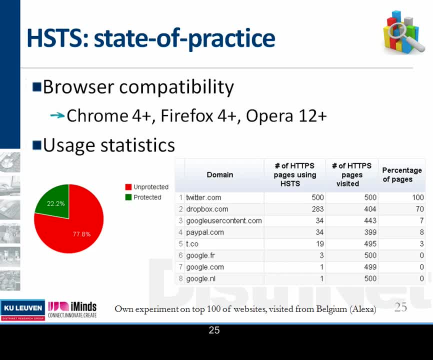 So, for instance, Twitter was one of the pushers in this technology, also actually defining the spec around this. They're using it on all 500 pages that we visit during the experiment. We also see that all the websites are using it less frequently, like 7%. 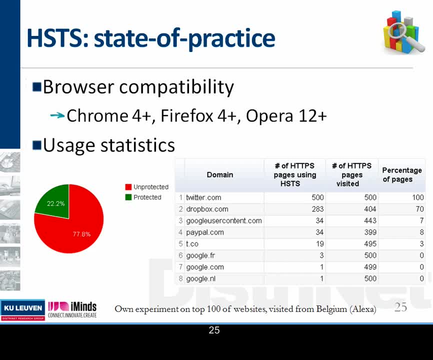 or even less than 1% of the pages issuing the header. So probably some of them are still experimenting or some of them are only on one entry page protecting their website. Do you think we can really use it, because it's not supported by the? 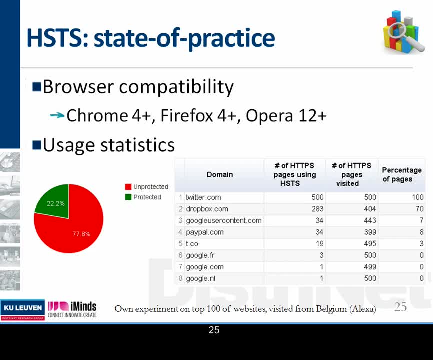 I think it's not at this moment supported, but there might be an extension in Internet Explorer 11,, for instance, actually taking that up. So the technology is quite new. It's only like one year old, and I think in the next cycle we might expect this to happen as well. We see, 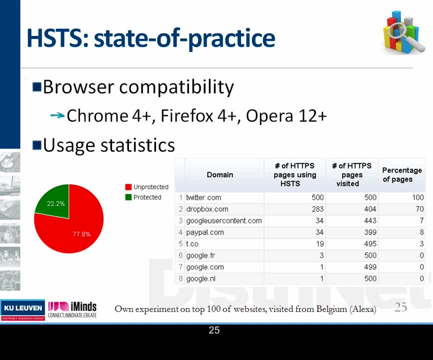 for most of the technologies today, not all the browsers will support it, but my expectation is that for most of the technology that we discuss today, within two years all the mainstream browsers will actually protect you against that. But I guess that if a browser doesn't support this header, then 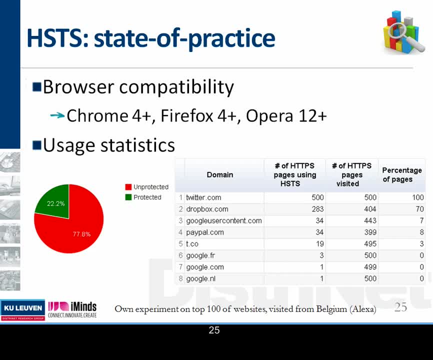 you know, too bad, It just ignores it. It just ignores it. So that's also the mechanism of using header. If you don't understand the header, you just don't process it, but you fall back to the original scenario. So you're still. 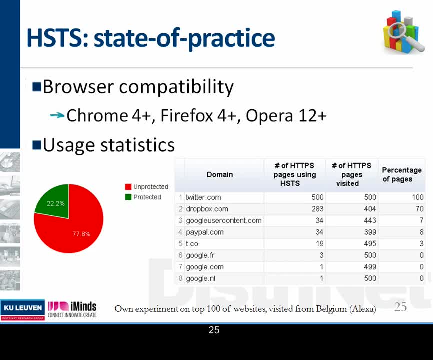 vulnerable to the SSL stripping attack, but the ones that you can protect are also protected against the attack as well. Okay, We have now a session over HTTPS. We guarantee next time that we'll be connecting over HTTPS as well. Well, we saw already in the slides of: 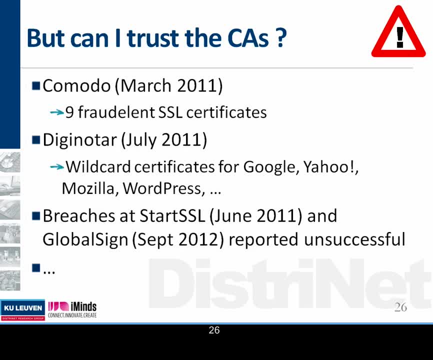 yesterday. what a lot about the CAs. We really trust a whole set of CAs in the browser. Some of them might be in some way government controlled. Some of them might just be sending out fraudulent or be very vulnerable. What can we do against that? 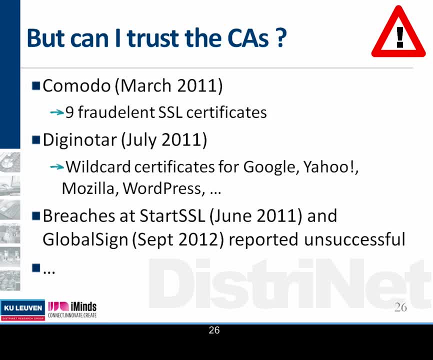 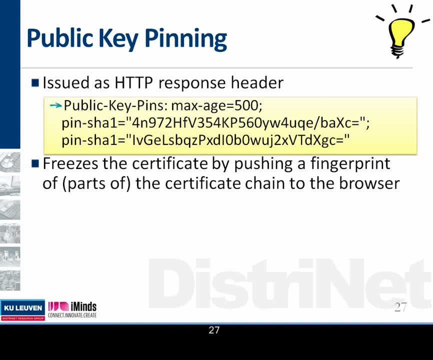 And this is technology that is still in its early days, But it actually tries to make sure that the certificates you have on your server are also the only ones that are actually representing your domain. So what the public key pinning technology tries to do is actually saying: 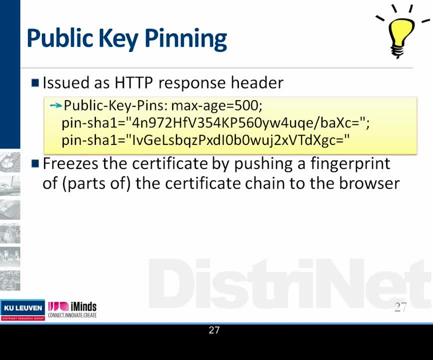 I fingerprint my certificate I'm using on my server. I'm storing this on the client side and any time that browser, in the lifespan of this header, is visiting my page, it should always see the same certificate, or at least some element from my certificate chain. 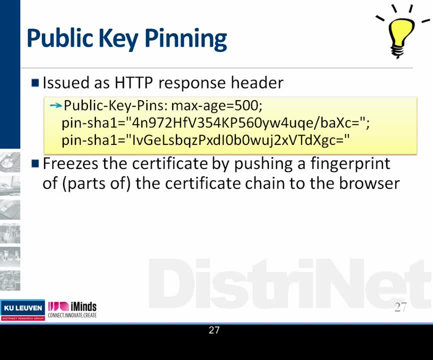 It could be that you issue only a fingerprint of the CA itself or one of the intermediate steps, but you could say: I, my certificate, is always to actually include that fingerprint in the whole chain of certificates. Important, of course, is that you also need a second backup. 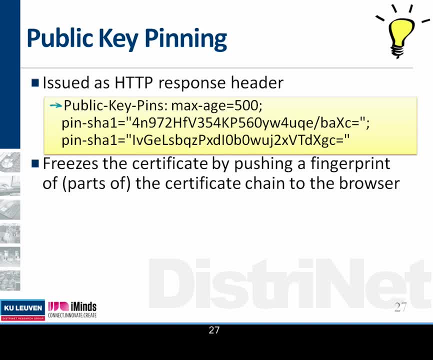 fingerprint, because if your first certificate gets revoked then you have a big problem. So typically in the spec they are all actually pushing that you're using a first certificate in production, that you have a backup certificate securely stored that you are not using actively but in case that your first certificates 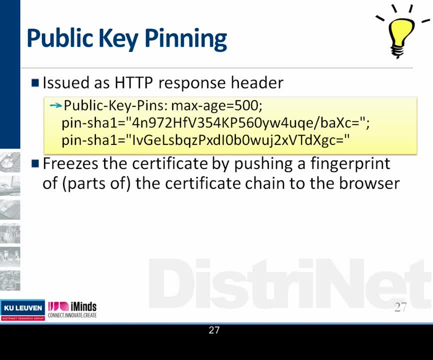 get revoked as having been compromised, that you can actually use your second to actually still have traffic coming to your website. But this technology is still in early days of actually getting shaped. But I think it might be an interesting way of actually saying: well, the whole CA problem. 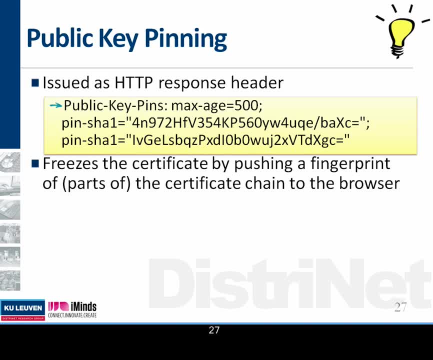 can be reduced. For instance, Facebookcom can say: anyone visiting Facebookcom is only visiting by the CA that we have chosen with Facebook And all the other CA's, all the other 60 CA's in your browser, if they're issuing something for Facebook. 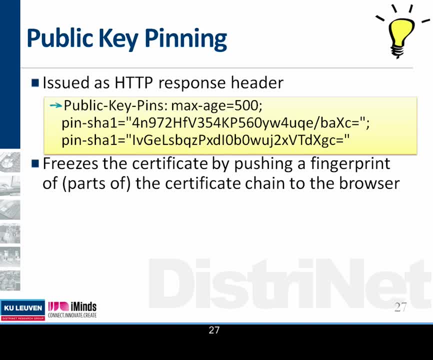 com. well, you just ignore. Again, there's a bootstrapping problem because you need to push this the first time to your client, But we see quite some traction of people interested because of the recent problems with the CA's in the last. 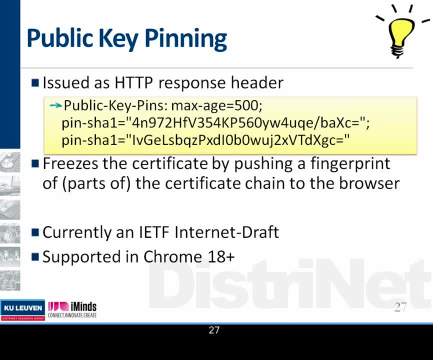 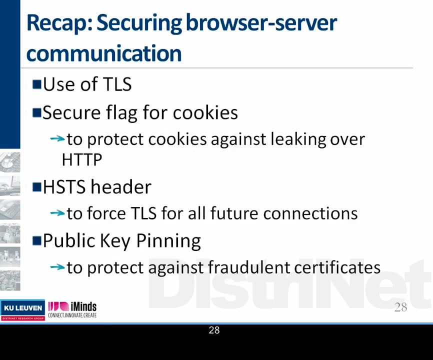 2-3 years. It's an internet draft, so it's really in the early stages, but it's now supported already in the latest version of Chrome, So they're really trying to push this as the next step. protecting the client server communication. 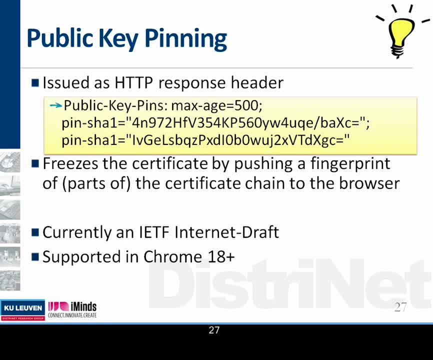 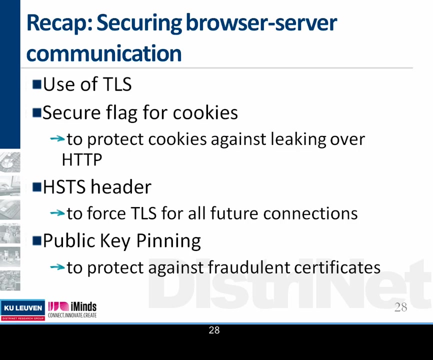 this. don't have any remaining questions, because now we're going to a completely different. 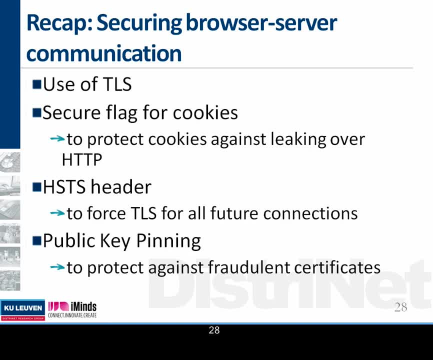 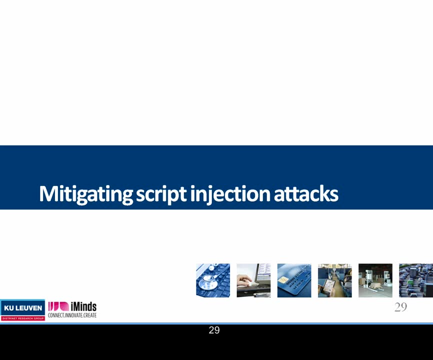 topic. So what's the next topic? So I want to actually look into script injection attacks or the cross-site scripting or the JavaScript inclusion of injection or what Jim wants to call it. Here we want to see- we have a lot of techniques against cross-site scripting on the server. 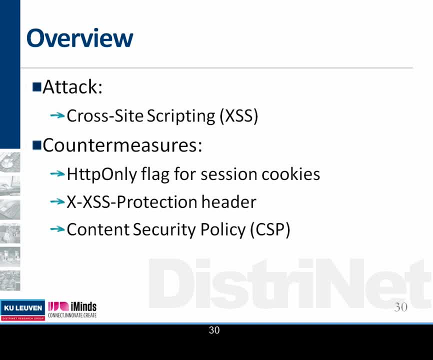 side. we have the output encoding, we have input and output validation, we have all kinds of techniques, but can we have one step further and actually protecting it as an additional line of defense against cross-site scripting, Because it's actually becoming one of the main problems in websites? it's very easy. 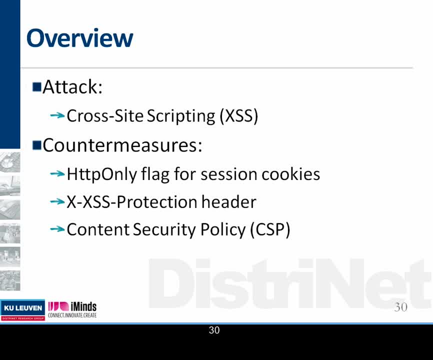 to make one mistake on your page and once you have JavaScript execution in an environment, you can do a lot of harm. You can actually mitigate a lot of the techniques used to protect your website. So we will see three countermeasures in increasing complexity, and there's only one attack, namely 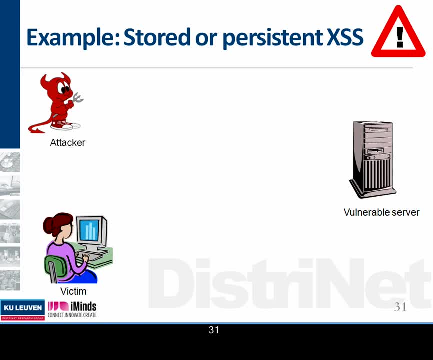 the cross-site scripting. I will just, by means of illustration, show you the stored XSS again. We already saw it on previous slides, we saw it on previous talks. The idea is you have some payload being sent to the server. the victim is downloading the. 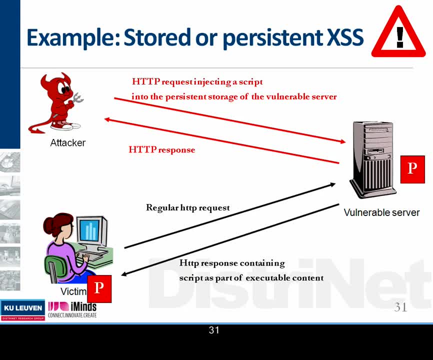 payload by visiting an interesting link, a forum, whatever, but the payload gets executed in the origin of the payload, Of the origin of the website he's visiting and at that moment you can steal cookies. you can send new requests to the website. you can read cross-site request forgery tokens. 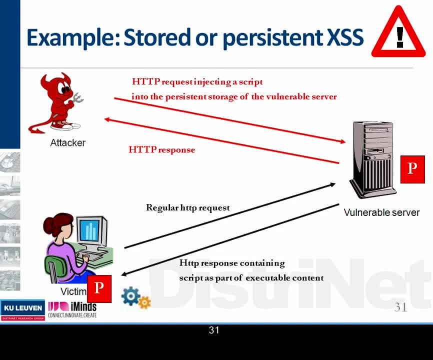 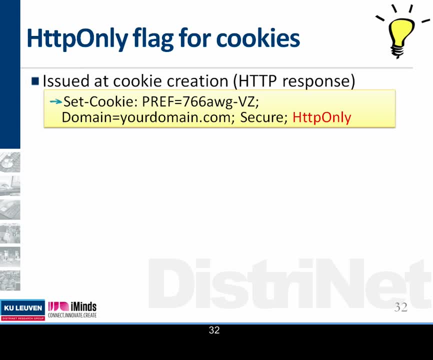 you can do the whole shebang on that domain. The first one is actually not protecting but it's actually mitigating the risk of a cross-site scripting attack, and it's the HTTP-only cookie. So the system is very similar to the secure flag we had previously for securing your cookies. 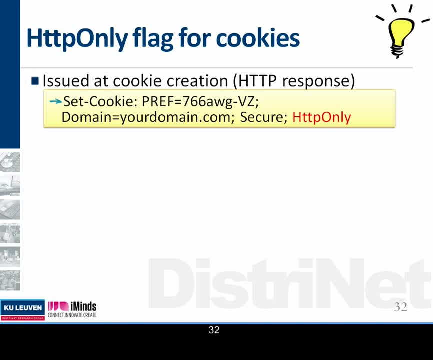 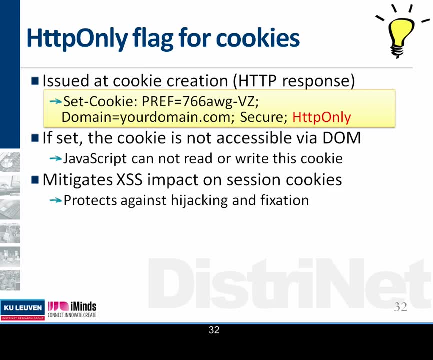 over an encrypted channel. Here the HTTP-only flag actually indicates that the cookie only should be used in communication between your browser and your server, but should not be accessible by your DOM environment. So JavaScript should not be able to read out. your cookie should not be able to update. 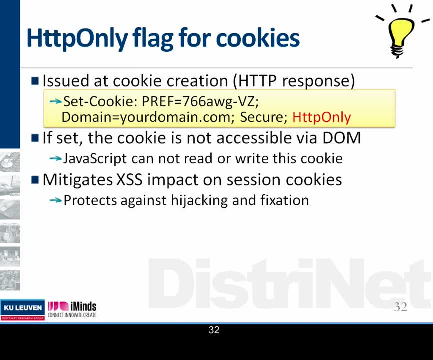 your cookie. it's only used by the browser infrastructure, communication infrastructure, to send a request to the server. This actually mitigates the impact on session cookies of cross-site scripting, because you can't hijack a cookie. you can't fixate a cookie once there is already an HTTP-only. 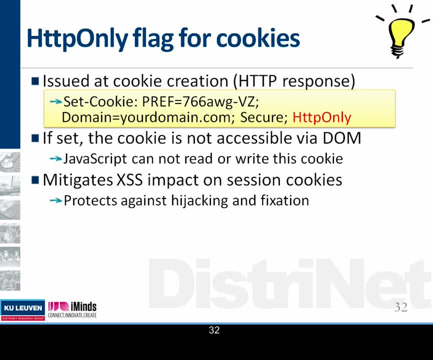 cookie in place in your browser. Again, good advice: if you have a session cookie, please enable HTTP-only by default. I really don't see good ways why you need a JavaScript having access to your session cookie or setting session cookies. We saw some of the cases where we saw different domains collaborating together, passing by 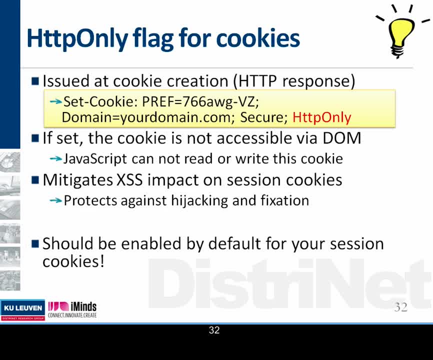 cookies by actually reading out the session cookie, passing it on. I think it would be a much better idea to actually pass on a token And then the server-to-server communication is replacing that with a new session cookie for the second domain. But that were the issues. so if you're just blocking all the session cookies available. 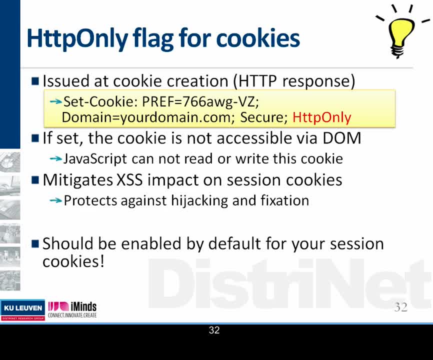 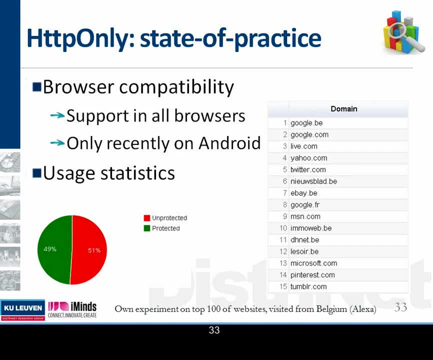 by HTTP-only, we saw that some websites were broken because they were using JavaScript to pass on the session cookies with related domains. What is the state of practice? Well, it's supported in all browsers apart from some of the older Androids. I think in 4.0 it was entered as well. 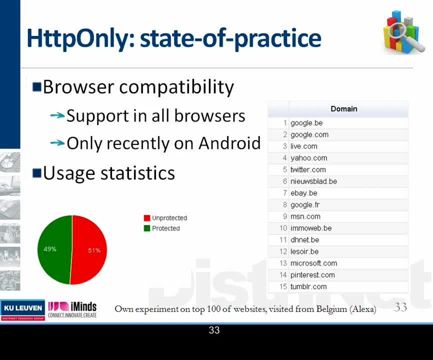 But these are statistics. Half of the domains are using the HTTP-only cookie and I think it's already a good sign that it gets traction and we should use it by default for our session cookies. So one thing I want to say about session cookies, also the SQL flag. when we did the experiment, 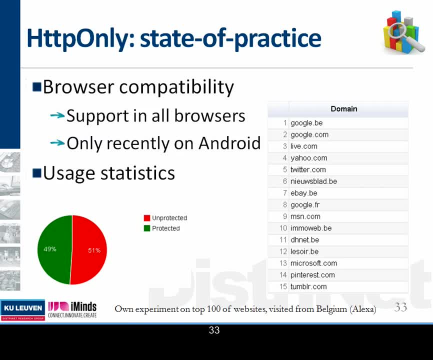 we were not sure that there were actually session cookies installed on the client side So you could have websites that you're actually crawling with the web crawl, that you only see pages that are not issuing any cookie unless you are logging in and at that moment are issuing a cookie. 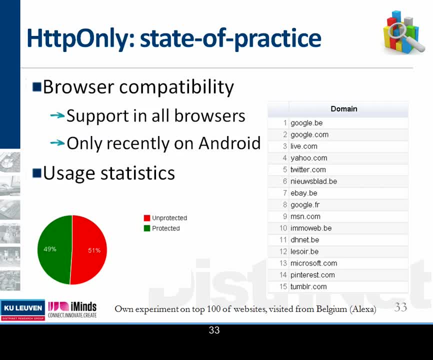 So that's one of the caveats I want to say. with all the statistics here, It could be that more domains are protected, but that we just didn't see the sensitive parts of that website. So very basic technology. The next step is actually a default technology that is enabled by default. if that was the 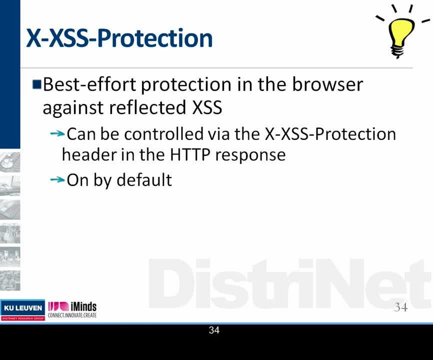 only question. This is the XSS protection header. The XSS protection is actually a mechanism already in place in the browser, but it allows website developers to control to what extent the protection should be protected. Okay, So the XSS protection should be on or off? 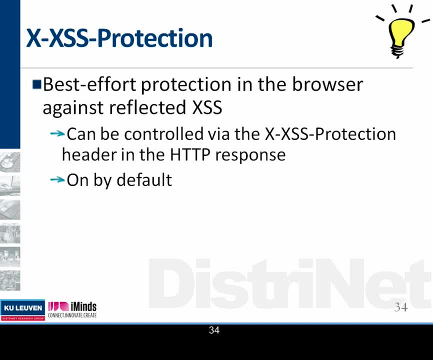 But by default, if you don't send anything to your browser, the protection will be on in your browser. And what does it do? It tries to protect against reflected cross-site scripting. It means if it sees a string in the URL and sees that string being executed as part of. 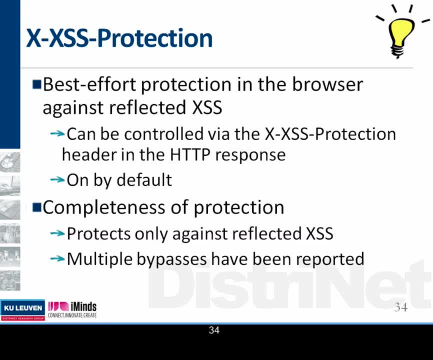 your page. it will actually try to block that execution. Important to say about the completeness of the protection: it's not foolproof. It tries to protect in the best effort against reflected- sorry, reflected cross-site scripting, But we saw multiple bypasses being reported in the past few years. 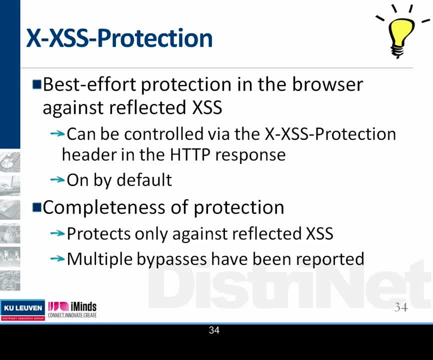 But it's an additional step, a little bit raising the bar again. So the default: I want to insert an alert on a forum with a reflected cross-site scripting typically will be catched by this technology. So where is this technology being deployed? 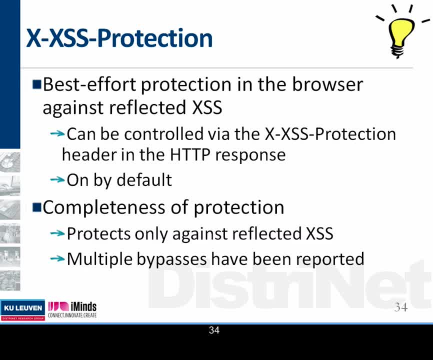 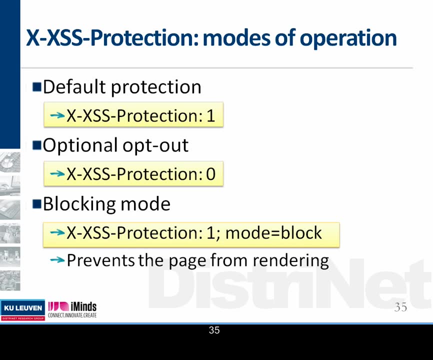 In Internet Explorer, Safari and Chrome. But the problem is, some of the websites actually suffer from this technology being able unable by default, And therefore they actually made a mechanism to control whether you should actually have that protection on or off. 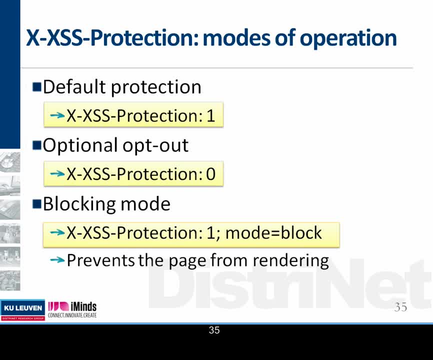 So you can control it with the header XSS protection by settling it to one or to zero, if you want to, optionally out. If you don't send anything, it's equivalent to actually settling it to one. There's one additional mode, the blocking mode, which means instead of actually rendering, 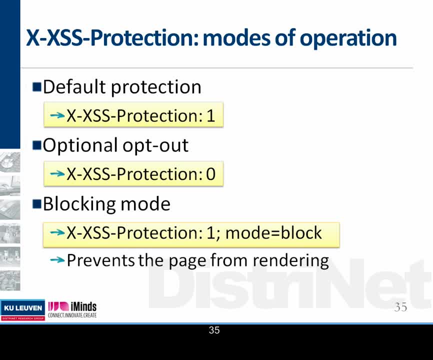 the script execution useless. you could also block the whole rendering of the page and display it to the end user So that there might be a harmful script as part of the website itself, and that's typically what Internet Explorer is doing in blocking mode. 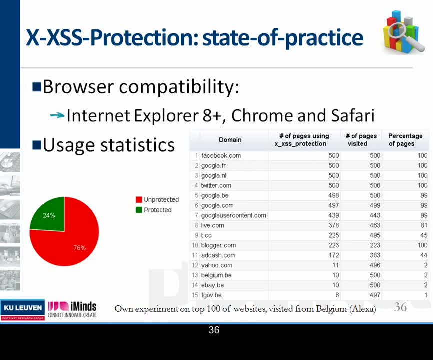 So from Internet Explorer 8 on Chrome and Safari, I think it's called XSS Auditor in the other two, in WebKit, we see one fourth of the websites actually using this technology by configuring Here. it doesn't give you an indication of how well they are protected. 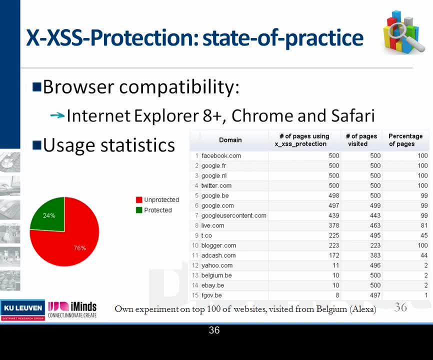 So the unprotected protectors is not purely correct. it actually means they're already taking it into account. but it's the browser that decides. I want to push this technology or I don't push this technology. So you see the difference. I'm sorry. 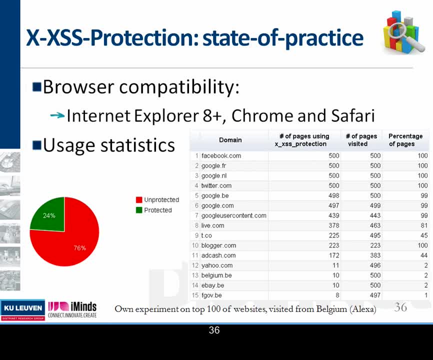 So protected in this context means that the header is explicitly protected. So I don't have the data here on the slides, but I looked. I only saw, I think, one case where it was disabled and all of them were actually specifying one or actually specifying. 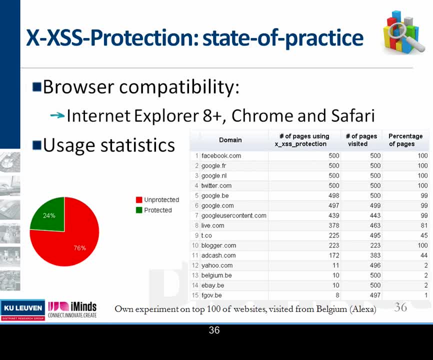 one in the block mode. So it's not that they are disabling the protection, but rather actually explicitly saying I want to have this protection. So it might also be legacy. I'm not aware of that. It could be that, for instance, the first version of Internet Explorer did not turn. 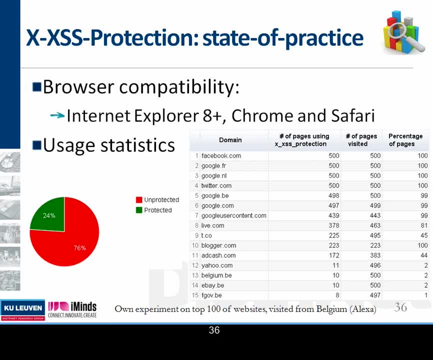 it on by default and only in the second iteration it put it on by default, but people are sending out this header. With respect to browser compatibility, in one of the previous slides you said the app was only on the latest version of Android. 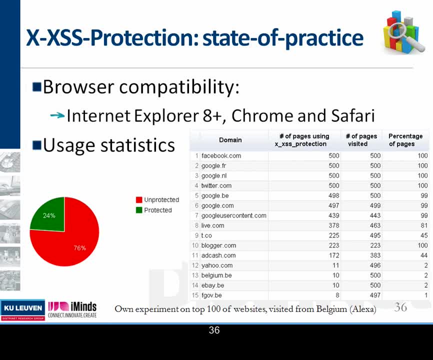 So if you're mentioning Safari, there's a little bit of a difference between the two versions. What's the difference between the two versions? There's a little bit of a difference between the two versions. There's a little bit of a difference between the two versions. 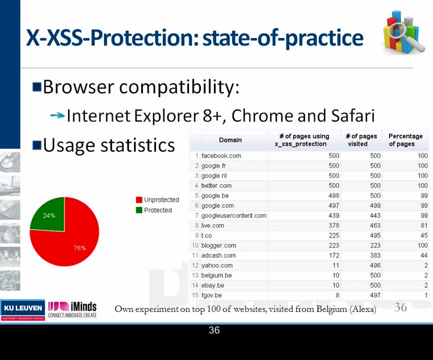 There's a difference between the two versions. Do you think that both include Safari on OS X and iOS? I think so because they're actually implementing this XSS order as part of WebKit. But, to be honest, for all the browser compatibility, the moment I'm actually presenting the slides, 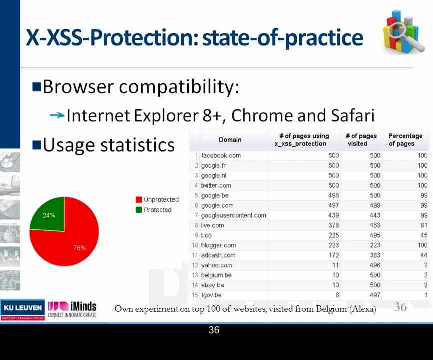 the information might be outdated. There are good websites actually for each of those technologies, rendering on a very, very frequent base what is actually protected in which or what is supported in which browser. So if you want to know that, I would actually try to refer you to that. 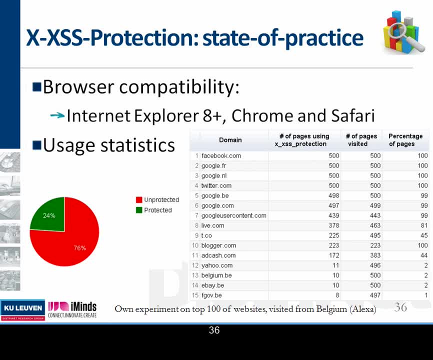 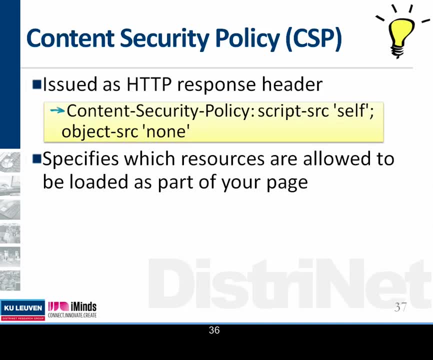 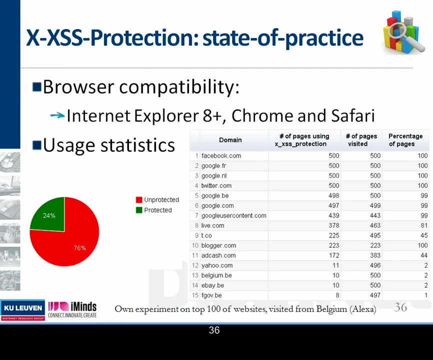 We can do it also during the break. There are good websites actually indicating what version of each of the operating systems is actually supporting this. Okay, this is all basic. Now I really want to go to the core of the presentation. Jim already announced it during the keynote, announced it yesterday. 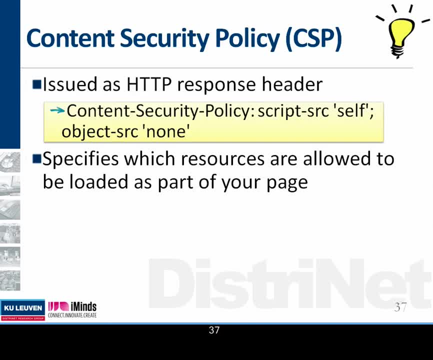 It's about the content security policy, And I think this might be the most promising technique of actually protecting against cross-site scripting as an additional layer, without touching any of the code on your web application, With a small caveat. We'll discuss that later. 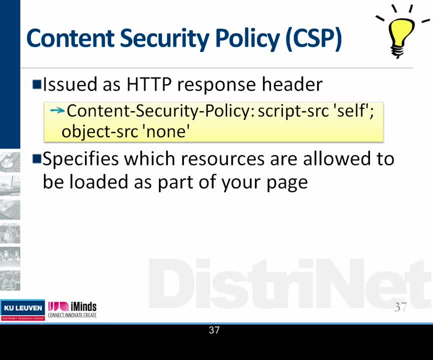 What is the idea? As a website, you're actually on a per-page basis. you're issuing a response header that says: what is the security policy for that specific website, And the security policy describes which external resource or which resources are allowed to. 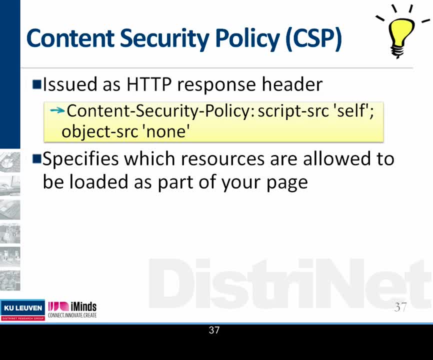 be loaded as part of your page. We'll discuss a little bit later on what are the different types of resources, But I think for what I have in mind, we mainly focus on which scripts And which frames can we actually include in a web application. 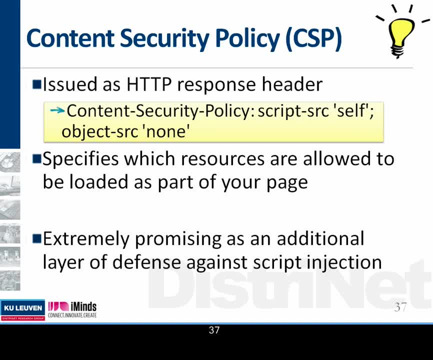 So I already said that it's very promising, And we'll see also that it actually is an enabler later on for actually making a good security architecture by using this technology. How do we actually set up the policy? So the policy here might be a little bit obfuscating. 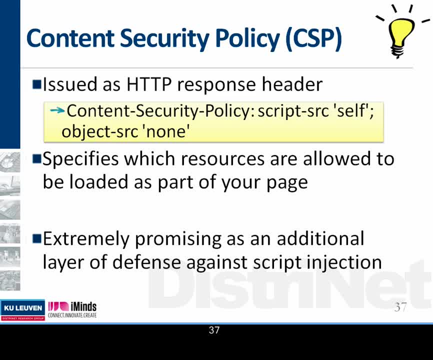 But here the policy itself is to say: well, you're only allowed to load scripts from your own origin And you should not have any plugin, And you should not have anything installed in your browser. This is just very short, what this policy means. 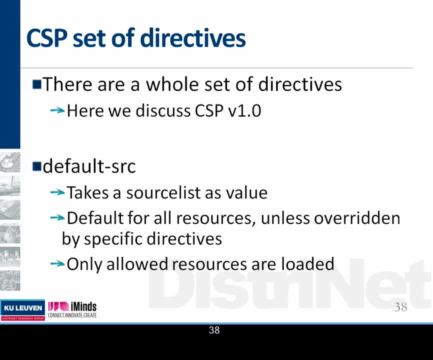 But we'll go in a little bit more detail how we can actually set up the directives of CSP. In this talk I only will discuss CSP version 1.0.. This is the one that is being drafted. It is being actually pushed towards a standard. 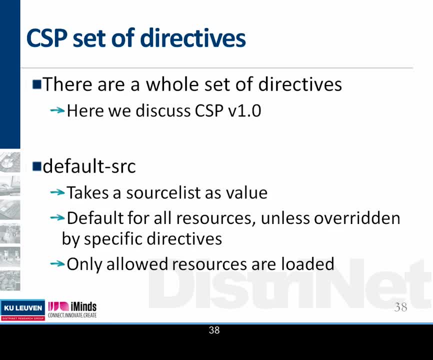 They're already working very hard on version 1.1 as well, pushing additional features, And it's my personal feeling that a lot of people, and especially, for instance, Adam Bart of Google, They're working very hard to absorb even the features I'm discussing in all the parts. 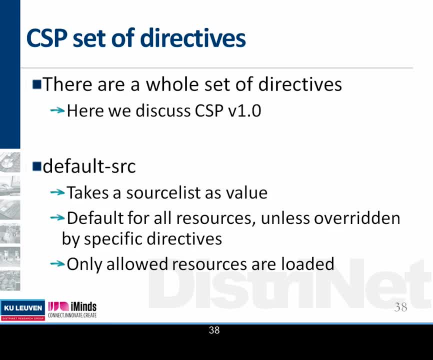 of my presentation as being part of the content security policy. That is really the default policy. you push from your server to the browser, protecting against all kinds of attacks that they can protect in this way. The main directive is a default source. Anything you don't specify in header can be specified by the default source. 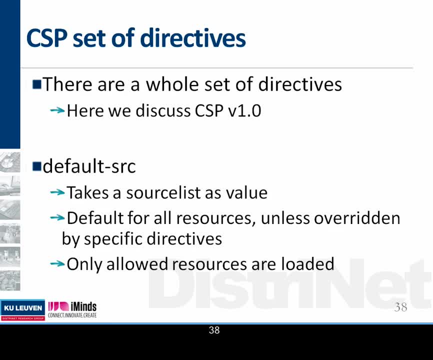 And as values. it actually takes a source list And we will see a few examples of the source list, And it defaults for all the resources- All the resources, unless explicitly overwritten by specific directives- And it mentions which resources are allowed to be loaded as part of your page. 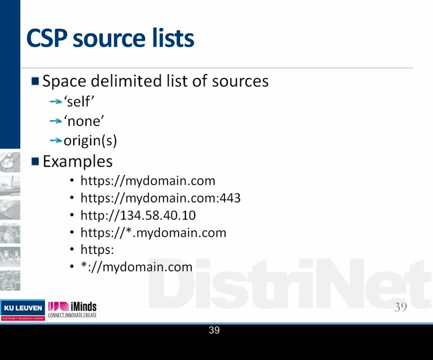 And loaded, I mean being fetched and rendered in your page. The source list itself can say well self, which means the website itself. None, if you don't want to have any being included, even if from your own website, And origins can be presented in different ways. 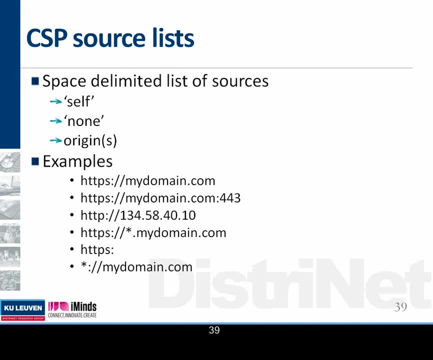 For example, the scheme, domain and port. So this is the traditional representation of an origin. You can omit a port, You can use IP addresses. You could have wildcards for subdomains. You could have also wildcards for the scheme. 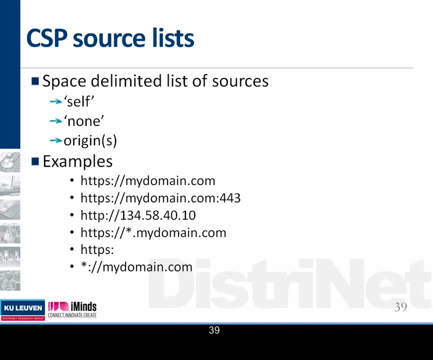 And you could even say: I only want to specify the scheme, Which might be an interesting enable that we will see later on. to say I only want to have secure content being included in my page, What does it mean if you use an IP address? 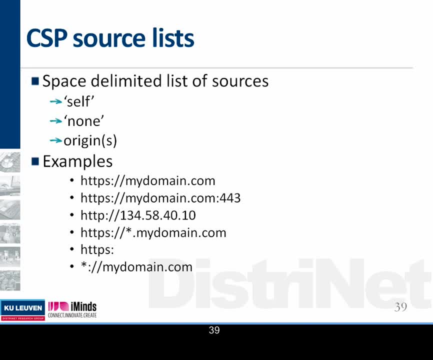 Does that mean all the websites that are hosted? I think that are specified with an IP address? I don't think it's hosted on an IP address But to be honest, I didn't see any mentioning of that in the specification, But I should look it up again. 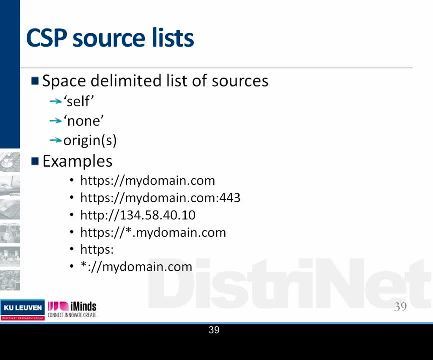 But in my interpretation it was: if you specify directly an IP address, then that resource will be fetched. It will not do the check by DNS lookup and then look to the IP address. I think Also important- and Nick and Steve will talk much more about that- 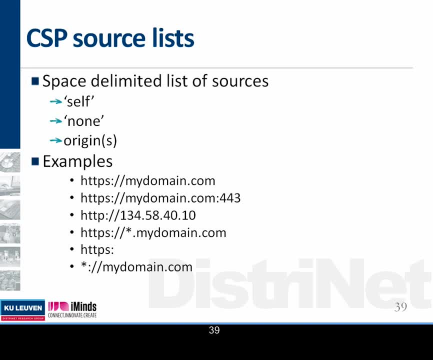 But IP addresses might not be such a good idea, And especially what we see in the wild is they're using 127.0.0.1.. And that's quite easy to generate on your own PC, for instance. Or they're using an internal network IP address, which is also quite easy to generate. 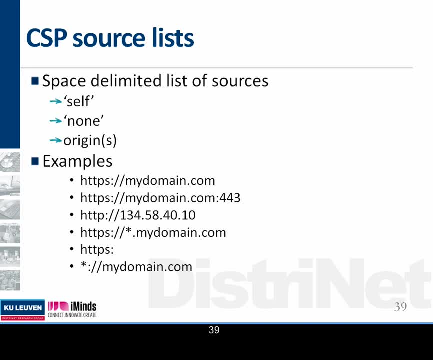 Certainly on, for instance, public Wi-Fi and so on. Personally, I'm not such a big fan of using IP addresses, Especially if you're deploying your website in a testing environment And then you need IP addresses because you don't have resources. 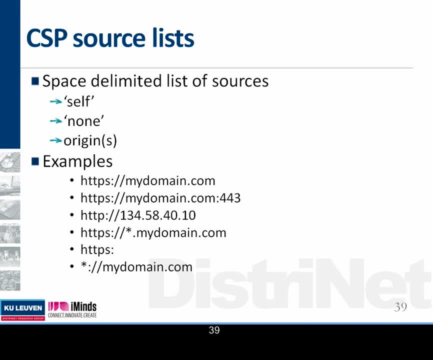 Or you need local machines To load the NetBeans or whatever. Make sure that it doesn't be pushed to the production environment Because it really can hurt you. Attackers can really use that attack. But more of that in the talk of Steven and Nick later this evening. 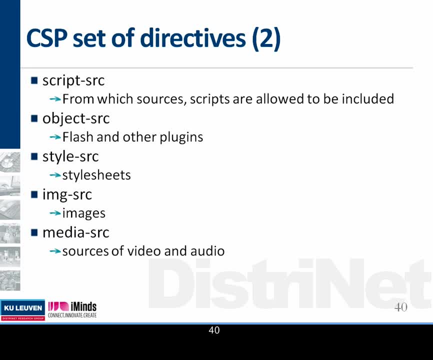 I won't discuss the whole set of directives. I just wanted to include them in the presentation so that you have kind of reference And so that we have an idea of what kind of resources we can protect with CSP. Import all the scripts that we can say which JavaScripts are allowed to be included on our page and being executed. 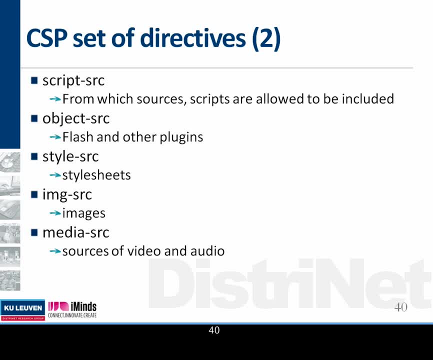 Objects, or actually the whole subset of objects, which are mainly, for instance, the Flash or the Java plug-ins being enabled in your application. You have also style sheets, And we didn't hear anything about this in the previous talks. But if you're talking about script injection, disabling JavaScript is not protecting you completely. 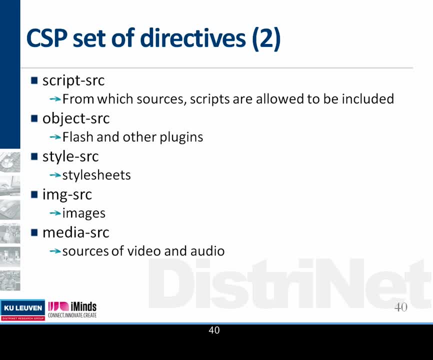 There is an interesting work of Mario Heiderich which actually goes on scriptless attacks. with style sheets, CSS, You can do very similar things As executing a whole environment. I think the people of W3C even say: with CSS they have a true and complete machine. 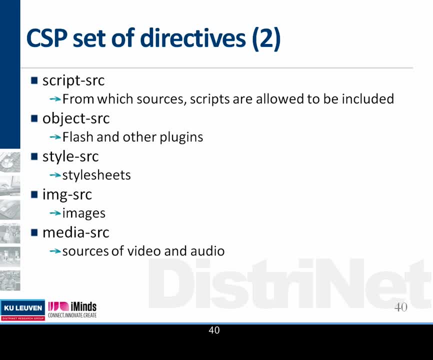 So they can actually execute whatever they want in the CSS. Interesting thoughts, But we don't go in any deeper in this talk. What we also can specify is what images are being loaded from: Audio and video, Frames, Fonts, Web fonts that you can use. 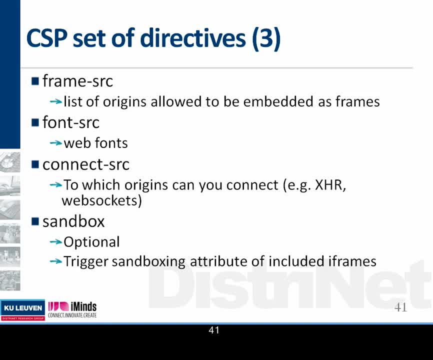 And the Connect is actually a bundle of all the ways where you're actually all interacting with each other. Okay, So you're actually connecting over the web, over the network. So XMLHttpRequest is the basic one we have in mind, But also WebSockets follow the same directive of Connect. Source. 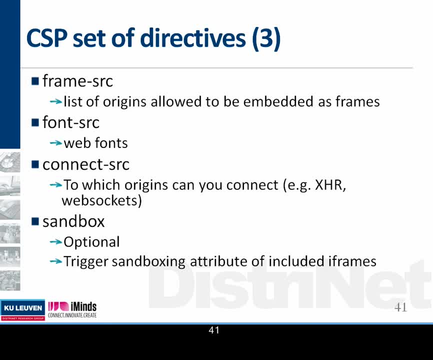 So this is the only one that is not actually including, But it is actually discussing about outgoing requests. Actually, this is what: to which origin are you allowed to connect? Or then, which of the origins can connect to you or push resources to your website? 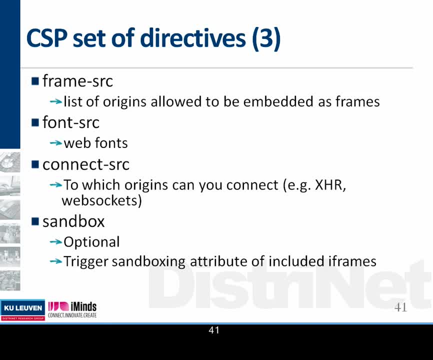 One optional thing is Sandbox. I included it here to mention it Because it actually will trigger all the technologies that we'll discuss later on with frames, Which is actually using the Sandbox attribute in HTML5 for iframes. So you can specify it with CSP to actually enable the Sandbox attribute on the iframes you are including. 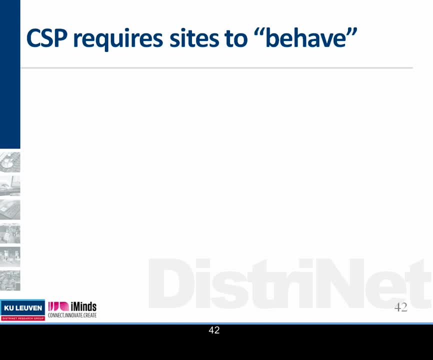 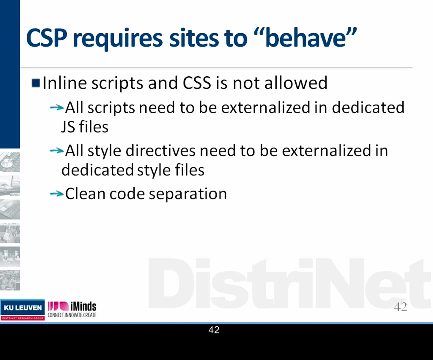 One problem with CSP- And problem is not the correct word- One interesting side effect of CSP: In order to operate, It needs websites to behave. And what do we mean with behave? Well, we have two steps. The first step is we should not allow any inline JavaScript or CSS. 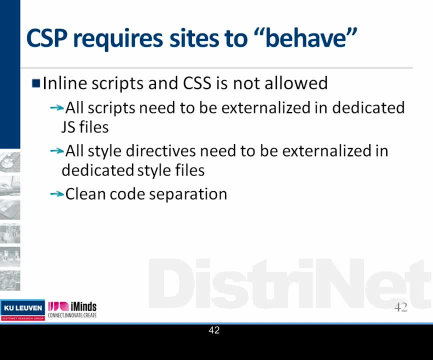 So all the JavaScript needs to be externalized, All the style directives needs to be externalized in style files. It has the big, big advantage of having a real clean separation between code rendering directives and the data itself being in the HTML. The side effect is: 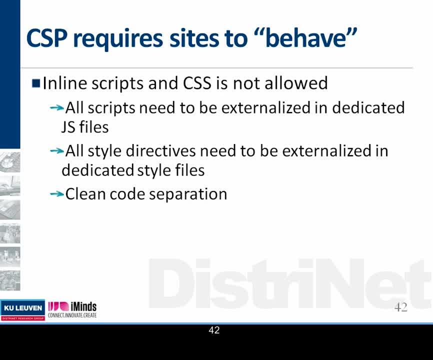 It's very hard to refactor existing applications. Think about your application of about 100,000 line of code And HTML being all wrapped together. Try to externalize all your JavaScript. So it might not be that easy to do, But I think. 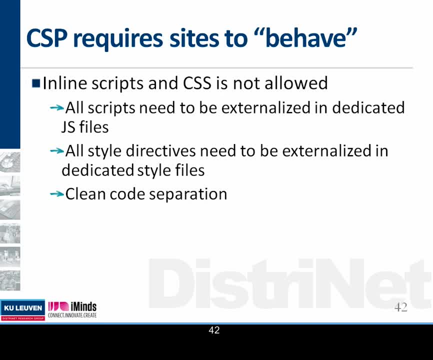 And Jim also mentioned it already on the first day of the second series. I think it might be a very good way of actually enforcing it on all the newly developed applications, Apart from being using CSP, Because it actually gives you the good separation between what is code. 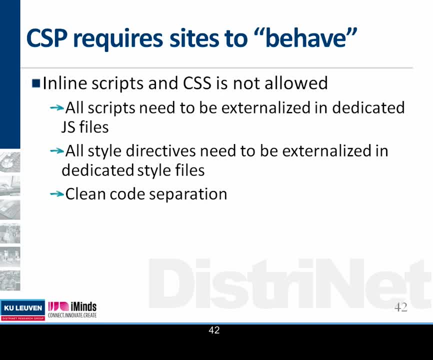 What is not executable. So this is one of the things that actually might slow down the adoption of CSP. The second one is you are not allowed to use eval, And the reason for that is If you are using eval- Any string- even on the pages that do not contain any JavaScript. 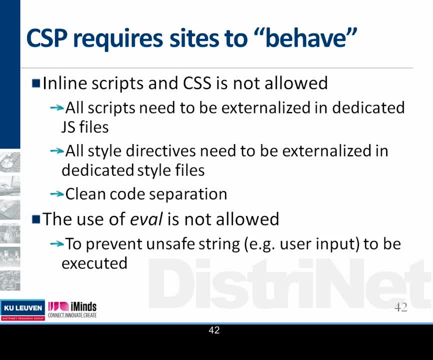 With eval could turn into executable code, And this is also something that is having a big impact On which of the sites, Which of the JavaScripts, I actually can use this technology. Yes, You say that JavaScript is not allowed. Is that enforced? 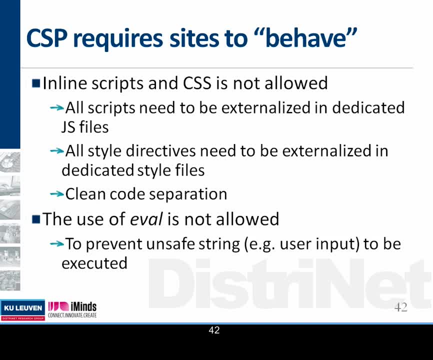 That is enforced. Yeah, But I will discuss. There is a way out To bootstrap the whole process, But in fact You should go to a website Where you actually The JavaScript itself Is actually having the code And the binding technology. 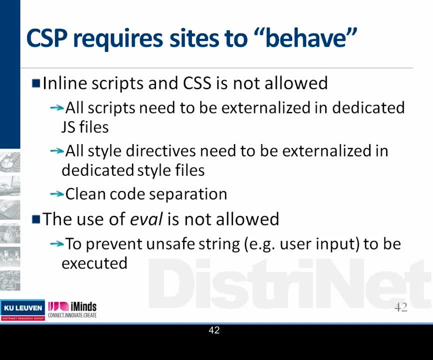 To bind that code To your HTML page itself. So even if you specify a script, Source equals self, So you allow JavaScript to load from itself. Then having a new JavaScript Isn't that sort of the same No, So I will discuss my example. 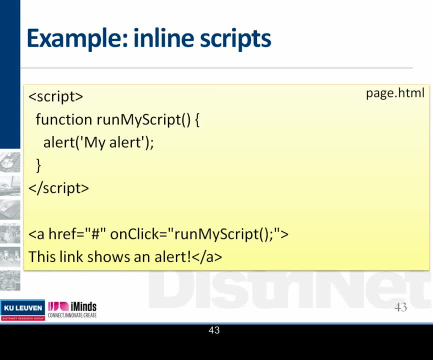 And I will come back to that question Because I think it is a very good question In that respect. So I will first show. This is typically the normal code For people not separating JavaScript and HTML. We have here an anchor tag. 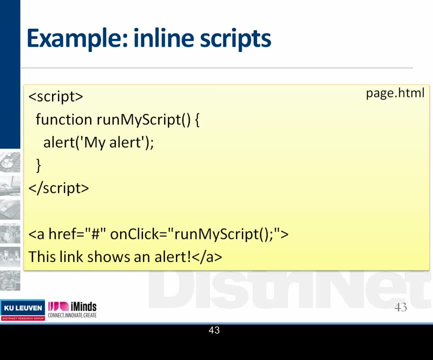 Once you click, You run MyScript When MyScript is actually showing an alert. Again, This is not the perfect example To convince your managers That JavaScript is evil, But for me It is the easiest way To actually show. 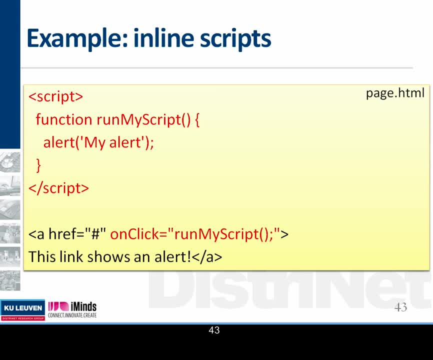 That something is going on. The problem here Is that we have inline JavaScript In our page, So even Between the script tag We are declaring our function. We are also having the call In the onclick handler Why we have to go to. 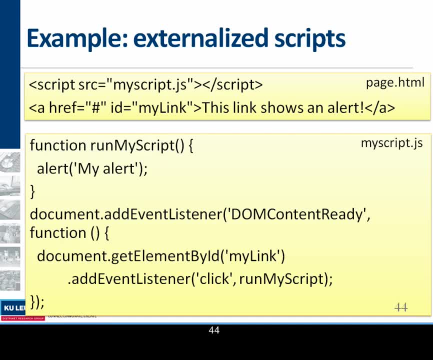 Is that we actually Say we are including script From our own website, But we don't have any JavaScript Being specified on this page, Apart from loading A JavaScript resource, And the code Here down Is again the same Function declaration. 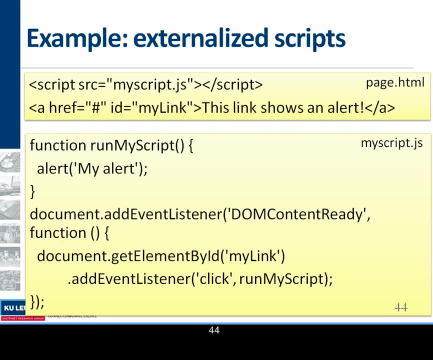 And then you have some code Of actually adding An event listener To content That is searched by My link. So, Indeed, If you are looking to this code, It is making Somewhat complex Than writing it inline. 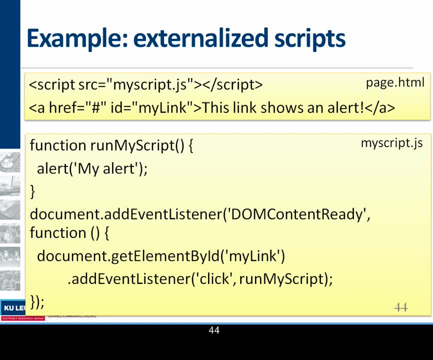 On the other hand, This should be abstracted, Actually, By the tools you are using To develop your applications, And it might Still take some time By tools to actually Generate that code, But this should Be much easier. 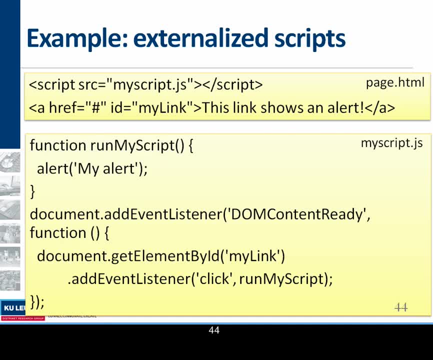 To say, Well, If we have The code Being set Here, We can actually decide Where The code Should be allowed To run Or not to run. If you see The spaghetti Of all the code. 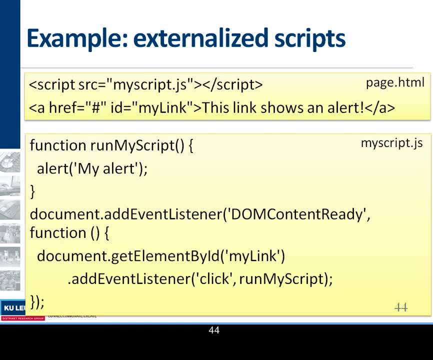 And the HTML Being mixed, I think both of them Have disadvantages. Yeah, But If you Go To the reverse Data, We try To find Solution To directly, To see Directly. So If 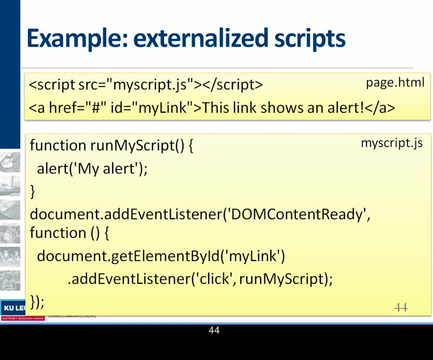 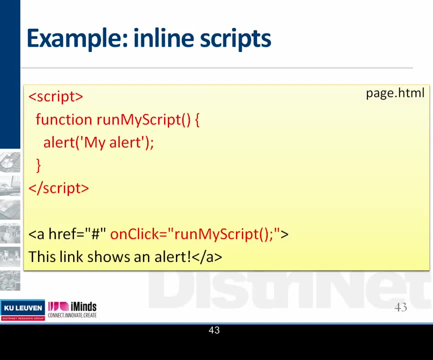 You Don't click And you Ask Time, Some JavaScript. It's Easier Than You Are Listening, Because You Don't Have Really Things That Link Your Stuff. 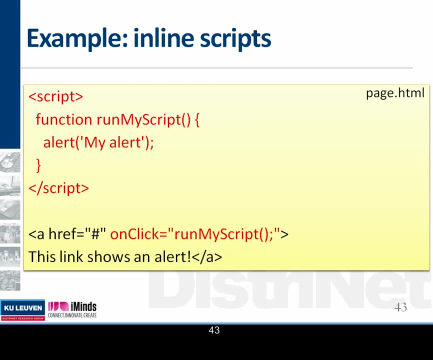 With The Corresponding Functions. That All Defined In Your External File. I Think That Might Be A Good Compromise, Because You Say Well, I Specify. 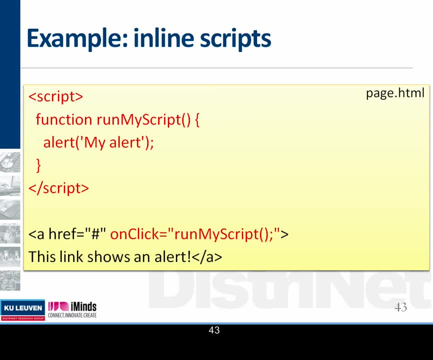 Clearly What Is Allowed To Execute On My Security. But For Now The Standard Doesn't Specify, Certainly Not The 1.0. But I Understand Your. 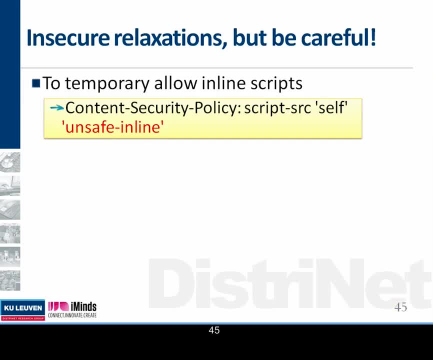 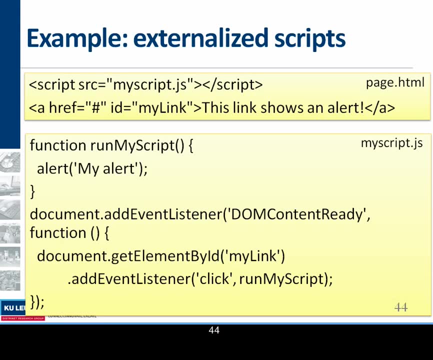 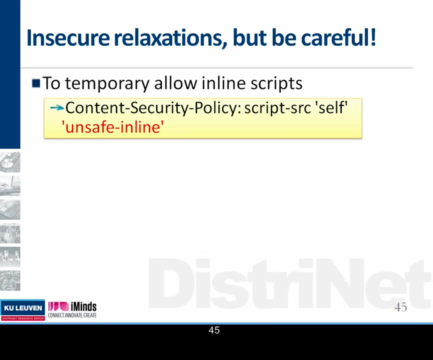 Concerns, And If I Would Be The One Deciding, I Probably Would Invest. It Doesn't Mean That You Are Allowed To Run Inline JavaScript. 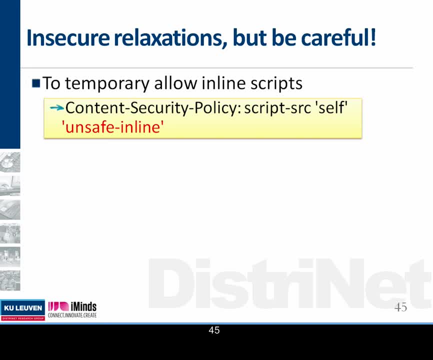 That's What Self Means. But Of Course We Have Legacy Applications. We Have Inline JavaScript. How Do We Load It To Be Inline In The 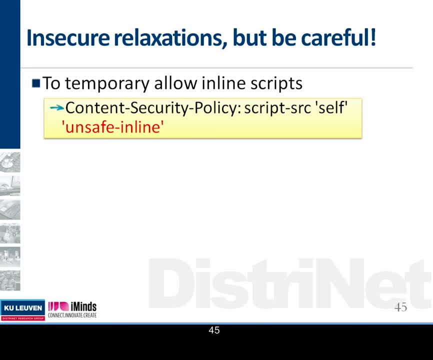 Page Self. It Will Tear Down Some Power Of CSP But Maybe In First Way To Start To Get Certain Things Being Made May Happen. 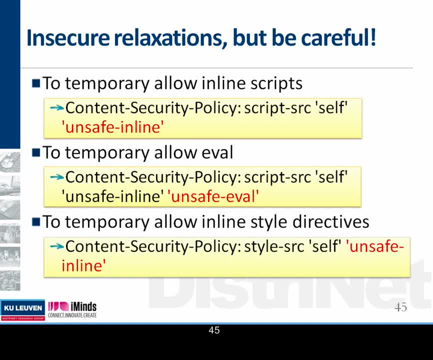 And Similarly We Can Also Say The Unsafe Inlining Of Style Sheets Is Allowed As Well. But I Really Want To Stress This Might Harm. 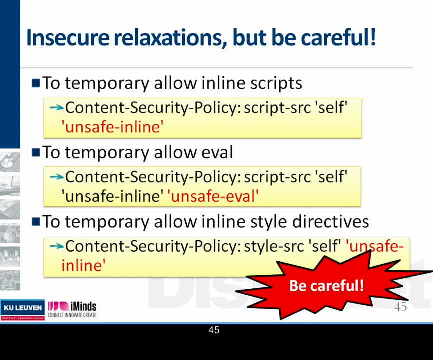 The One Of The Interesting Features With I, So Maybe, Before I Go Further On, Does Everyone Understand. Well, What's The Concept Of CSP? What? 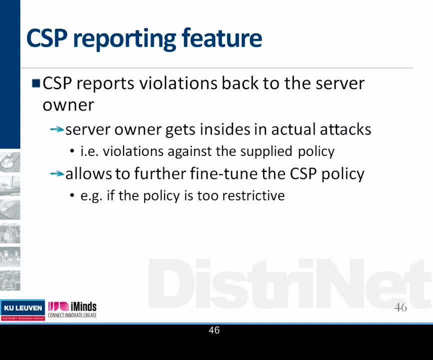 Is The Idea Of Actually Limiting That Any Violation To Your Policy Can Be Reported Back To The Server Owner. It Means That You Actually 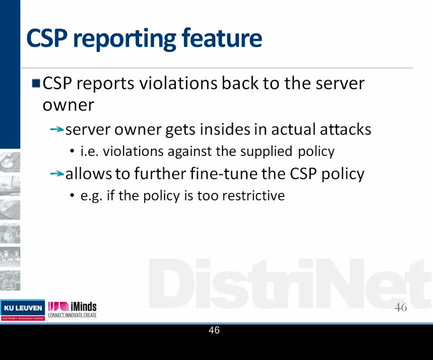 Can See Attacks Happening In Real Life On Your Application, Find In Your Policy, And We'll Discuss A Few Examples Later On, But Now You 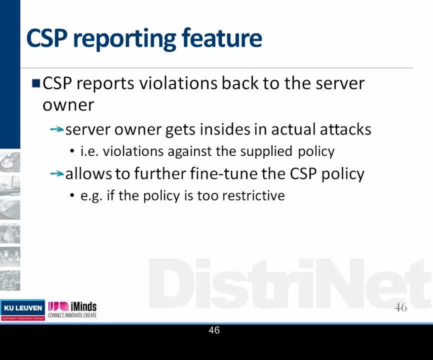 Know That Certain Pages Are Not Rendering As You Expected Because The Including Stuff- What Your I- Is A Certain URL. It Can Be Local, But 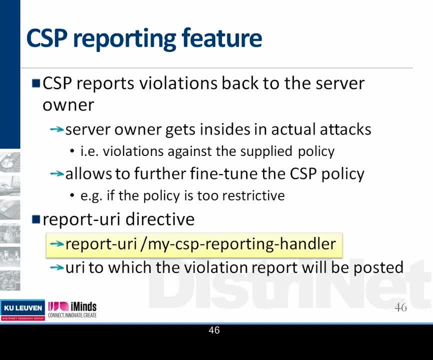 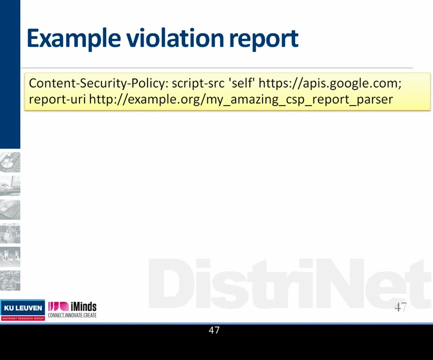 Also, After Some Discussions On The Main List, Is Also Allowed To Actually Send It To A. Let's Look To One Of The Examples Of 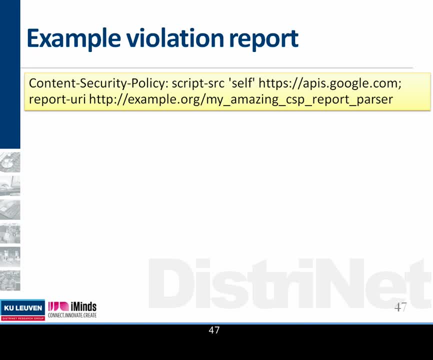 Such A Violation Report. So We Have Here Very Simple Content Security Policy, And By Now Everyone Should Be Able To All Resources, Because We 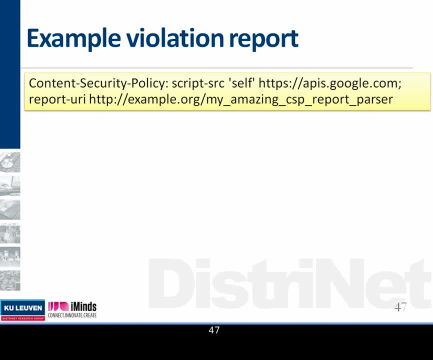 Didn't Discuss. Other Resources Are Not Disallowed By Default. If There Would Have Been A Default Source, None All Other Resources Would Have Been Blocked. 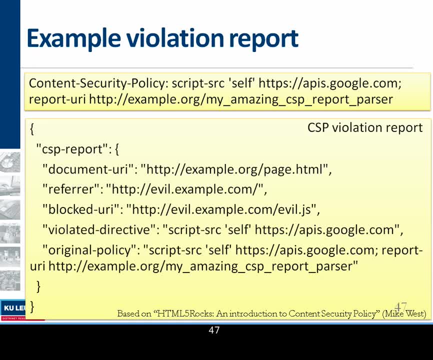 By Other Resources. So This Is A Very Simple And Very Simple, But It Is Very Simple, And It Is A Very Simple, But It Is. 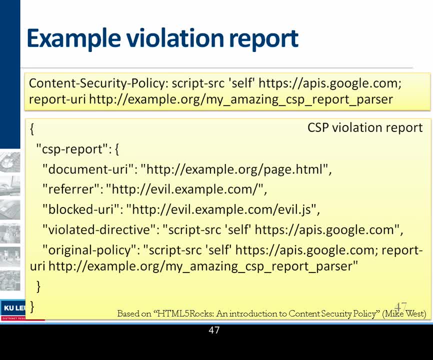 A Very Simple. This Is A Very Simple. Material Is A Very Simple, But You Have Some Information About Refer You Also Give As Part Of 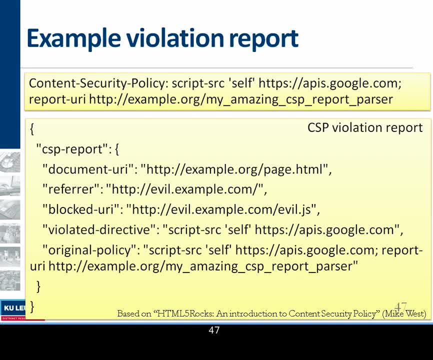 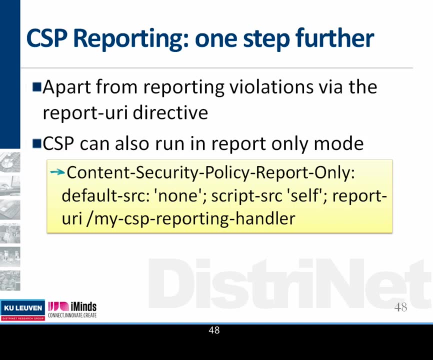 Your who And You Say. Actually, Interesting to fine-tune, interesting to see real-time attacks. It's actually even becoming one step further, even more interesting, with the reporting feature. So, apart from reporting the violations from a policy being enforced in the browser, 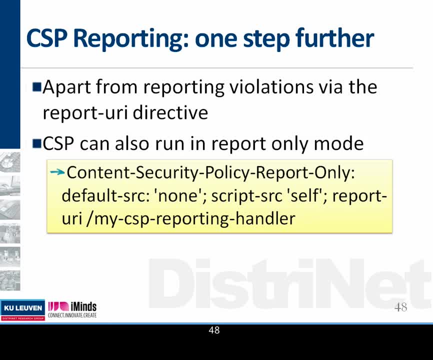 you could also run CSP in a report-only mode. What does it mean? You can actually specify the whole policy you want to enforce on your website, but you have actually a beta testing. What you do is you report violations back to your server, but you are not enforcing the policy. 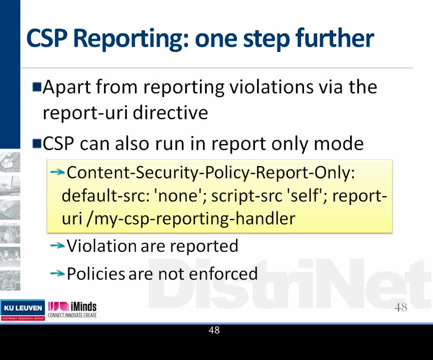 So the resources are still loaded so that the user doesn't notice anything what's happening in his browser. but at least you know for your page how well your policy is actually suited to support the policies that you want to enforce on that page. And this is the first step you do. 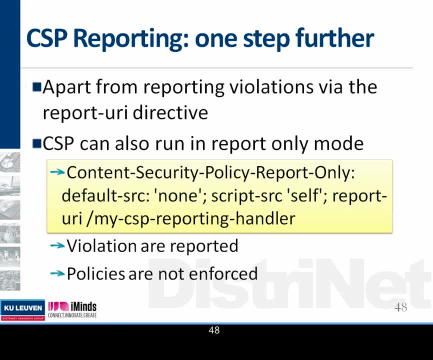 You run it in a report-only, You see how well your website behaves. what are the information, the violations coming in? false positives, false negatives. and then you can go one step further by actually enforcing it in real-time in your browser. 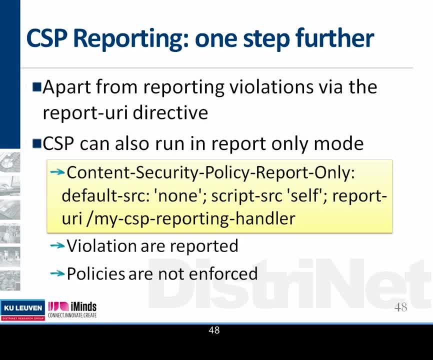 So I think the whole step of reporting and being in report-only mode is a very, very interesting thought of actually being deployed in new systems, on legacy systems, on systems in the wild, where you can actually have different steps before you're actually blocking content in the user's browser. 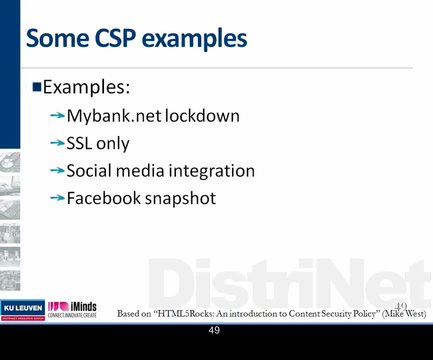 So does everyone understand those concepts and reporting concepts? Tom, Would it be possible for an attacker to report his own report? Certainly it would be possible. yes, Because it's just a normal URL you post. you could post anything, And it's something they have no means by now to actually protect. 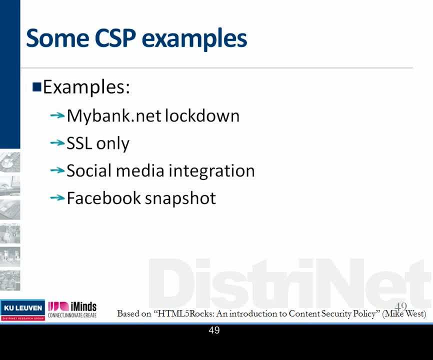 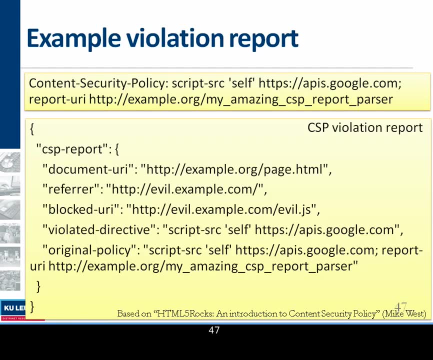 You could think of that. you're using, for instance, information in the URLs that you're having some kind of token which is actually specifying from where you're coming. You could think about a referrer. You could also say: even in the policy itself you could include that, for instance, 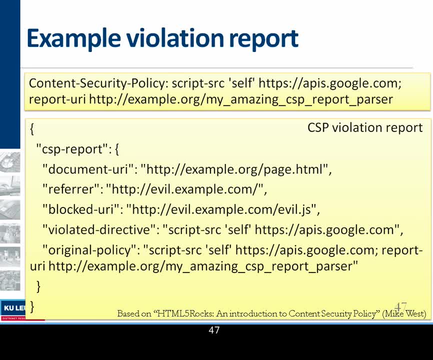 apart from these domains, you also include one subdomain which actually contains a token, to make sure that only the items you send to certain domains are being reported back. A little bit similar like cross-site request, for the tokens are all happening. 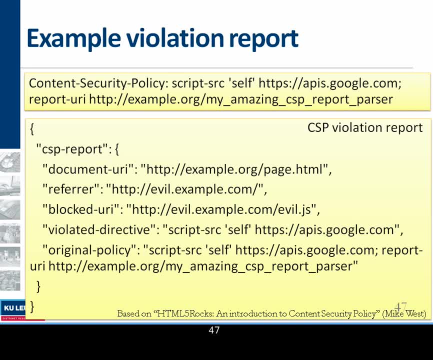 But I didn't have any thoughts on how to protect or how to. that are actually being discussed by the committees proposing CSP. But I think it's a very interesting thought because indeed what would be hell if you actually have kind of a lock on your server. 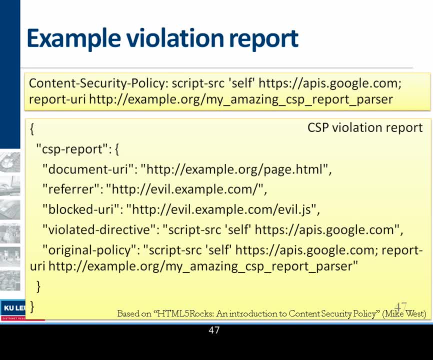 and that you can't trust the lock coming in Denial of service, Denial of service. Or you have like 20,000 things being locked and one is actually the real attack. So it's very hard to distinguish. I think you're absolutely correctly. 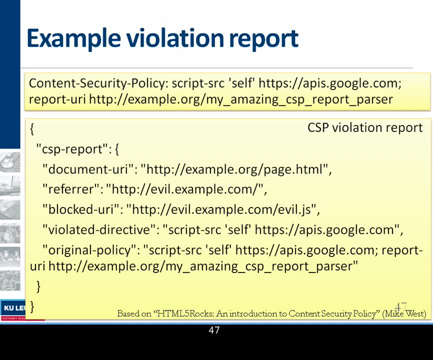 I think also the people that intended to report only in report mode mainly hadn't thought to actually do the report only mode as bootstrapping mechanism Or, if you are changing your pages or enforcing new policies, to see what's happening on the client side. 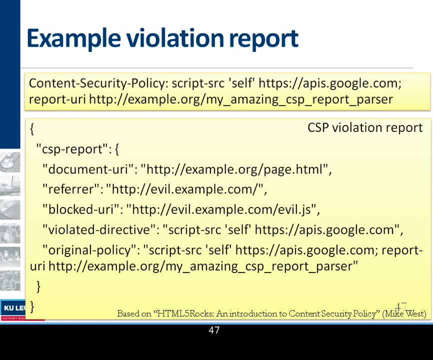 rather than real-time monitoring what's happening on the client side. But that's a very correct observation. Alec Is the content. security policy specification itself can be a possible target of an attack so that it's protected by DLS, only Because you send it as a header like okay. 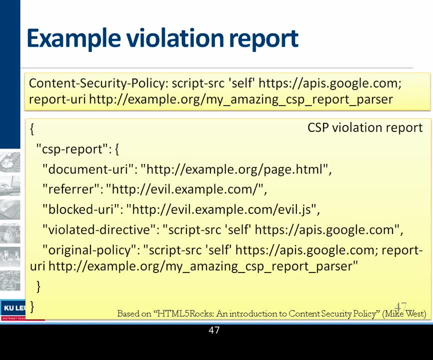 I can imagine if as an attacker, So if you're sending it over an encrypted channel, the integrity is preserved. If you send it over an encrypted channel, it's much easier to actually adapt the page itself than adapting the header. But you're true with that. 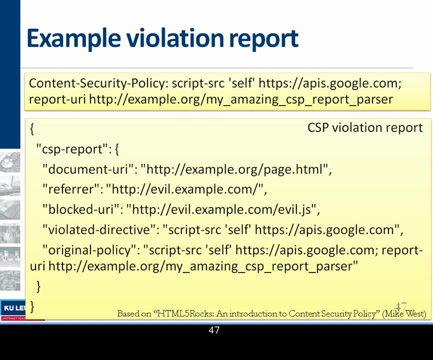 Also, I think people using CSP already took all the previous steps before they continue to CSP. Also, I don't think- and I want to really state that clearly- this shouldn't replace all the mechanisms you have in place to protect against cross-site scripting. 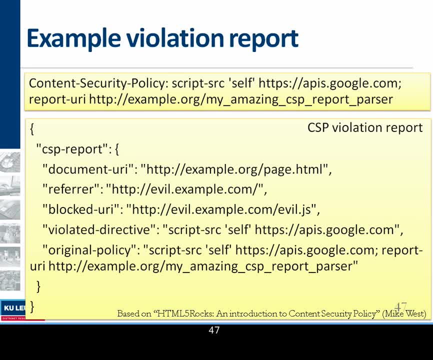 If you missed an additional layer, if you missed one thing and actually the coding guidelines in your company or external software that you are loading, you have a better way of actually being protected on the client side. That's the only thing that they want to achieve. 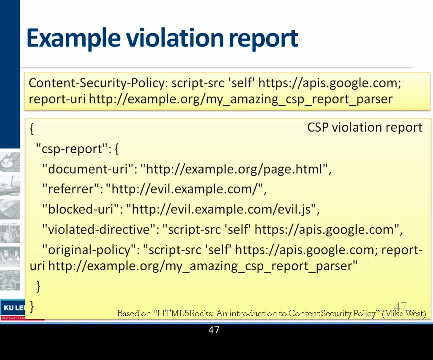 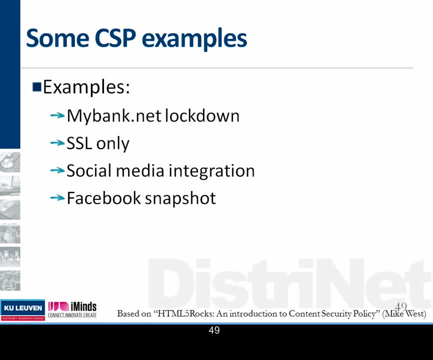 They don't want to say: you don't have to do output encoding anymore, you don't have to do any output validation anymore. That's certainly not the case. So a few examples just to get a little bit exercised in reading CSP, understanding what is the power of CSP. 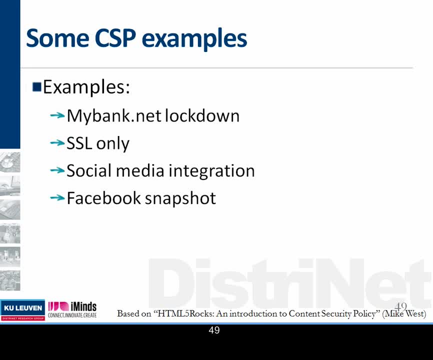 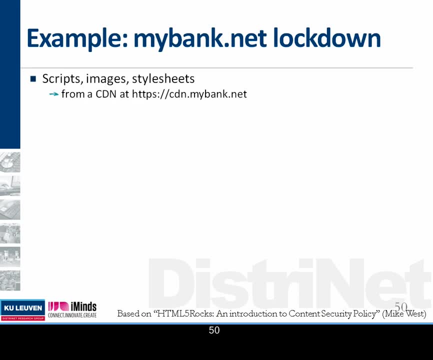 and then we'll continue to the next topic. So the first one is mybanknet. It wants to look down what resources are included in the bank. Again, those are examples based on my quest interesting report on HTML5 rocks. So one of the policies could be. 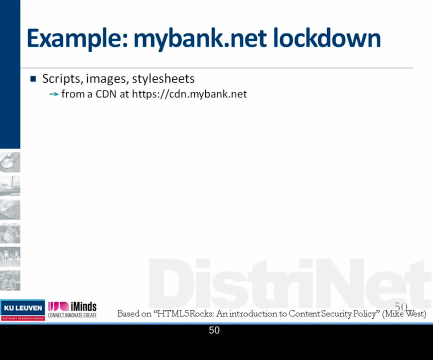 well, we want to load scripts, images and style sheets all via our content distribution network, So that CDN may actually provide us a lot of content. It's owned by us, We actually trust it, So we are able to load that. 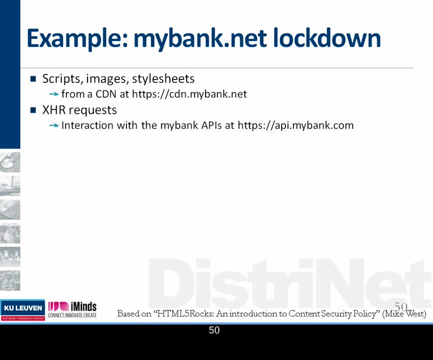 We need to make XHR requests, but we only allow it to the API that our bank is providing via apimybankcom. Third, we want to include IFrames on certain pages that might be advertisements. that might be, for instance, certain subsets of pages that we want to load in our website. 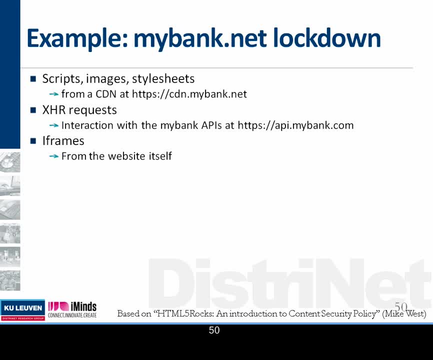 but only if they are coming from our own website. All the rest of the IFrames will be denied by default, And I think a good exercise. we don't want to have any zero days by a flash of Java. We don't allow any of those in our website. 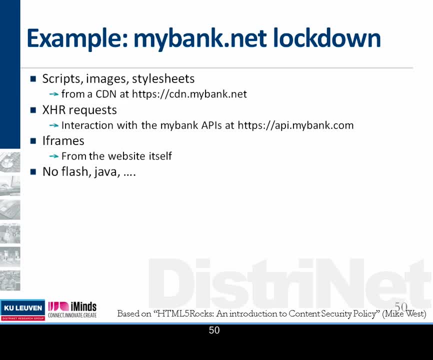 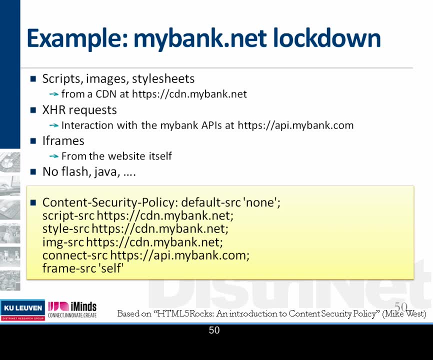 Well, if you would actually transfer that to a content security policy. so one thing I want to say. this is all one line in your header. I just broke it down in different lines with character return to make it a little bit more visible. 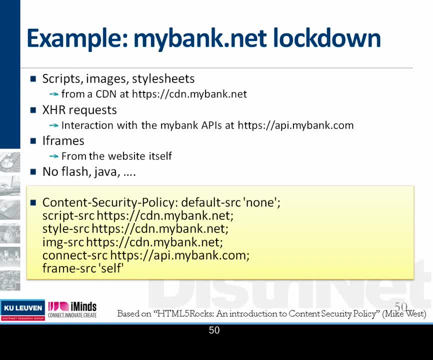 But you will see the policies are becoming bigger and bigger any time you want to add additional knowledge to your policy. The reason that I want to push it all as part of the header and not as a separate policy file is that I actually want to make sure. 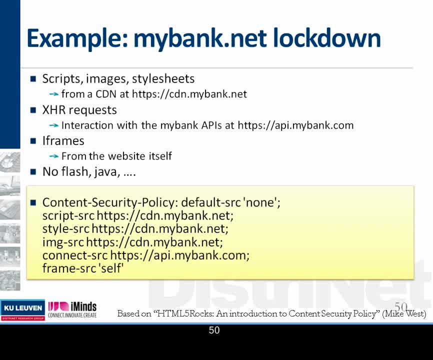 that you only need one response and you don't need to fetch additional resources before you can actually load the page. So there was a whole long debate on the mailing list: Do we want to have policies externalized of being part of response itself? But it turned out that they wanted to push the policy. 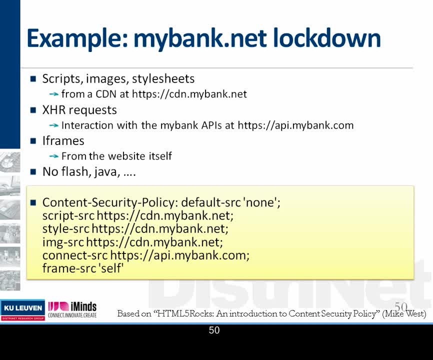 as part of response itself. So here you see the default. We don't load any content that was not specified in our policy. We load everything from our CDN in those three lines. We are allowed to exit chart to our API and frames are only allowed from ourselves. 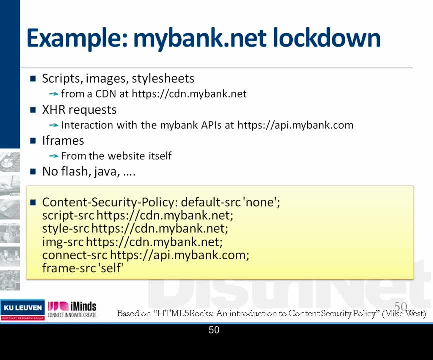 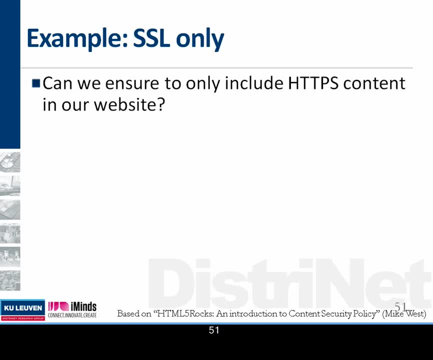 So this is the basic policy of explaining those rules on the top of the slide. The second example: Are we able to actually make sure that our website is only including HTTPS content And for people having an SSL certificate, for instance with extended validation? 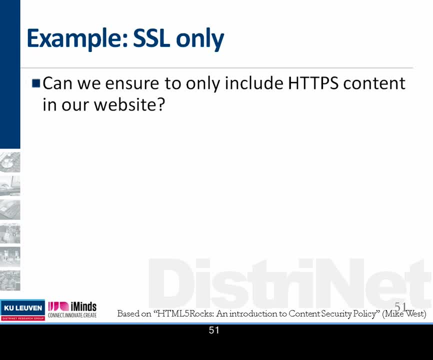 it's important to actually make sure that they load only HTTPS resources, because that actually will otherwise reflect in the way an SSL statement is reflected in the header bar of your browser. It will say: you're loading unprotected content. There might be a good reason to say: 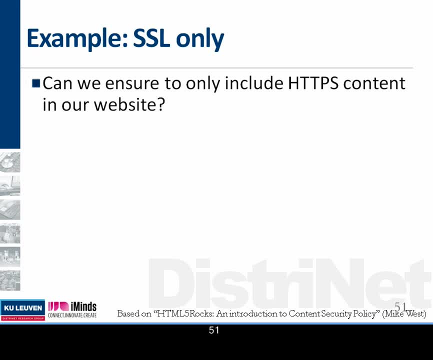 I only load HTTPS content, Certainly scripts. you want to load JavaScript only over HTTPS and we can discuss that later on during the break. How would that policy look like? Well, you say the default policy is the default source. only the scheme HTTPS can be used. 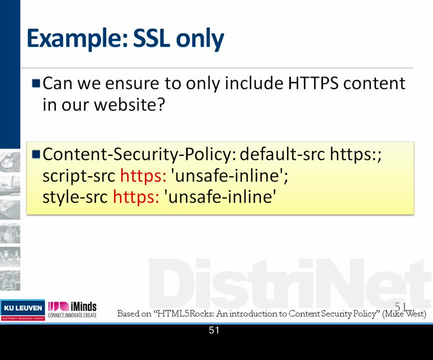 In case that you are overriding directives, the whole default is forgotten, So you need to replace it in any relaxation with unsafe inline for styles and scripts as well. So if you forget this, the scripts and the styles would still be allowed over HTTP. 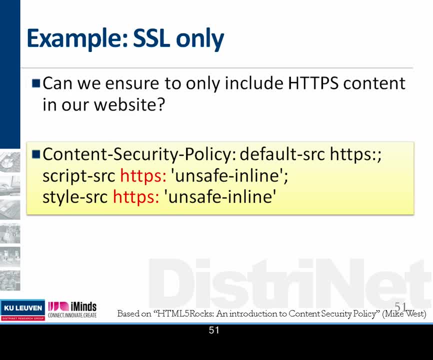 So this could be a policy that you can deploy At this moment without adapting any of your website. styles are still inline, scripts are still allowed inline, but by default you get the opportunity that you only use HTTPS in all your resources. If you had one additional line saying: 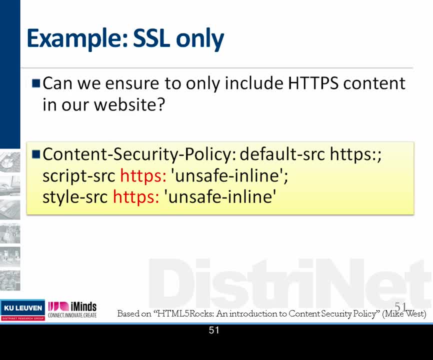 I don't want to use Flash or Java. you might have already a very good default protection mechanism on your website without changing any code. This could still allow an attacker to move third party resources as well as the other HTTPS resources. Yes, indeed. 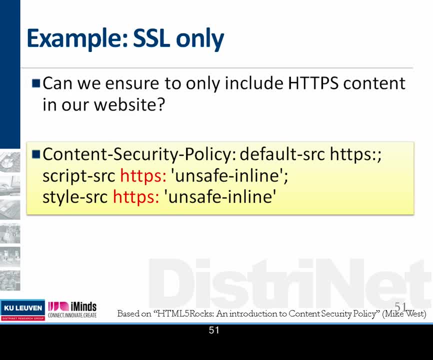 But it would make sure that, for instance, your JavaScript itself will never go unprotected over the wire. So this is only an example, certainly not the final step of protecting your website, but it gives you just a few ideas of how you can use the CSP mode. 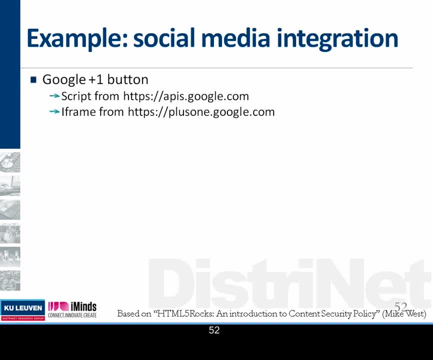 And then we have a lot of websites having social media integration. Google Plus has scripts and iframes, Facebook has an iframe, Twitter has a script and an iframe. So if you want that all to be included in your website, well, you need to add quite some content. 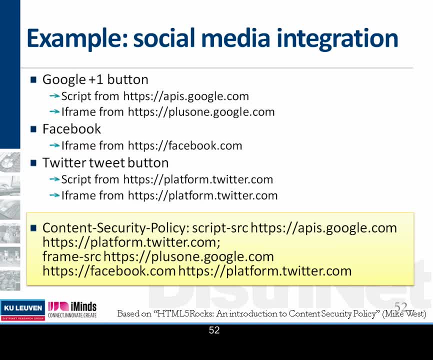 to your content security policy. I think by now everyone understands how this mechanism of CSP works. I won't go deeper in detail on explaining the policy, Just to give you a flavor. Facebook is not adopting CSP yet on all their pages, but in the crowds that we did, 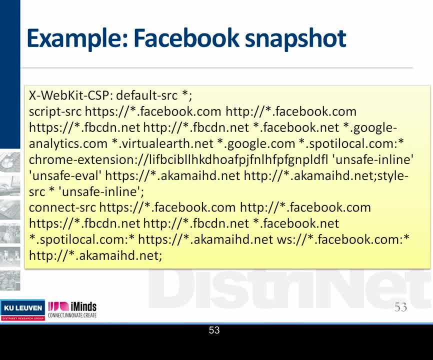 we found one response of Facebook coming back with a CSP header. so they're actually experimenting with CSP And this was already the whole policy that was sent with one page of Facebook And you see it's growing quite fast. if you need content for multiple pages, 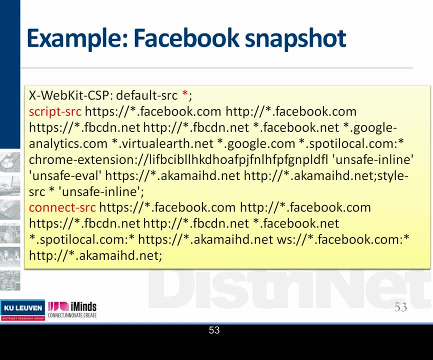 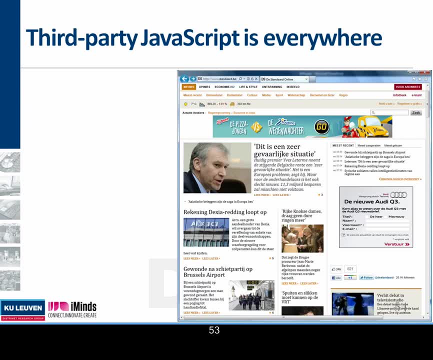 Interesting. so they're discussing which scripts are allowed to be loaded and to which websites they are allowed to connect with XHR. Maybe also interesting to show on this slide is you see here Chrome extension. So it means that for Chrome they're also allowing Skype. 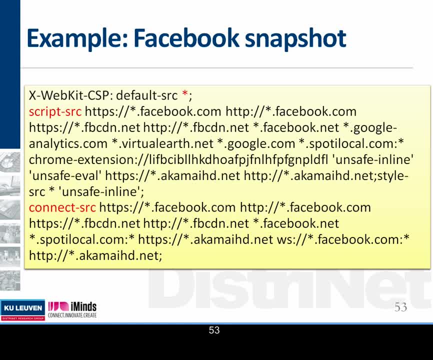 to load additional resources on their page because this is a Skype extension. This has been discussed as well in the CSP community. The next version of the implementation in the browsers should allow any extension to adapt to your page, because a lot of extensions, even extensions that protect your website- 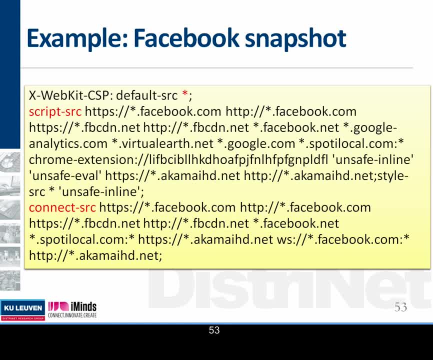 need to adapt your page or inline some script in the page. So in the future this line should not be necessary to protect your website. So the default source has to receive: So at the top, doesn't that sort of defeat I mean? doesn't that say like? 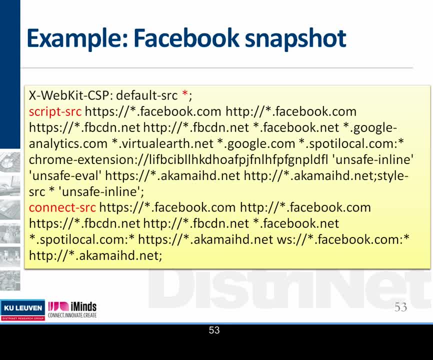 for anything. I'm not specifying anything. Yeah, well, if they would leave out the first line, it would be the same. Okay, so it happens, But they're explicitly saying it. I also think it's the first experiment. typically, what Gmail and Facebook? 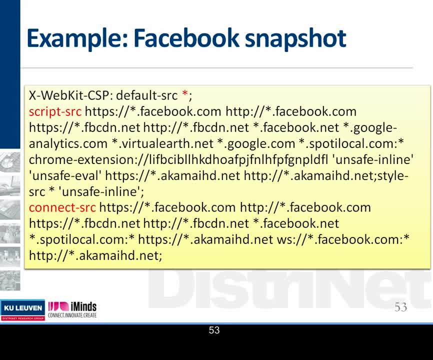 and others are doing is actually trying certain things out on a very specific subset of their users to see how they are reacting, And I think I might have removed the report URI, so probably they're also seeing what that gives up as reports and the violations. 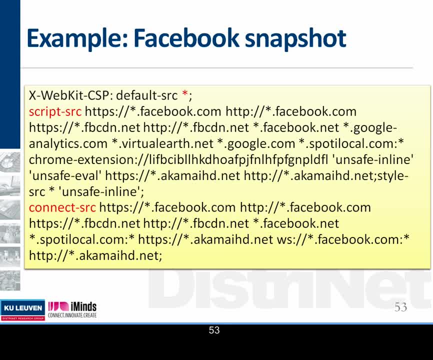 just to give an idea of is it feasible or not feasible. But we were just surprised by seeing this, because any other page that we were visiting with Facebook we didn't see any CSP header anymore, So it was really a snapshot If we didn't have captured that. 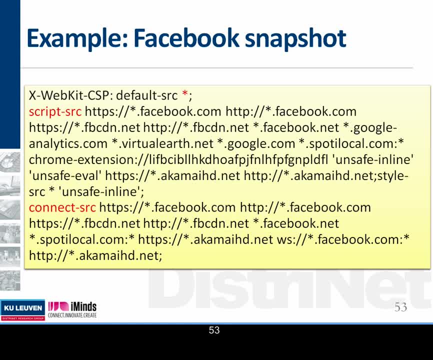 we wouldn't even have known that they were testing with CSP. So, if I understand correctly, the CSP is most effective. if you sort of view it as a wide testing approach, you really specify only the things and then you better send that default source to the model. 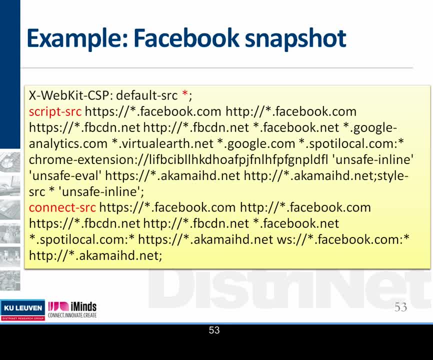 Yeah, indeed, That's sort of then. it's really wide Indeed And it's debatable. if you, for instance, for video and audio, you could question yourself: do I really want to say which audio video is allowed or not allowed? 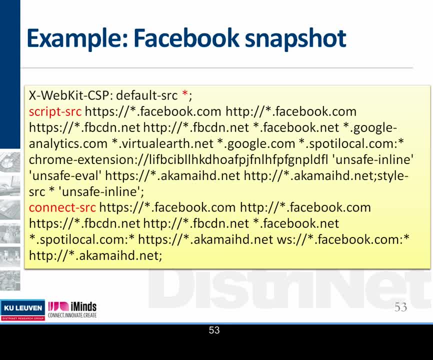 What I also see in my experience in the use of CSP- and I will discuss it later on, also with who is actually adopting it. people are also using those attributes to protect their IP, So YouTube wants to have that you visit the YouTube pages to visit their content. 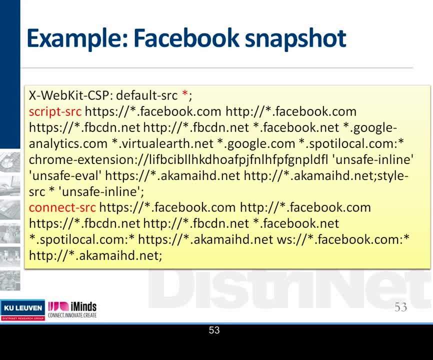 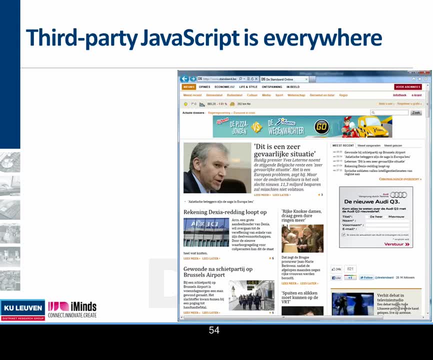 and that no one else is actually visiting it, And also- that is something that is interesting to see- that also there there might be some interesting thoughts as well. Well, just a little side note. we all know that JavaScript is everywhere. If you're looking to one website, 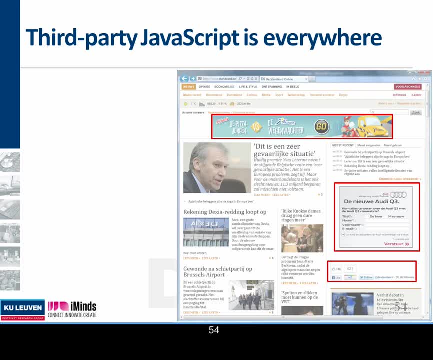 of the standard local newspaper. you see already some visible things like advertisements, social media being included, But behind the scenes there's a lot of JavaScript doing tracking, analytics and a lot more. There's a whole bunch of JavaScript you can include on your website. 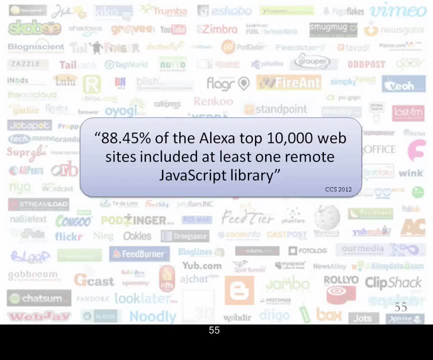 And we saw in an experiment that more than 80% of the top 10,000 websites are using at least one remote source and mostly they're actually using Google Analytics. But if you want to know anything more about that, just visit the talk of. 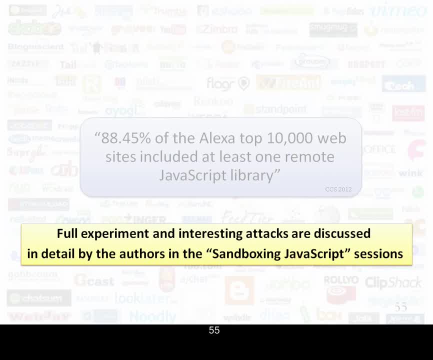 of Steven and Nick the last of this evening. They're actually having a whole experiment actually visiting websites seeing which resources they are including, and they also have some kind of neat attacks to attack the way people are including JavaScript. So I don't want to say 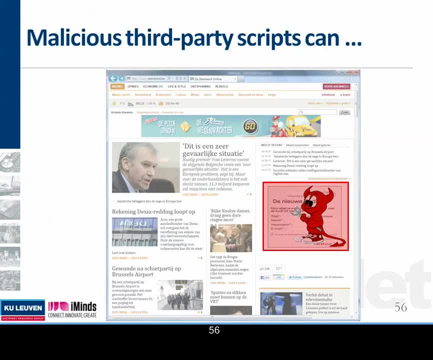 anything more than that. Just if you have control over one of those JavaScripts, you just own the website. I think everyone by now knows that this is the case, So let's focus on the state of practice. There are two browsers supporting currently CSP. 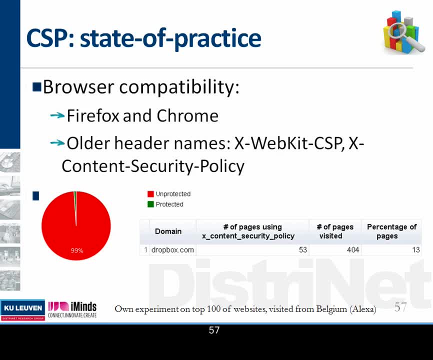 namely Firefox and Chrome. We also see in the wild that we had previously all the header names like the X, which means experimental, for WebKit prefix. for the Chrome version. We also have X content security policy, But I think one two weeks ago. 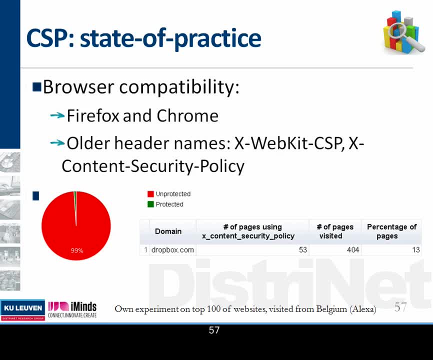 we had the final draft, So now we can just call the header content security policy And also the browsers are adapted to take the header name content security policy rather than being prefixed. When we did an experiment on the top 100 websites, we only found: 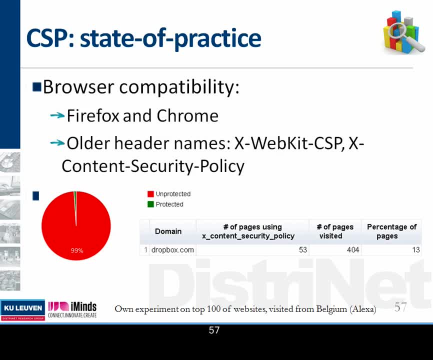 that Dropbox was sending out CSP headers. So you see, it's still an early stage of what we're doing, So we have a lot of information that we want to share with you today, So let's get started. So the first thing we want to do, 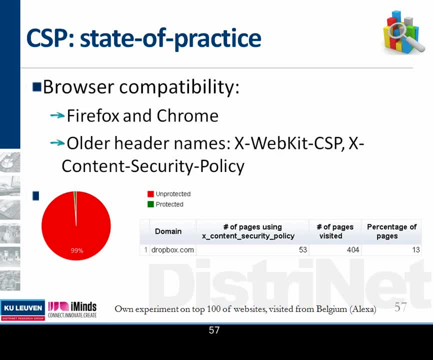 is. we want to show a little bit of adaptation. People will be using it probably much more in the next few years, But for now, only a handful of websites are issuing the CSP And I think, similarly to Facebook, probably a lot of websites. 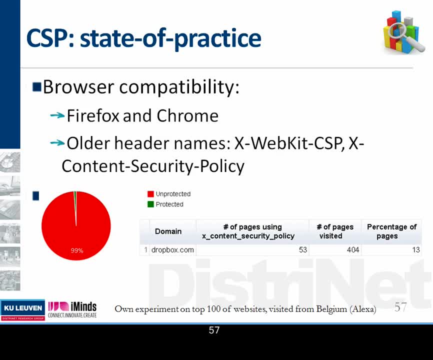 are very temporarily trying out certain things on CSP and disabling it again just to make sure that they are not breaking anything on their website. So a very small recap on what we saw about script injection, what we saw about the text. We had the HTTP only flag. 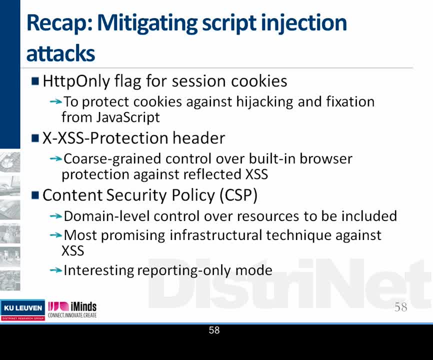 We had default behavior names in the browser against reflected cross-site scripting And a very interesting way of actually using the content security policy as an additional line of defense. The last topic I want to discuss in this session is how to use framing, And I will actually. 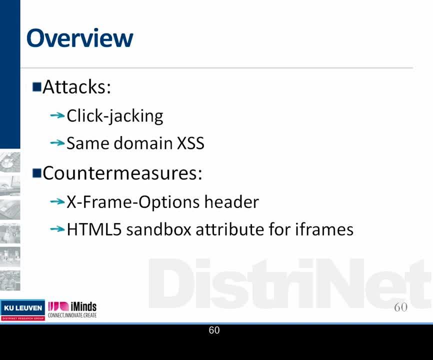 visit two things: Click-jacking- And I will only focus in a very small bit on click-jacking because it was already mentioned by Jim twice, But I also will discuss same domain cross-site scripting, So the name is not correct. What I mean with this? 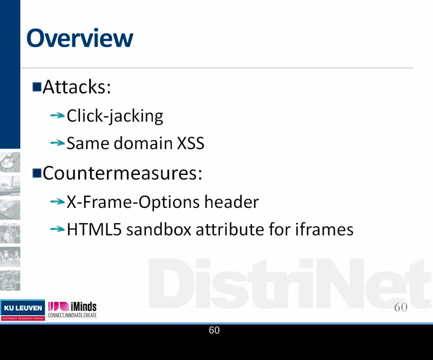 is actually? we saw a good way of actually using frames to actually remote. content can be isolated in its own security context. But what happens if the security context is the same, because you are actually loading unsaved resources from your own domain And we focus on the HTML5? 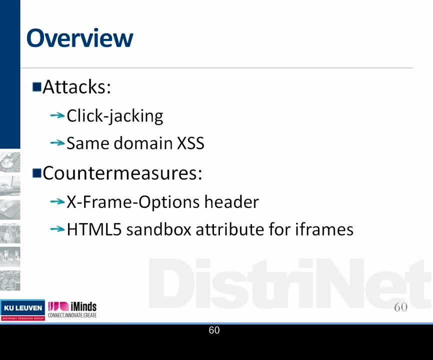 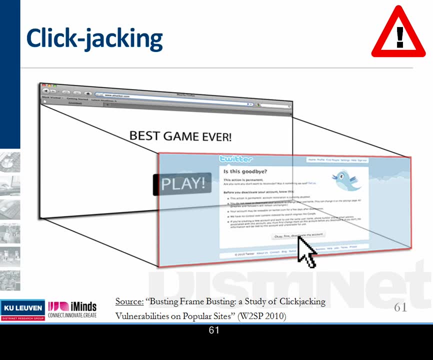 sandbox attribute to actually protect against that. So click-jacking: you just show an additional frame in front of the other one. The user doesn't see it because it's transparent and you are actually clicking on the wrong thing. Any kind of random measure that was specified? 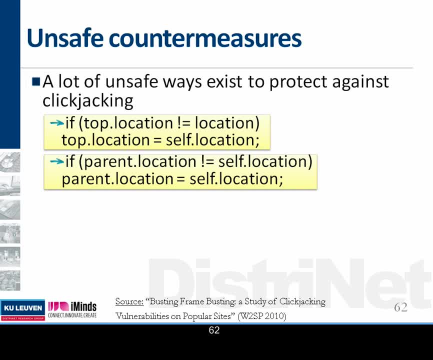 previously written in JavaScript or using all kinds of neat techniques as a developer, to defeat that by actually navigating your own page and things like that. Well, they are broken. You can disable them by disabling scripts and using sandboxing techniques. You have the frame. 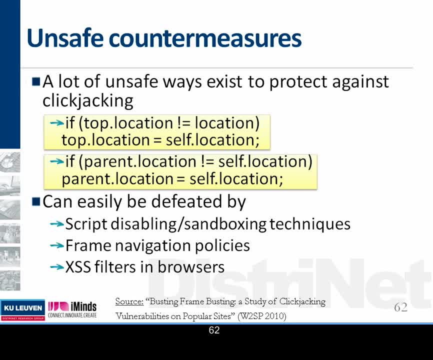 navigation policies actually making sure that you can't navigate the top level domain. You have certain techniques, even being protected by the cross-site scripting filters- that protecting against reflected cross-site scripting. So it's very hard to actually see what is the way to protect. 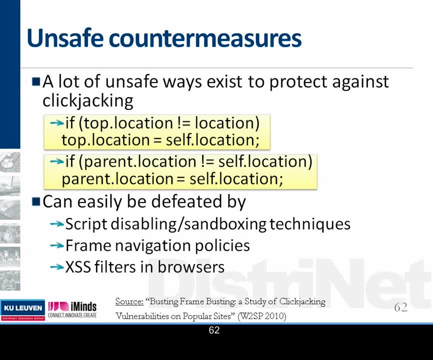 And there's an interesting paper Busting, Frame Busting, studying the whole experiment of click-jacking and also all the different ways that are actually broken to protect against click-jacking. But the good news is it does extreme options. Again, it's a. 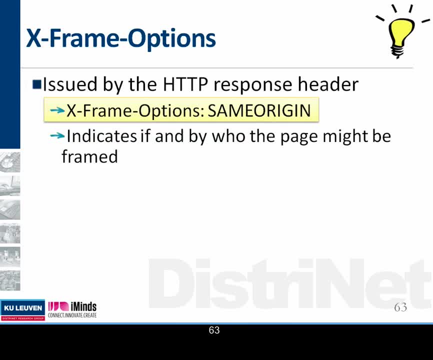 response header With extreme options. you say which domains are allowed to frame your content and you have three options to say. well, you could say deny, nobody can frame me. You could say same origin, which means you can frame but others can't, And you also have: 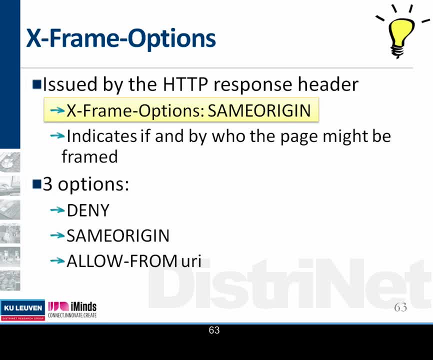 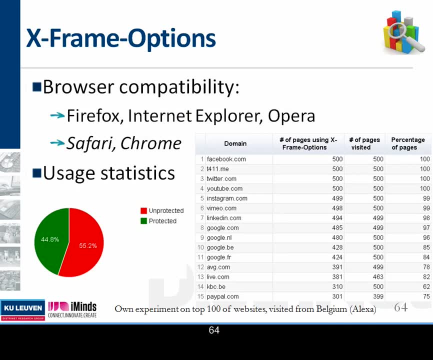 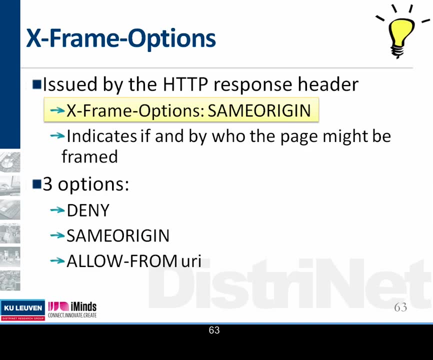 the allow from where you can specify certain origins are allowed to frame me. The browser compatibility is Firefox, Internet Explorer and Opera all support this feature fully. Safari and Chrome do not allow, do not support the allow from, but they do support the deny and the same origin. 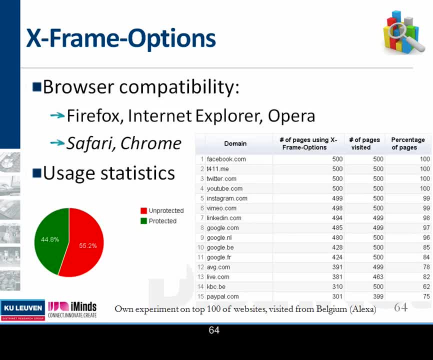 Again, almost half of the websites are protecting themselves and I think it's a very, very good countermeasure. if you have a stateful operation on your server, just issue an additional header naming saying you only allow it from the same origin to be framed. 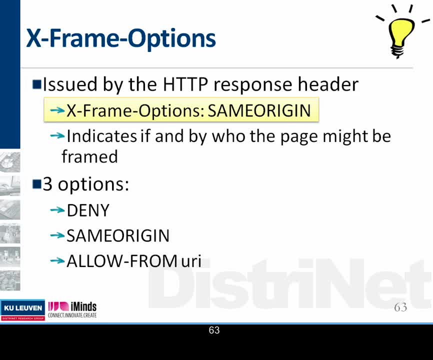 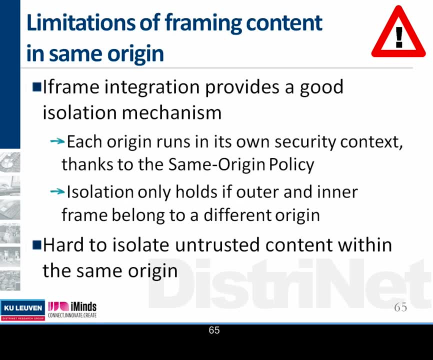 All certain websites don't need to be framed and you're protected against click checking. Very short. there's much more information in the paper. I don't have the time to go any deeper on that. What is important here is what's important in framing. 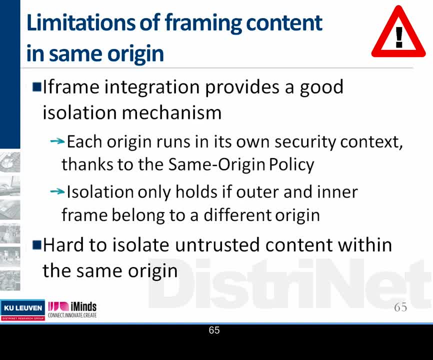 in general, we saw frames being used as separation contexts, but if you have content from the same execution coming, they're running in the same execution context. so even if you're using an iframe for them, they just will be able to walk to the other DOM chains even remove. 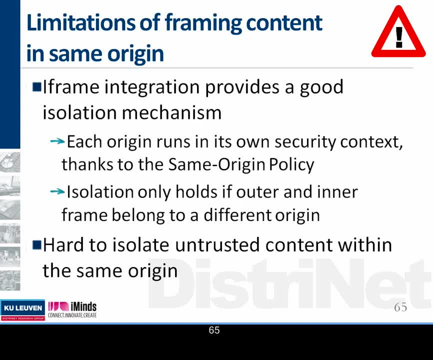 the iframe, so they actually have full power over the whole website. So it's very hard to isolate content coming from the same origin, And for that we have the HTML5 sandbox attribute. What does this HTML5 sandbox attribute do? Well, it actually. 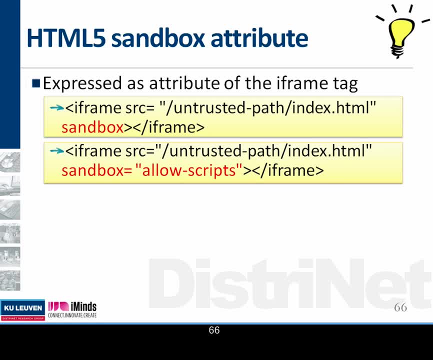 enables the same origin policy even for content from the same page. You can use it without any value. then it's the default behavior. but you have also ways of actually making it more fine grained. So the level of protection you have very coarse grain sandboxing. 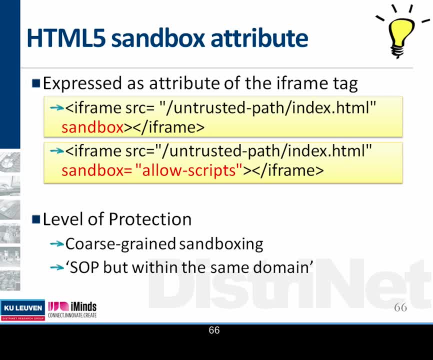 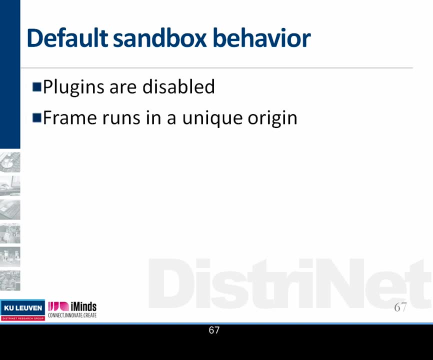 you have the same origin policy within the same domain, and this is the basic set of sandboxing JavaScript. much more advanced ways of sandboxing JavaScript are discussed in the talk of Steven and Nick this evening. So let's talk about the sandbox attribute in HTML5.. 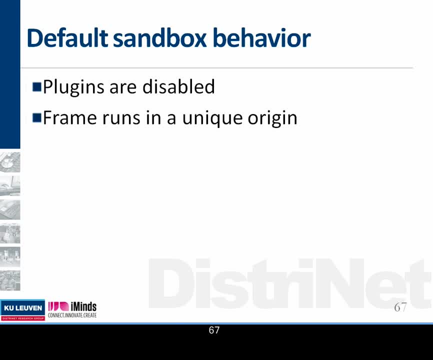 Well, you disable plugins and you run frames in a unique origin, which means for each of the frames having the sandbox attribute, they will generate a unique origin. and actually, that unique origin has its own execution context, which means if you have content from the same domain and you have three, 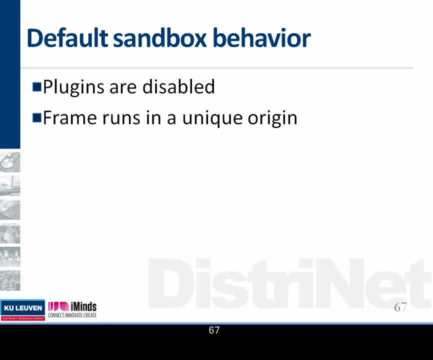 different iframes with the sandbox attribute, you will have three unique origins running in your browser. they are not able to see any of the origin and they are not able to communicate unless you specify it, so they are really bound to something that you uniquely create and cannot be. 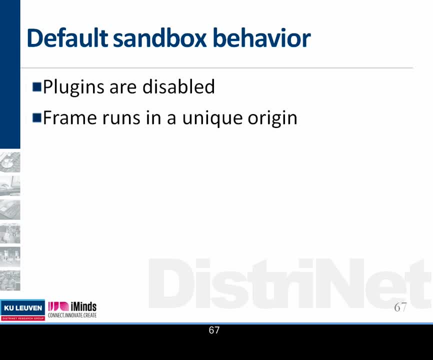 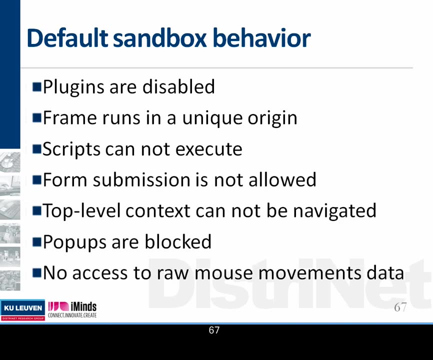 duplicated. Also. by default, scripts are disallowed to execute in such a sandbox. you are not allowed to submit any form or push any form button. you can't navigate top level context and popups are blocked. you don't have access to raw mouse movements, so you actually 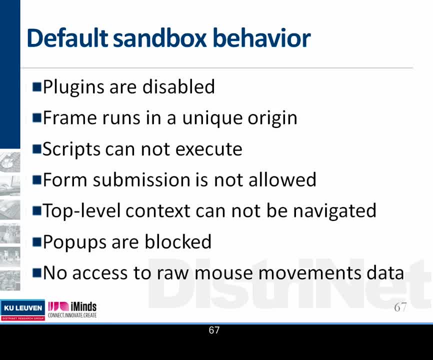 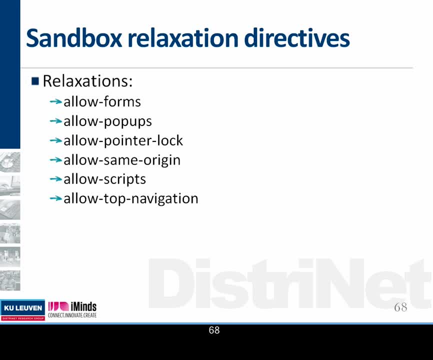 have a very confined environment. you can't do much with a sandbox environment. of course you could do some relaxations to say, well, I allow scripts to be running, I allow to have popups, for instance, so you can actually fine tune what the sandbox environment can do. 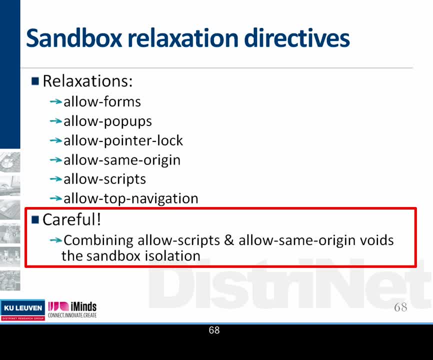 but please be careful: if you combine some of the relaxations you could just actually mitigate the whole technique of sandboxing. so for instance, if you combine allow scripts and allow it to run in the same origin, well you can just walk up the DOM and just remove. 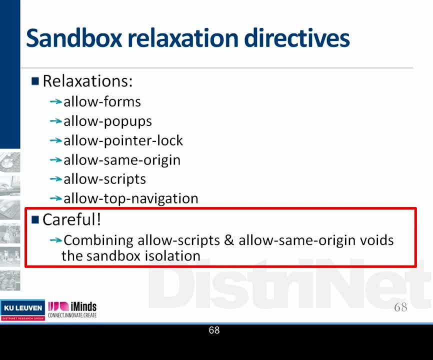 the sandbox without needing additional content. so be very careful. if you do the relaxations, I think the default relaxation should be allow scripts, because you allow scripts to run, but they're running in a different context, so they can't harm your website. I think that's the 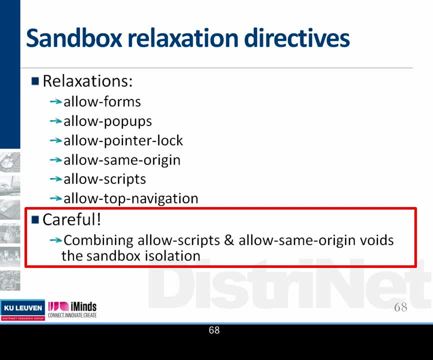 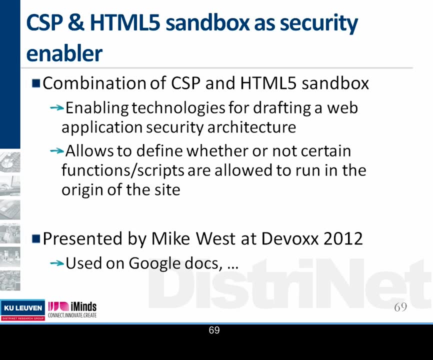 main idea of sandboxing, and one thing you can't relax is plugins. any sandbox environment doesn't run any plugins. I think that's also quite good behavior by default. so- and I think I'm closing to the end of the presentation- so I really want to show you. 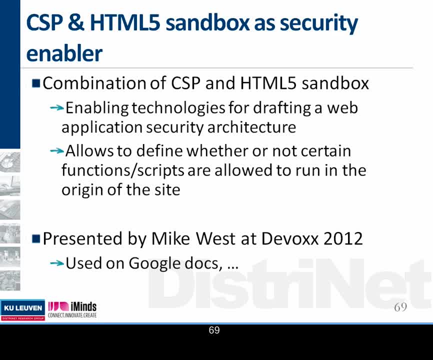 an additional step, namely how some of the technologies I discussed today are just the basic building blocks, because what's interesting in developing applications is actually using those building blocks to have a more secure security architecture for your web application, and this is why, for instance, CSP and HTML5. 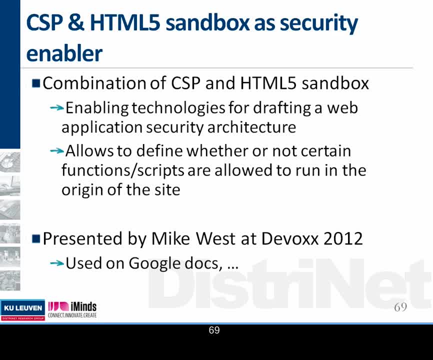 combined can play a very interesting role. so one of those architectures presented by Mike West at DevOps 2012- and they're actually using this technology to confine certain unsafe functionality in their repositories, like Google Docs, where they want to allow scripts to be executed, but they want 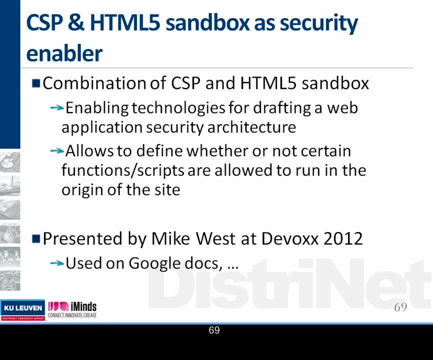 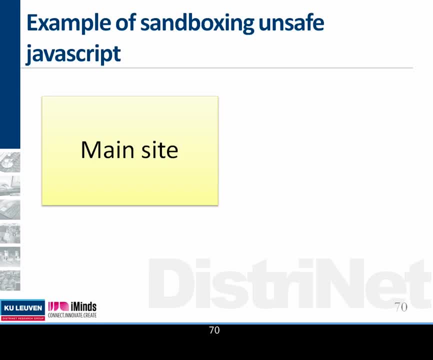 to confine it via those architectures. so how does such a security architecture look like? well, you start with your main site. your main site wants to protect itself of untrusted executions. what does the security architecture do? the first tip is you create a sandbox JavaScript execution environment. 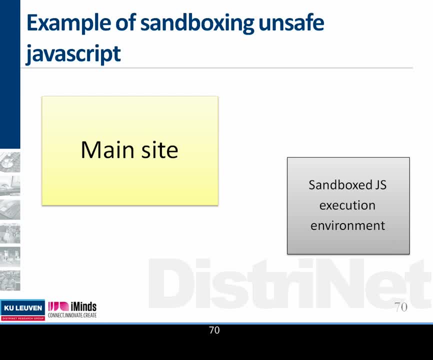 and then you actually have web messaging allowing communication between the main site and the sandbox environment in a very controlled way. and how does the security policy actually apply on those topics? well, the first site, the main site: you protect it with CSP, which means you're not allowed. 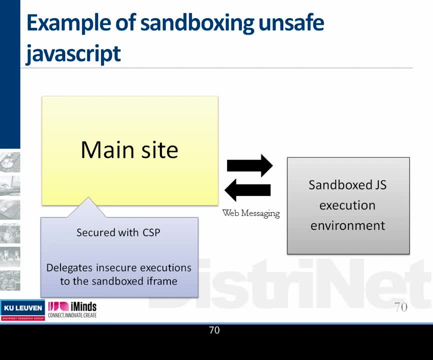 to run any inline JavaScript on that website part on the main site. you're not allowed to run any inline JavaScript on the main site. so what is not allowed is to delegate all the executions towards the sandbox environment. the sandbox doesn't have any restriction in executing JavaScript. 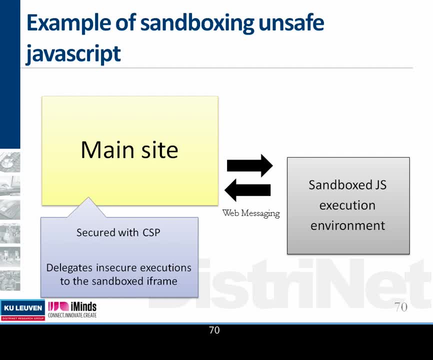 but it doesn't have any access to the data being protected in your main site. it doesn't have access to your cookies, to your local storage. it can't issue as being from that domain. it's really in a confined environment, sandbox environment. you can create a quite interesting. 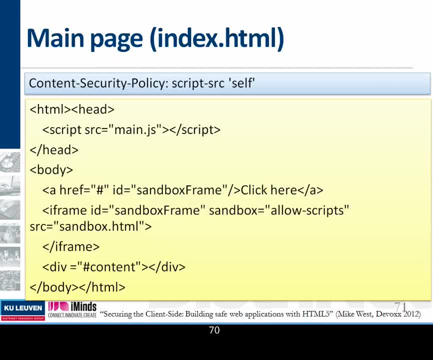 security architecture. so let's look how this would be actually implemented, and then you will understand what I mean by interesting features. you have your main website, which is actually loading a JavaScript mainjs. we're having an iframe. being the sandboxed frame, it's allowed to run scripts. 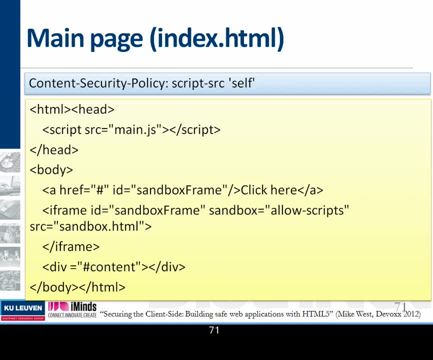 and it's sandboxed, so it means it runs in a unique origin, but still you can run JavaScript. it's not safe. we know it's from third parties. it might do any harm, but the resulting string, we would like to display it to the end user. so we would like. 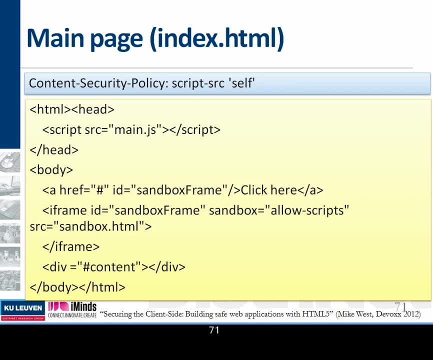 to display some content in this element on our web page. so this is the main setup. we want to execute something. we contrast what's going on. it could read our cookies, send out whatever it wants, but we want to execute it without having impact on our own security. 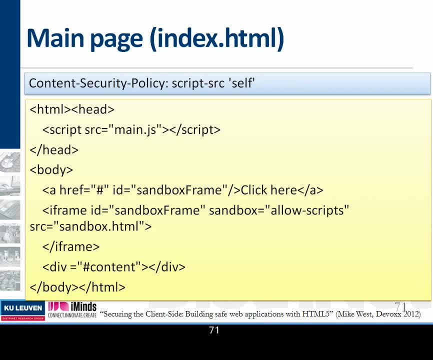 but then the results should be displayed on our website and the same thing is actually enabled because we have the content security policy. we can load mainjs, but we can't inline any JavaScript later on in the process. so the mainjs: what does it do? well, on clicking. 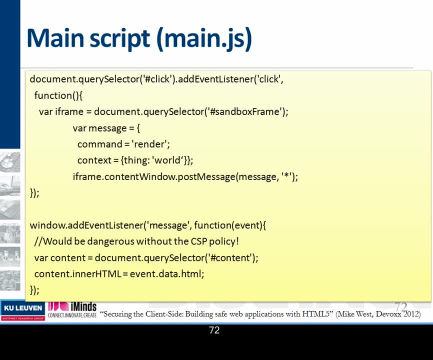 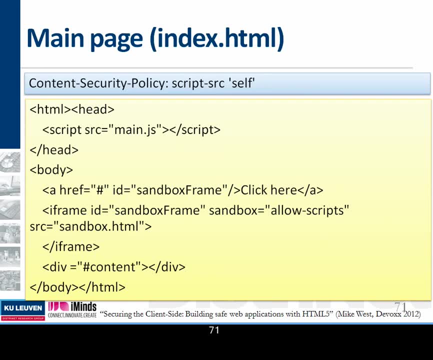 the event handler on the previous page. so we have an event handler that we want to bind to to the click here button. so but this shouldn't be sandboxed frame, this should be click. then what we do is actually we click and then we say: once you have a click. 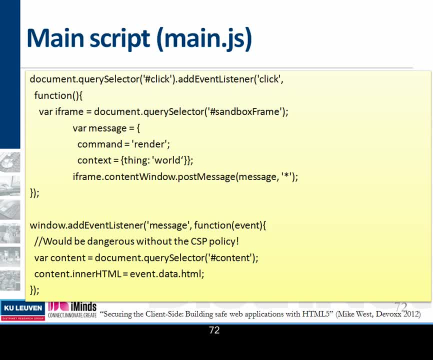 we contact the sandboxed frame and we will actually do web messaging via post message and sending the command we want to execute in the unsafe execution environment and the data that might have to be used, that might have used. so we provide him some content, only a subset. 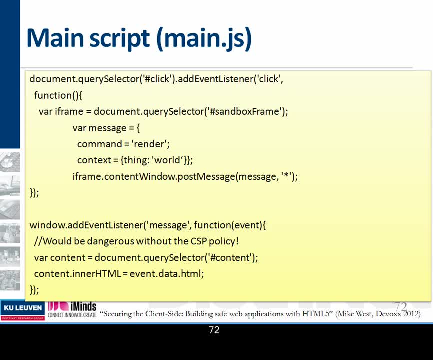 of the data that we have on our website, but that data can go to the untrusted environment. it does some execution on that and gives us a little bit of information about the content that we want to execute and then we actually, from that insecure frame we just take. 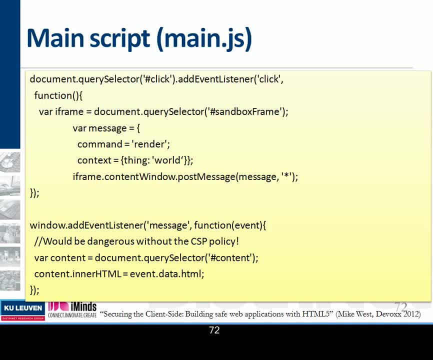 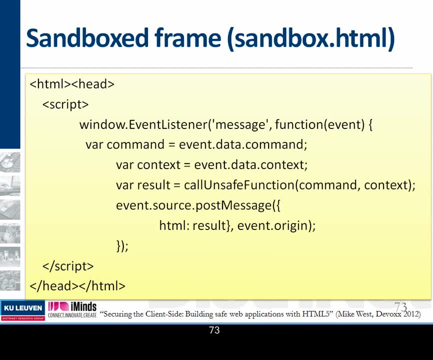 the content element on your page and push that html to that, so all the results coming back from the content will actually be inserted on our page. and then we have the sandboxed frame itself. it can run all the executions once, so it gets an event handler, that string. 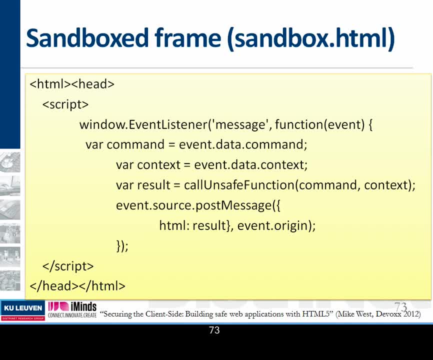 that we are pushing to the main site, because the csp policy says no inline script. we only will render the attack users, we only will render the pure html on our main website. so it's a basic idea. I don't think it's the different security architecture. 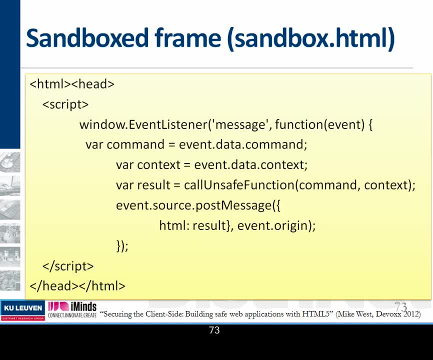 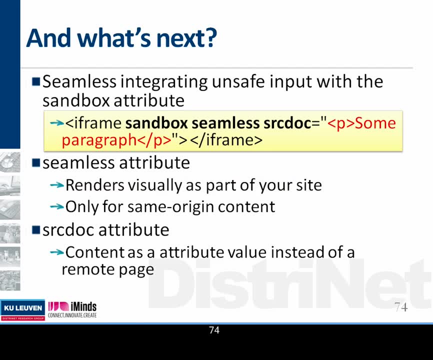 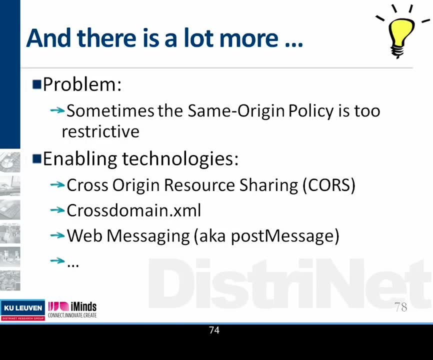 we want to go for, but it shows that the building box themselves can be combined in a very interesting way. and again, Steve will discuss much more about sandboxing later on and I think it's important to go to the conclusion. so maybe one interesting statistic. we did an experiment. 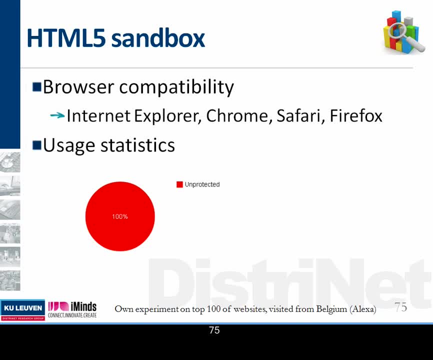 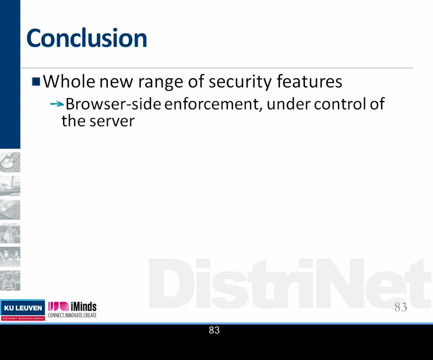 how many websites use sandbox in the top 100, none of them are using the sandbox attributes, although four of the browsers are actually implementing the sandbox in their behavior. okay, so wrap up the conclusion we saw in this presentation. the first thing we wanted to do is go. 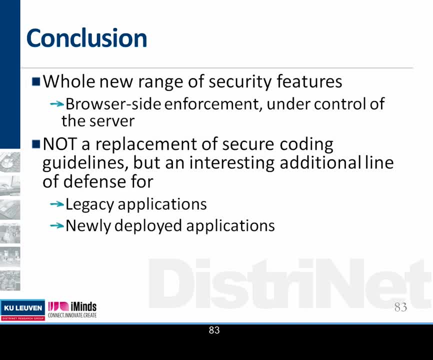 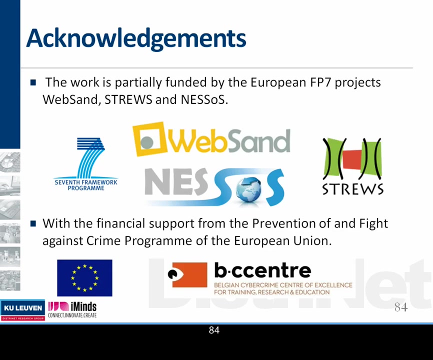 to the main site and we will go to the top 100 and see if we can use the sandbox in the main site and we will use the And with that information I would like to thank some of our sponsors in Project Context and I have also a full list of references if you want to read more, also seeing some 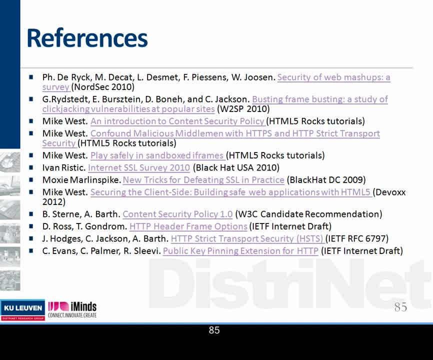 of the presentations going a little bit deeper on one of those topics And that's the end. If you have any questions, please feel free to ask No questions anymore. I think version 1.0 is standardized, but they're continuing version 1.1,, 1.2, and so on. 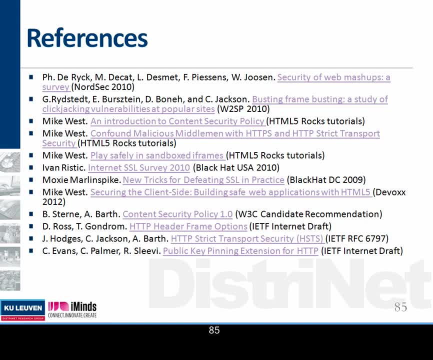 So it's a very active community. It's mainly driven by Adam Bart, which is actually pushing it very hard to get it implemented, Also because he's one of the Chrome developers- anything being discussed almost the next day and next week it's actually having a proof of concept in the Chrome version. 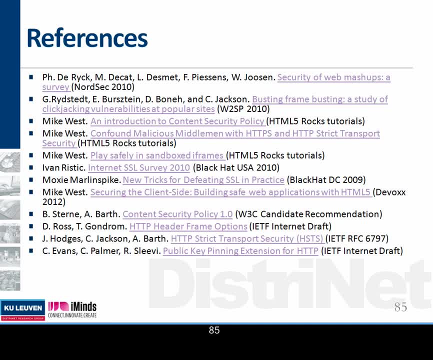 So it's really having a lot of interaction, a lot of traction there as well in the community, You know, is there something like a code user interface for defining the CSP policies? Not yet, I'm not aware of any. I saw some research actually trying to extract your CSP policy from your website itself. 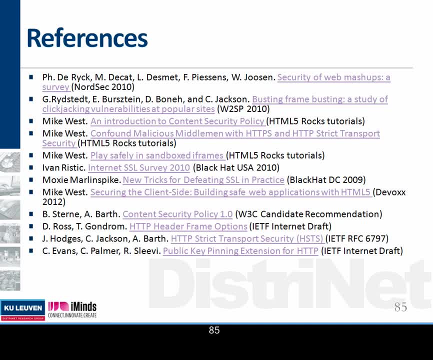 So it's actually scanning your whole code base and saying what would be a good policy. Also some of the refactoring to externalize JavaScript. But, to be honest, most papers I read on that topic only the first initial step. It would probably not be practical on your larger websites. 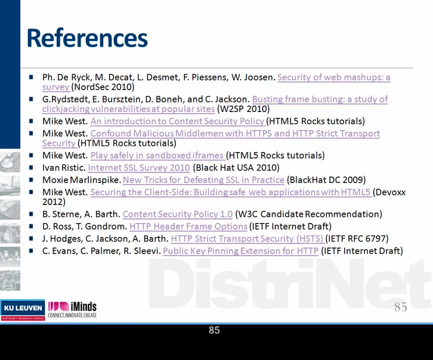 But I think there are much more to come. once that information is there, You know what are the benefits- People will jump on that. There's certainly a benefit there. I see a good benefit in actually providing the whole infrastructure of handling the reports and actually filtering out which are interesting violations. 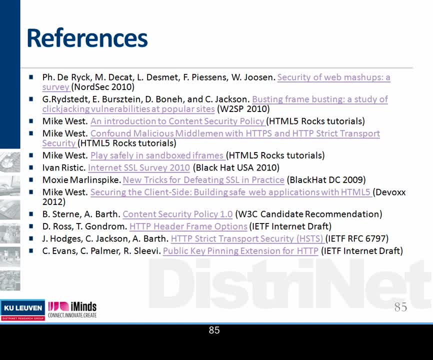 Also, there is a whole community or possibility to add new technologies in place. I guess the first thing would be also the web framework. Yeah, Indeed. So, for instance, one of the things there is, if you have multi-tier languages, like Google Web Toolkit or all those, if you're actually having it already in a meta language, that 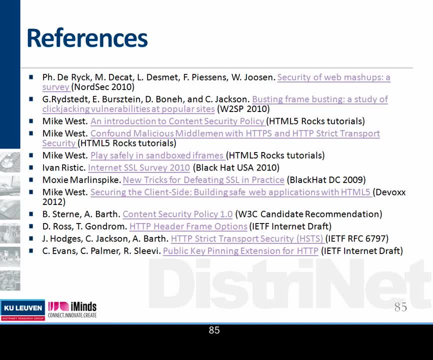 you say I want to include an external resource, then it would be very easy that that page is also compiling to what's saying. well, I also will issue a CSP header. So there might be some advantages, depending on your framework on the level of abstraction. 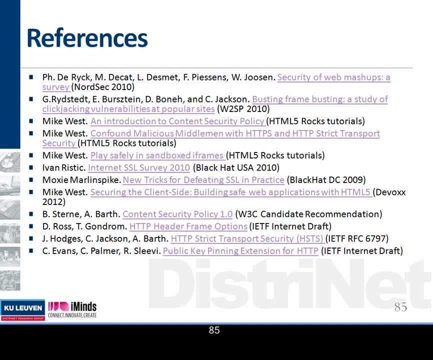 you have there. Yeah, To actually extract that information For people writing the code manually in a PHP, I think it's cumbersome to actually achieve this level of protection. But I think also there we will see a new trend in actually how you're programming your websites. 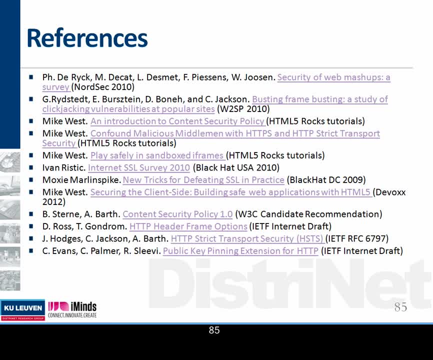